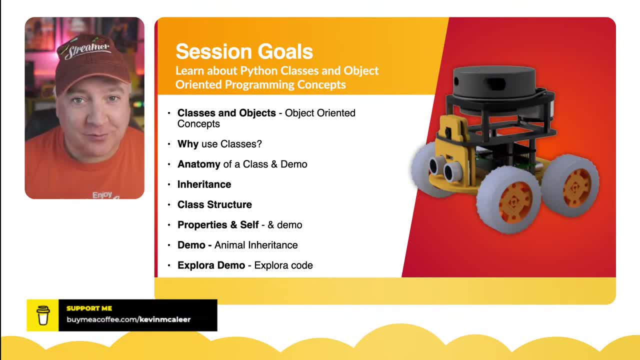 Python, object oriented programming, and we'll. we'll go through quite a few of those things today. So many cool things to show you as well. So we're gonna go over classes and objects and the concepts behind them, why we would use classes, Anatomy of a class, more we'll get into some code. It's gonna be quite quite a lot code today. 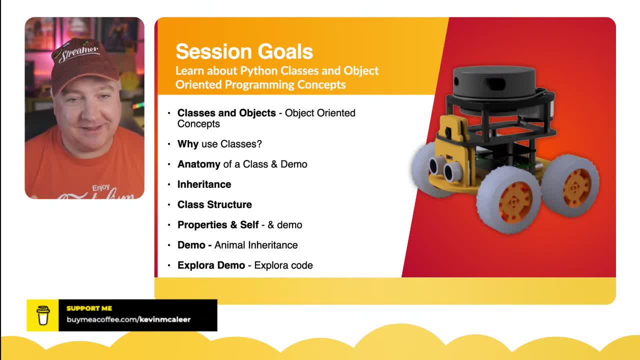 We're gonna be looking at inheritance. We're going to be out, and that's not to do with money, That's to do with how things get inherited by classes. We're going to be looking at class structure. We're gonna be looking at Properties and something called self. It sounds very. 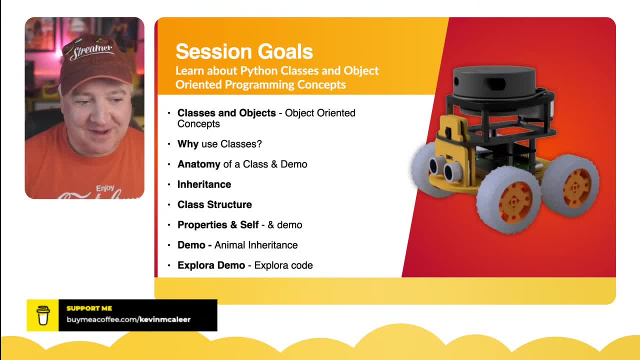 Psychological, but I have more demos on that. I'm gonna have a demo about animal inheritance and I can model it in our code, and also the Explorer, Which is the little robot I have Just behind me over here with one that's on screen there, Cool. so let me know if the audio is coming in a bit strong there. I can see it's peaking a little bit yellow. 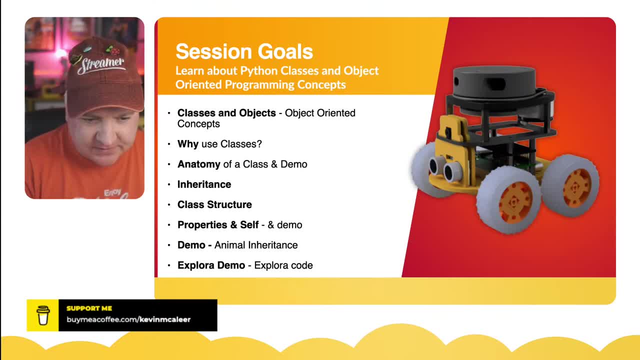 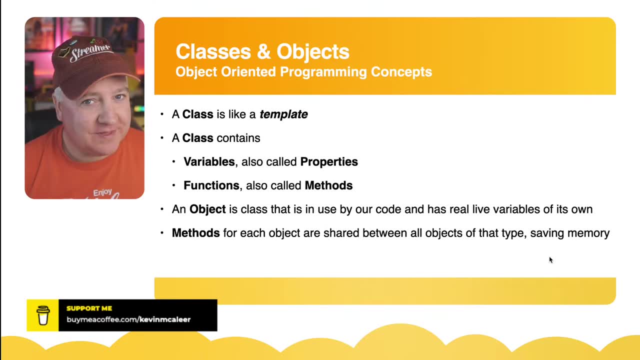 It's gonna make sure it sounds good for you. Okay, so let's go over to my next slide. So yes, classes and objects. So we're gonna go through what these are all about. So a class is a bit like a template. a class contains variables- They're called properties. when we're working with object oriented, 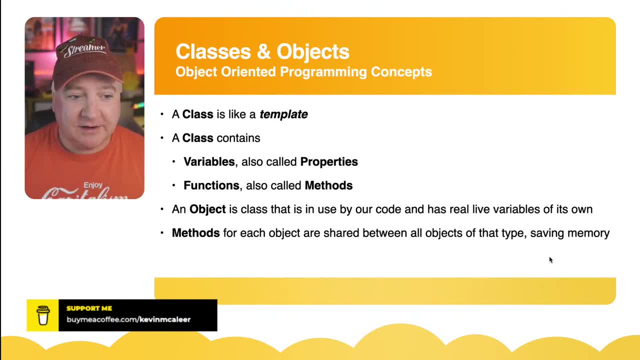 concepts and Functions which we've created before, and they're called methods when it comes to object oriented programming. So an object is a class that's used by our code and has real live variables of its own. So an object is a class that's being used. 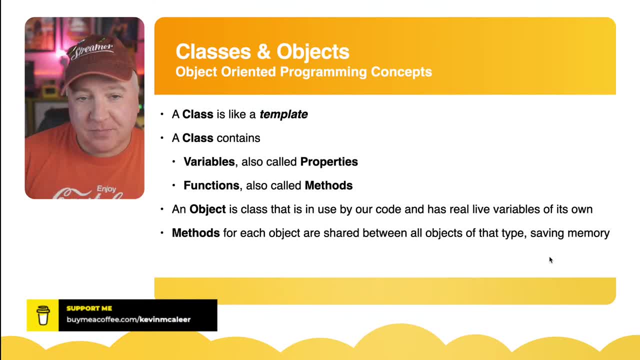 It's being executed and the methods for each of the objects are actually shared between all the objects of the same type, Which saves on memory, so it's really efficient on memory. You don't have to have like two lots of it. if you've got two lots of code using the same thing, it manages all that, for is pretty clever. 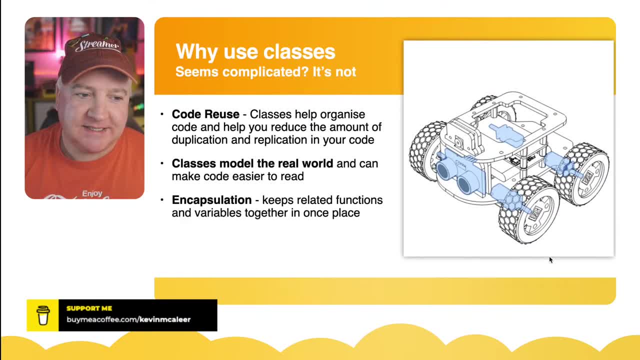 And why would we want to use classes? It seems quite a complicated thing when you first see it. you think that maybe I'll just carry on doing things. I've always done them. It's not really complicated, It's just new concept if you've not used it before- and it really helps with code reuse. 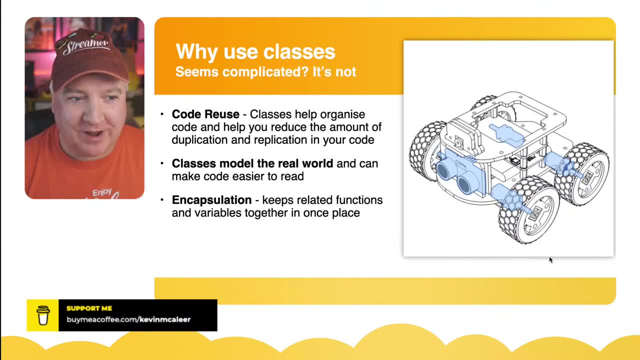 So you'll see this and hopefully what the penny will drop and it will click, why you want to start doing this yourself. So a class is how be organized, code together So it can reduce the amount of duplication, replication, in your code and it can help you model real-world things. 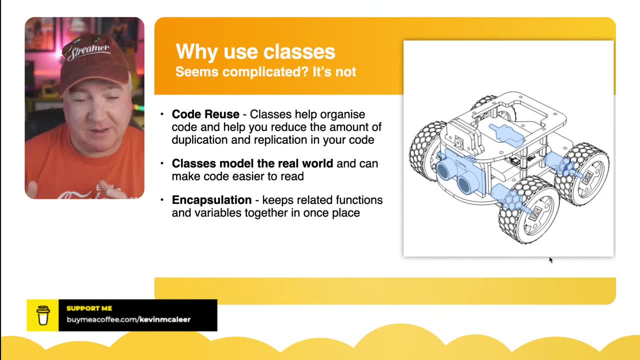 this is one of the reasons that object-oriented programming came about. people wanted to really model objects, physical things or thing concepts that make much more sense together rather than apart, so you can keep your code together. it can make your code a lot easier to read as well, and 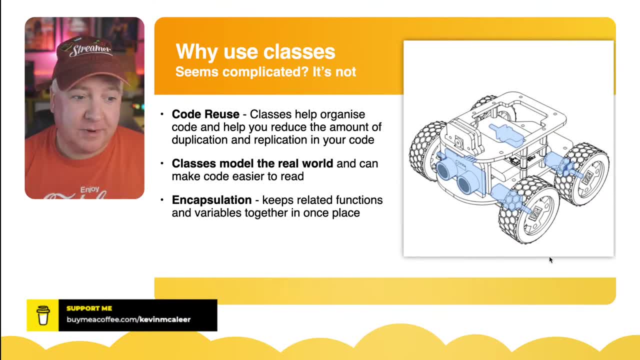 uncluttered, and one of the concepts of object-oriented programming is called encapsulation. so this is all about bringing together related functions and variables in one place. so if we want to model, for example, a motor, anything to do with the motor, speed, the direction, all the 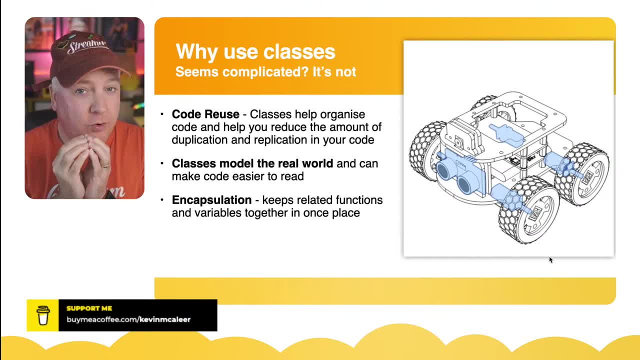 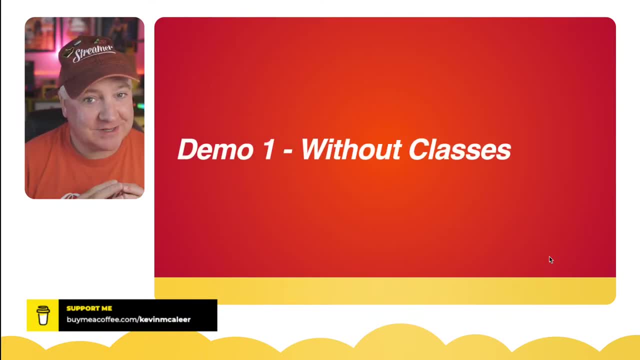 functions for making it go forward and backward and stop in. they can be all together in one object, one, one class. so we're going to have a first demo about classes. we're going to have a look at what it looks like without classes so we can start from a base point. so i'm just going to get 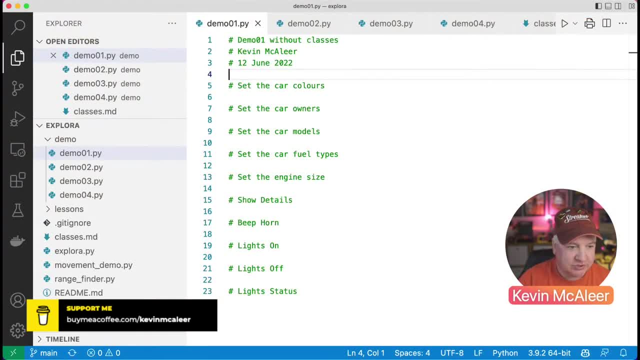 over to my um, my uh, visual studio and i've got here, without classes, i've got a bit of a template we can start from. so we're going to model cars in this particular one, um, so what we're going to do is we're going to create a couple of variables. so the first one, 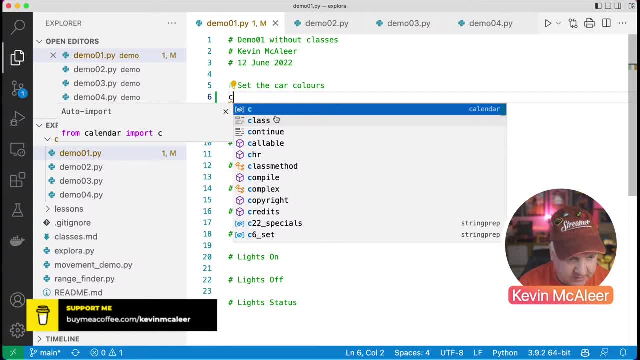 let's get my microphone just about there. hopefully that's still all good. just need to get my hands underneath my microphone. so it's a just a bit of a juggle going on there, right? so we're going to create a variable that's called car01, and this is going to be the color of the car. so i'm going to 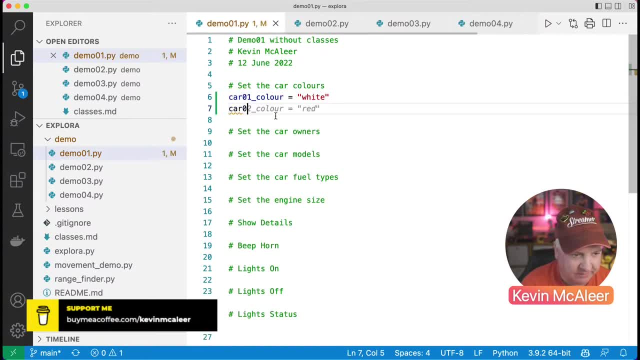 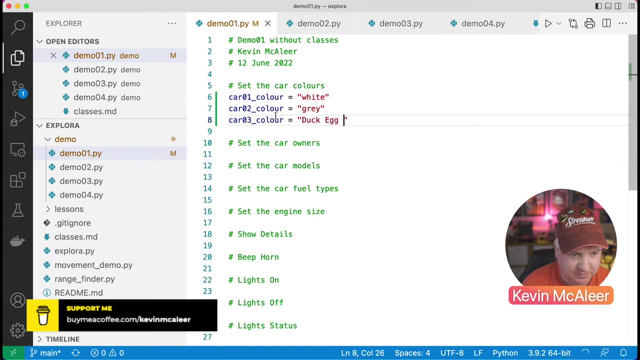 make this my car. my car is white. we can have another car which is going to be gray, and this is going to be jenny's car, and then we're going to have car03, which is going to be alex's car. so yours is duck egg blue, isn't it mint? i'm going with okay, because it looks nicer. 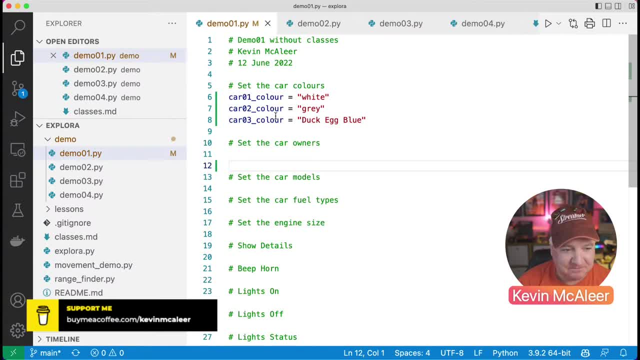 right. so three variables, we put three values in. we're now going to create who is the owner of these cars. so car 01 and then owner, and yep, it's guessed that. right, i've got uh copilot on here. it's going to be the owner of the car. so this is going to be uh jenny cars. what's the name? 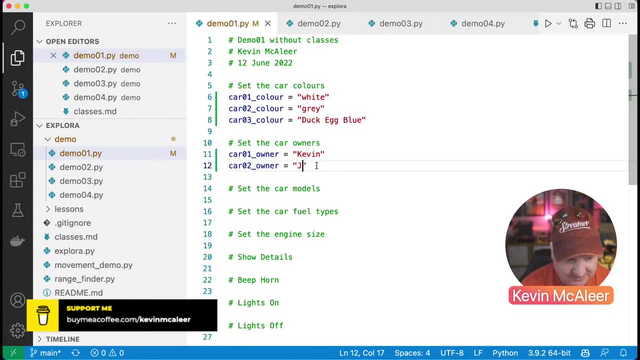 of that, one i'd like to go with- i don't know if you've used this before yourself- which is from github, and it helps you create code in a really smart way so you can do a lot less typing. so this is new to me literally today. so car three is going to be alex. 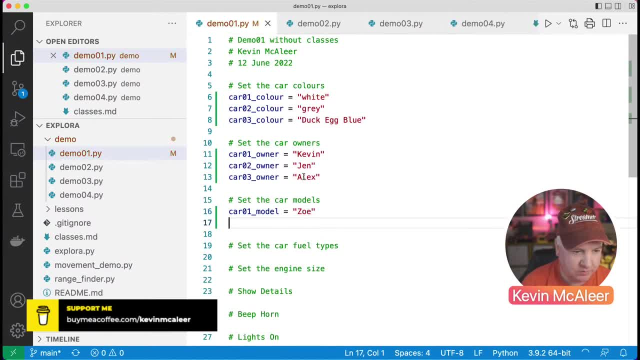 and then next the car model. so let's create another load of variables for car 01. model car. the next one is going to be jenny's car, which is an a-class merc, and then we have alex's car, which is fiat 500. we'll just go for 500 there. next up the fuel types. so let's go for car 01. 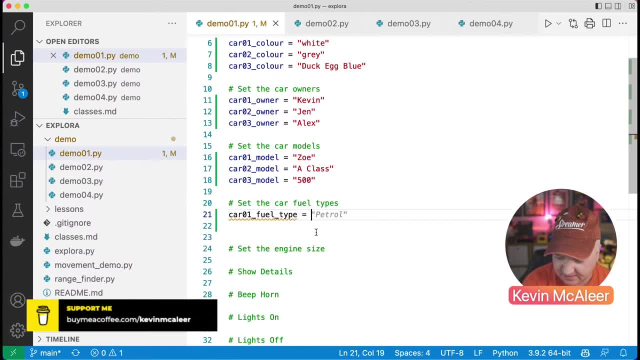 this is going to be fuel type and this mine is going to be electric. i like how it guessed the fuel type that it said petrol, which is pretty clever. car 02 is going to be petrol, absolutely it is. and car 03 is also going to be fuel type. 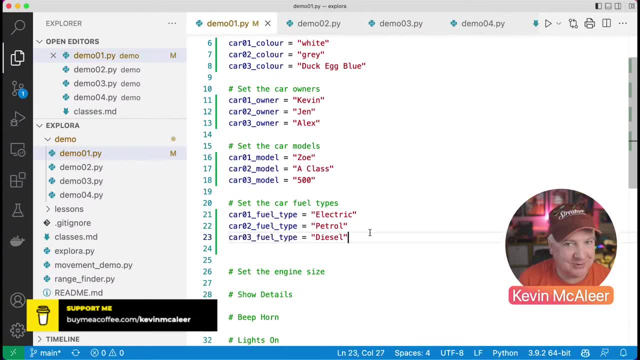 it's guessing diesel, it's not a diesel, but we'll go with that. just because it's different, that's, that's cool, and engine size is right. so i'm going to create another load of variables. you kind of see what i'm getting at here for each of these different things, which is like a car, one car. 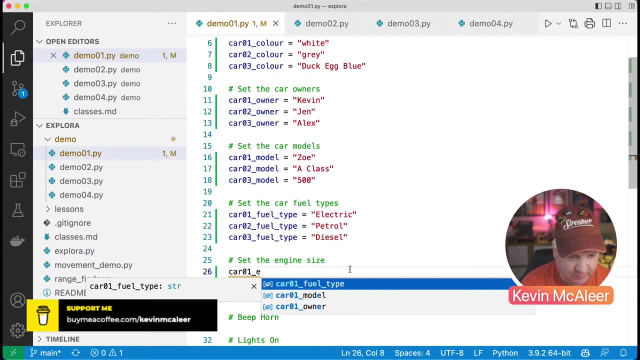 two or car three. we have to create separate variables for each of them. so engine size. so mine isn't um in liters, it's measured in kilowatts, which is small k, big w. so i have an 80 kilowatt motor in mine. car 02 is actually, i think it's a 1.6 liter, and then alex's car 03. 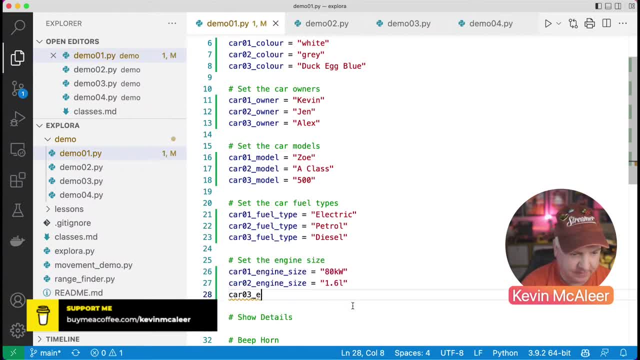 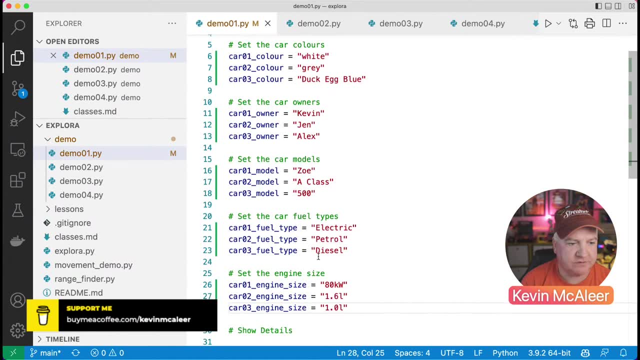 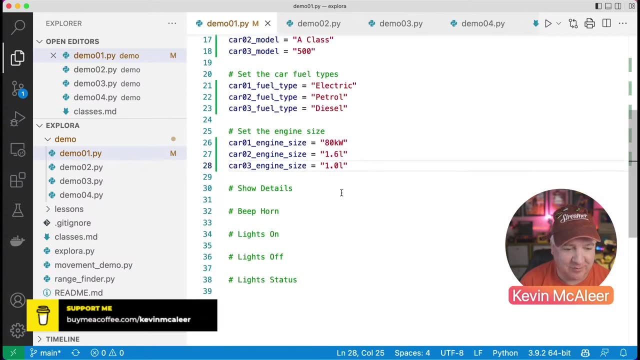 engine size is actually a one liter. there we go, okay. so we've created a whole bunch of variables there. so there's one, two, three, four, five variables for each car that we're going to do. so 25 variables that we created there. they've all got a similar kind of naming convention, so hopefully we can sort of keep hold of. 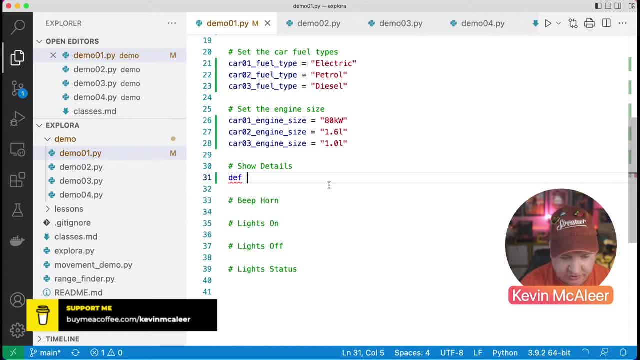 what's going on there. so the next thing we want to do is we want to create a function, so this one is going to called show details, um, details, and this is going to take the color. i'm using the british spelling there because i'm british. we're going to 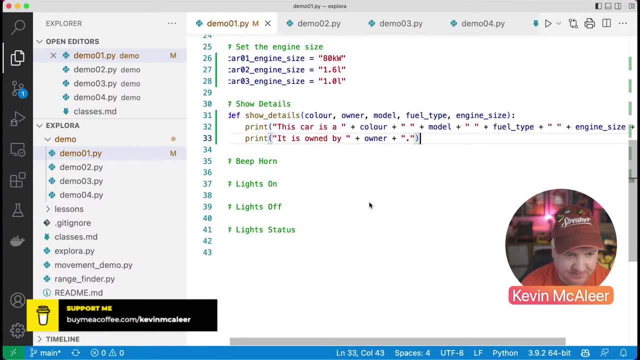 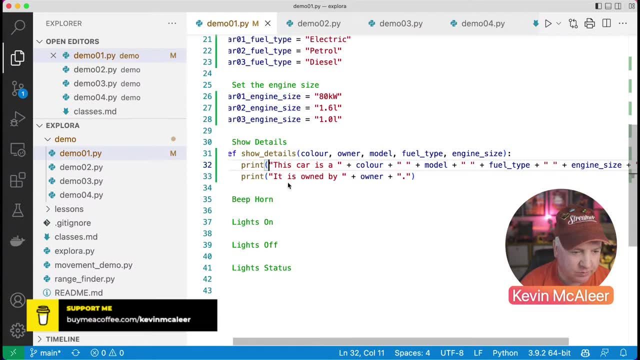 take the model and the fuel type and the engine size. it's guessed it right there. so so this, let's, let's do this slightly differently. so one of the more advanced features we could do: print when we want to print something out in in python and you can sort of break things. 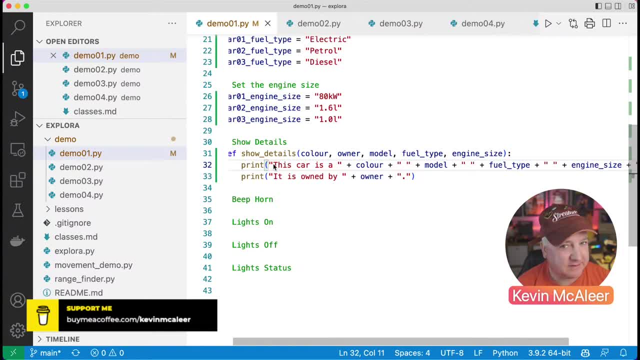 up by having these pluses in between them, but that's actually not an advanced way. so let's start by having one of the more advanced ways of handling strings in python, and that's using an f1 string. so we can instead, instead of having to this plus thing and breaking 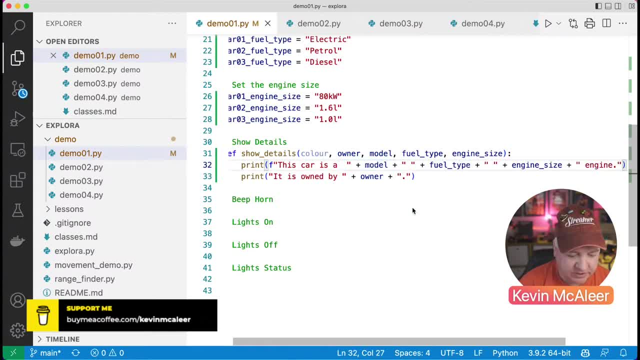 up our our little string there. we can actually use these curly braces and put the variable within that. so I can say the. so let's say the, and then color: it's like the blue car, the red car, whatever, and let's get rid of all this stuff. first of all like so, so the white car is a, and then let's put the fuel. 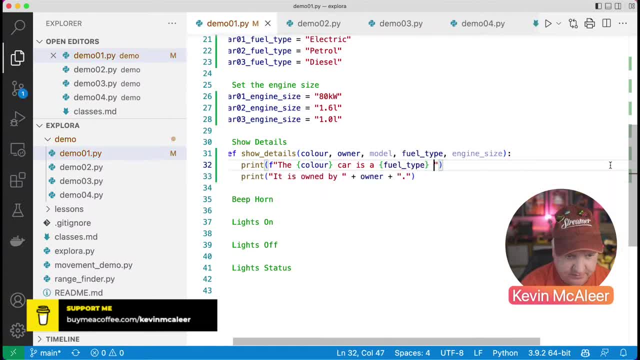 type in there, powered, and then let's put the model and then let's say, and oops, and he's owned by and is owned by, and then let's put the owner in there, brackets, okay. so what's going to happen there is, it's going to interpret this and basically, 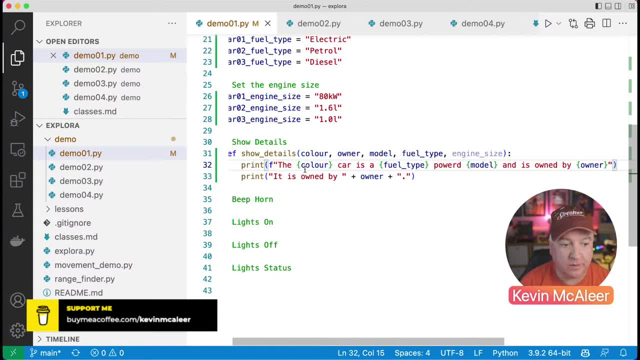 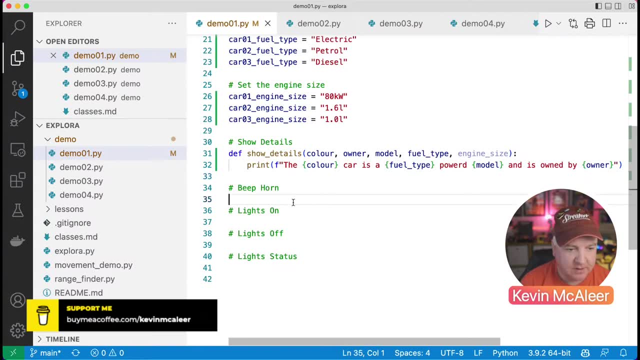 replace these variables with the- the value that's in them within our string- and print out. so let's get rid of that there. very impressed with copilot? oh, it's a creating a lot of our code for us, so that's the first one. it's not going to return anything, it's literally just going to print it out. 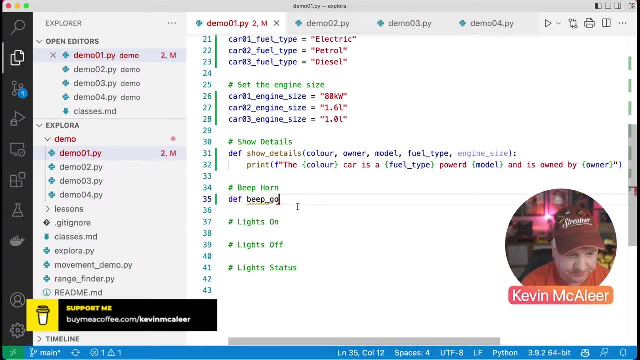 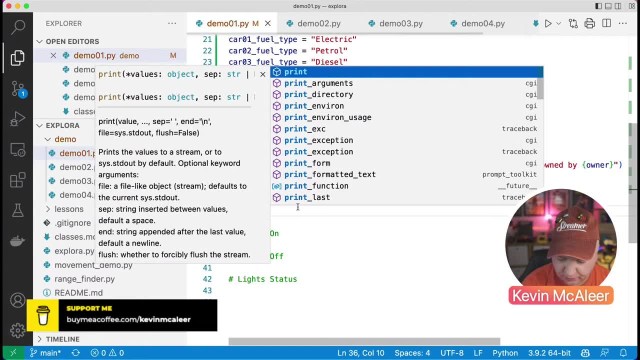 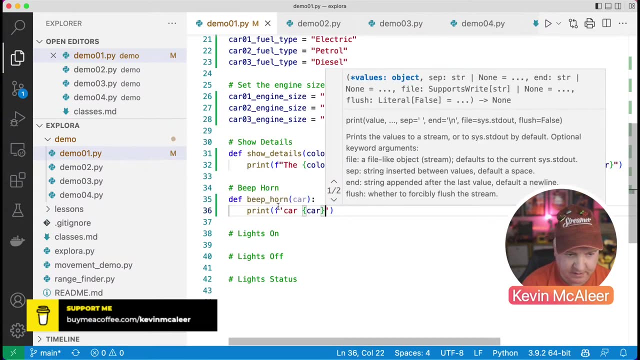 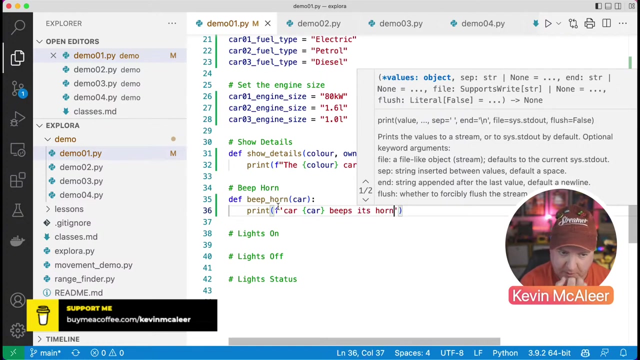 the next one is beep the horn. so let's do beep horn and this is just going to take the car and then we're going to say print, i'm going to use that f string again and we'll just say: car car, beeps its horn. there we go. okay, now one of the things that's a really good idea to do when you're creating. 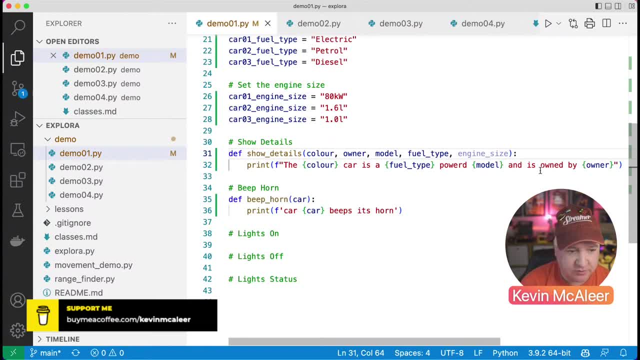 functions is to create a doc string. so the way that we do that is just underneath the, the definition of our function. we do three speech marks and then another three speech marks and then in between that we can put some kind of text about what this does. so shows the car details, and then similarly under this one, 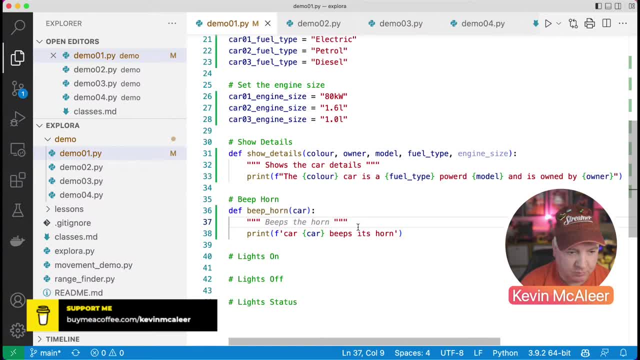 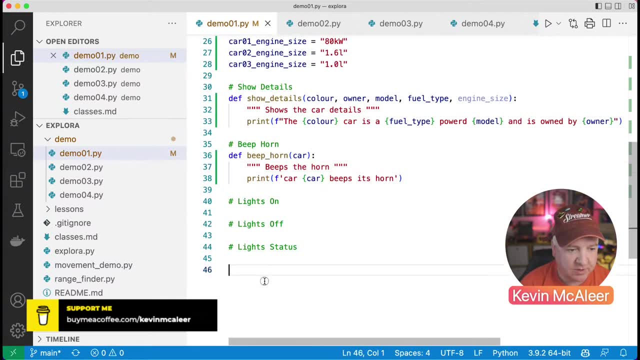 that we've just done for beep the horn. we can just do that again and that's fine. beeps the horn would be good. so beeps the horn. and what that means is when we come down here and we want to actually use sort of a beep horn. if i hover over that, that little piece of text there that appears is what 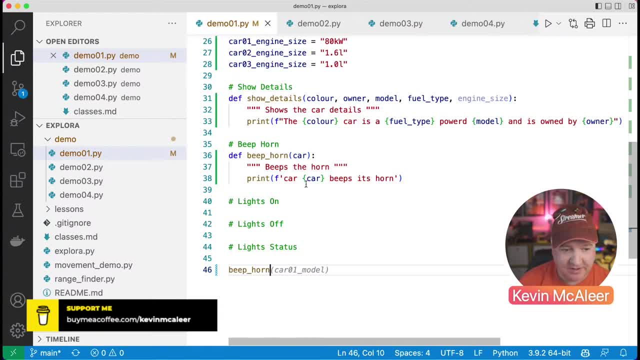 it really stands for bleep, beep beep. you could just type it in the information that's in there as you go down here in the description box. you could turn this on like that. you know, if you don't like something, you don't want to change it. 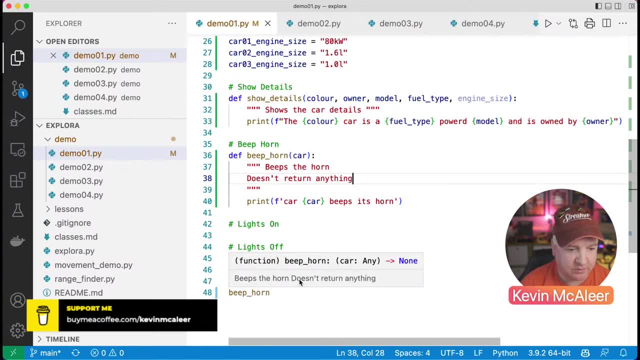 you could just pull it up and it would be an app or whatever. it actually sounds a bit better, yeah, so what we can do here. if i hop over here, הב׶ settlers, you're just going to pull up the text. suppose that your car is the right location. 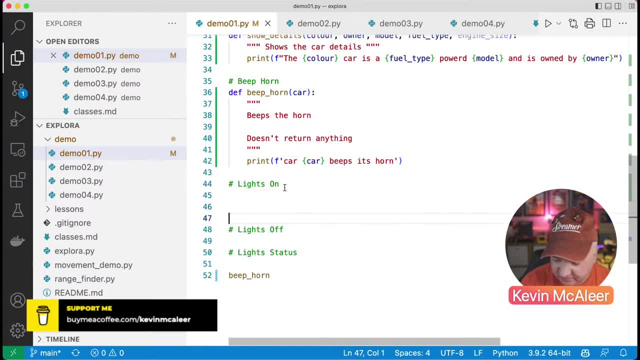 it looks more like conferences. but come on in, everything has a different general inside the commercial, a lot more like the ptv, another couple of functions on here, so we're going to have lights on and this one is going to take nothing, it's just going to uh oops. so let me just back up there. lights on. i think we do need. 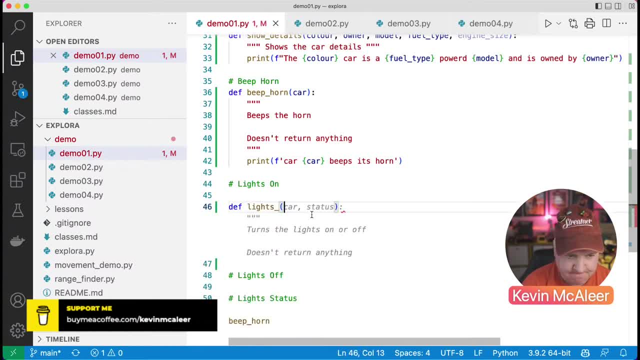 to have the car that it's putting the lights on for. but let me see, i'm just going to say lights on, it's not going to have any variables, it's just going to be empty and it's just going to return, true and similar, with lights off. 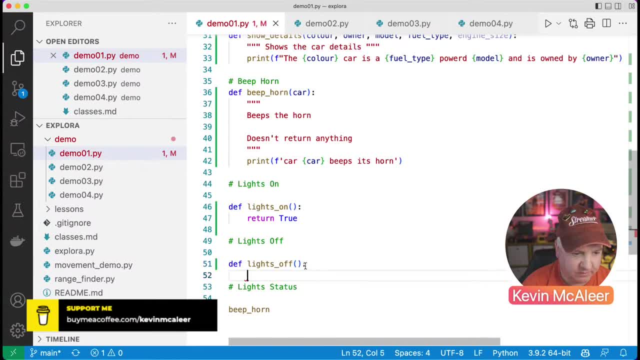 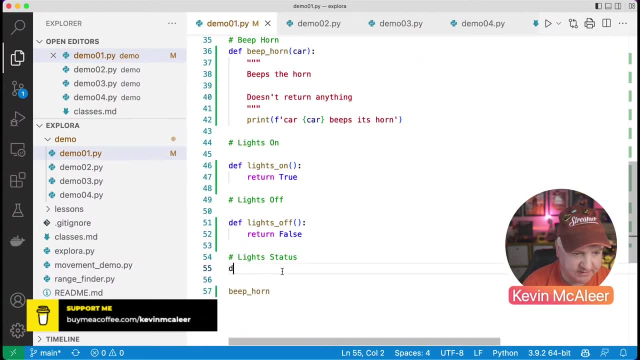 let's just make that lights on that's going to return false. so there we go, and then we're going to have another one which is just what the status of the lights is. so let's say def lights status and then car lights that we're going to pass in as 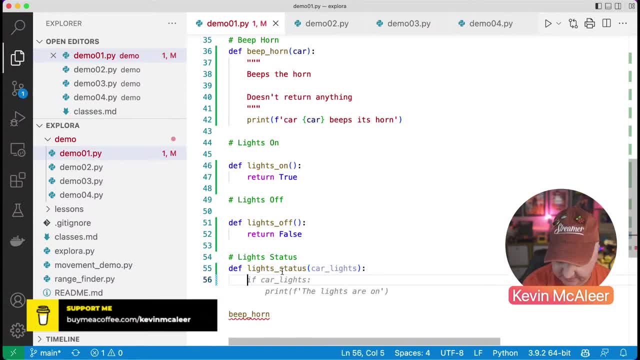 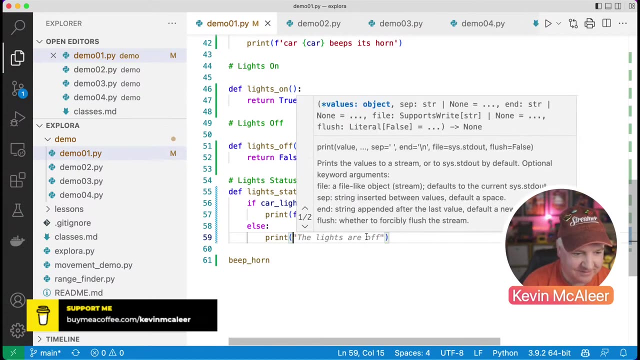 variable, and what it's going to do is it's going to say: if car lights, the lights are, this is cool, this uh. else print lights are off. i'm really liking that copilot. it's basically just writing the code for me here. yep, that's good, do that. so you just press tab to auto complete that, so what? 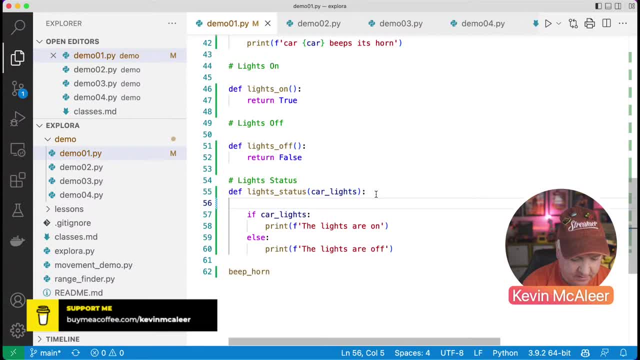 i'm going to do is just put another dock string in that particular one and that's going to say: um, shows the current status of the lights. let's just shows current state of the lights. there we go, okay. so what i'm going to do now is i'm going 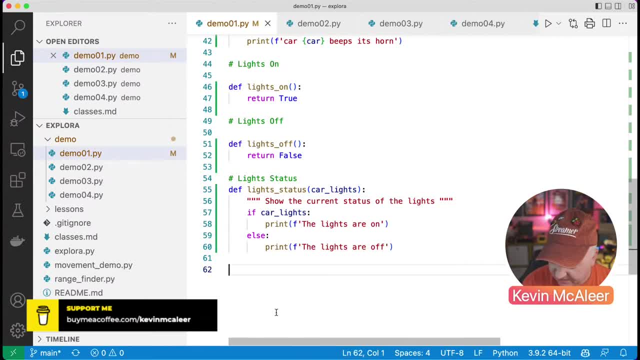 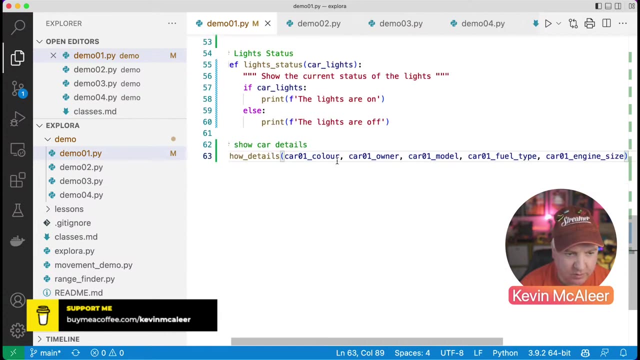 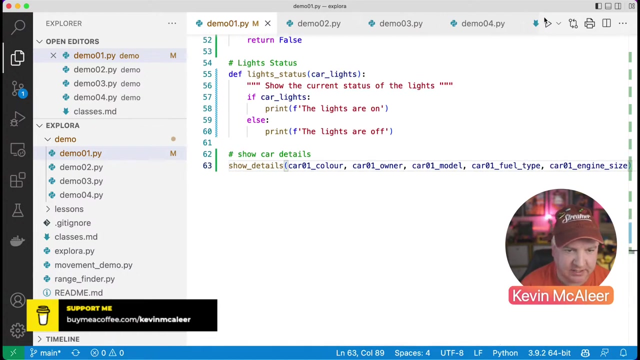 to actually start using this code. so let's come down to the bottom here and then let's say: show car details. so this is a very kind of functional procedural type program. so we're going to take car one, the color, owner model, fuel type, engine size, and we are basically going to run that and have it display. so let's just click run and see. 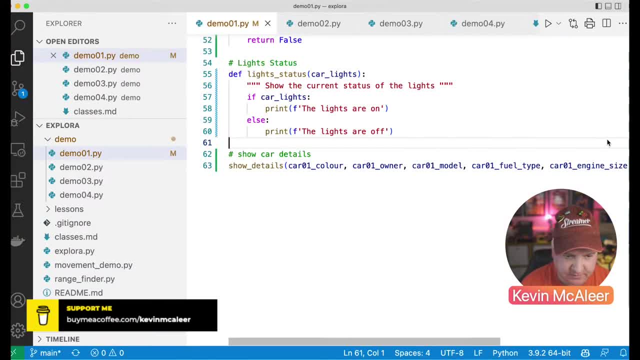 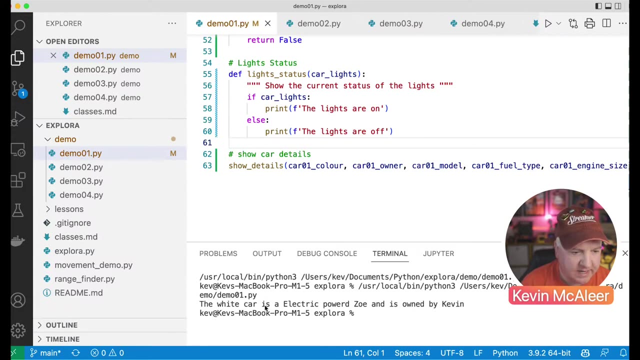 what happens there. oops, sorry, that's up in there. let's try that again so we can see in the little terminal down here. let's just make this a bit bigger. it says: let's just turn off that for a second. the white car is electric powered- with a spelling mistake there, zoe- and is owned by kevin. so let's. 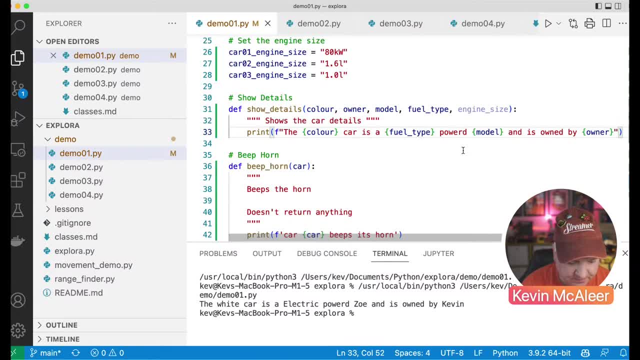 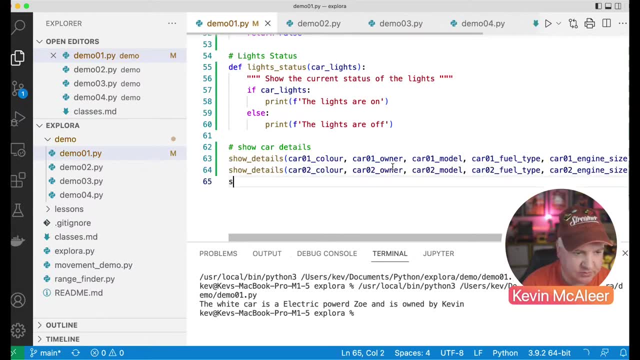 just change that, powered by, to correct that typo. okay, so what we can do now is we can do the same for all three. so do show details, car two. show details, car three. i'm loving the way it's also filling this out. i'm just so not familiar with this. um, it's new to me too. there we go tab to. 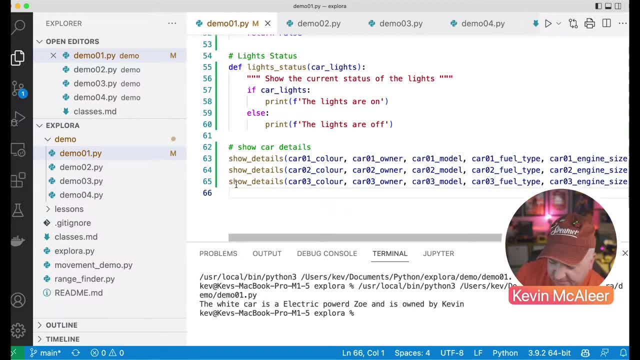 complete return, which also gives us a very nice little bonus, if you like, in the link, in the description. and then we're going to beep the horn for car one. so let's do that. so beep horn, and then in brackets, car 01, just passing in text, and then we're going to say car. 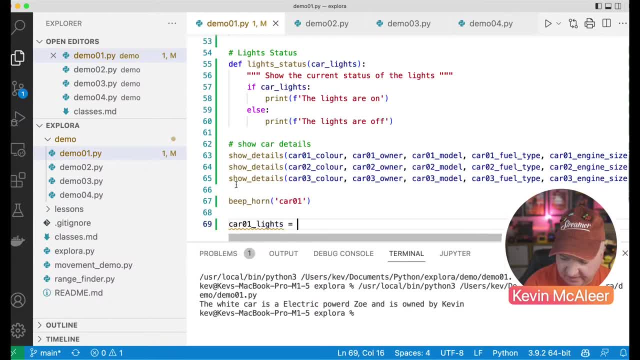 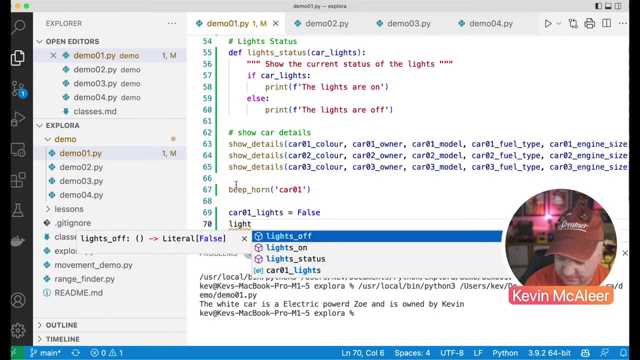 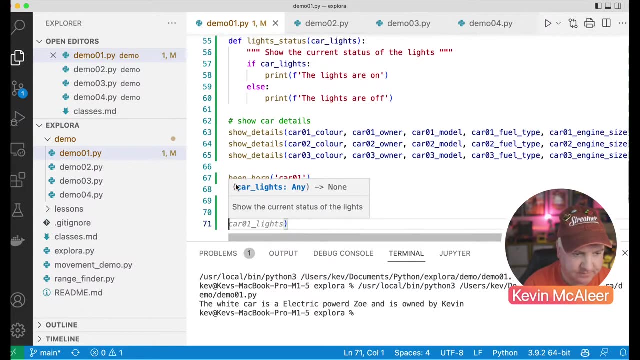 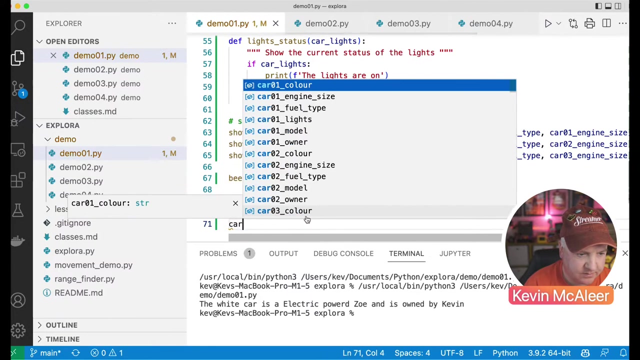 01 lights, which is a new variable, equals false. we're going to make that false to begin with, and then we're going to say light status like so, and then pass in car one lights, okay, and then we're going to do lights on, so car 01 lights, equal lights on. 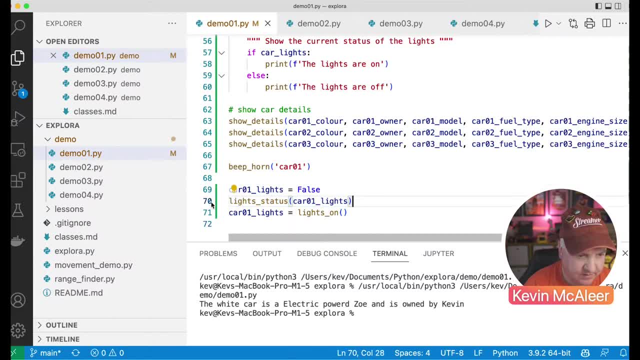 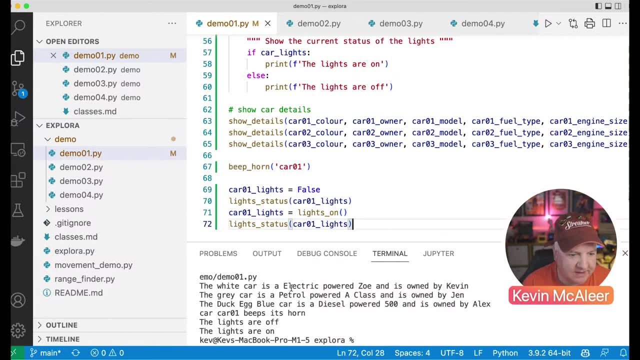 and then we'll do the status once again. okay, so we should see three details and we should see the car lights off and on and also the beep. so the white car is electric powered, zoe, and is owned by kevin. the gray car is a petrol powered. 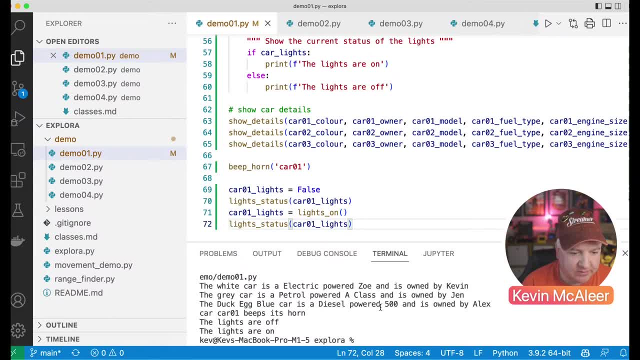 a-class and is owned by jen duck. egg blue car is diesel powered. 500 is owned by alex car. car one beeps its horn. the lights are off, the lights are on. so that's how we do things if we don't use classes. so it's quite a lot of repetition there we're having to repeat. 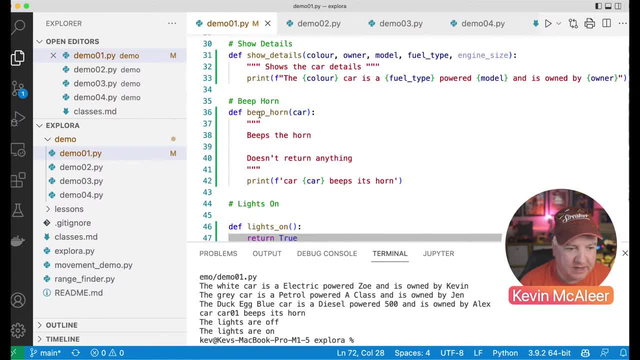 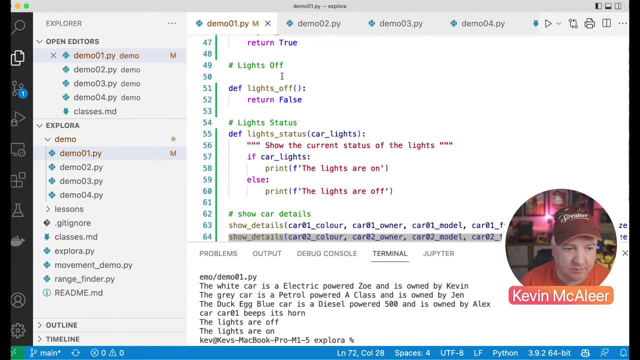 variable names multiple times. um, we're then having to, and this- the functions- are completely disconnected from the variables themselves. there's no concept of this all being together. we've got lights on on, lights off, um, we've got a status thing, and then we're just doing some. 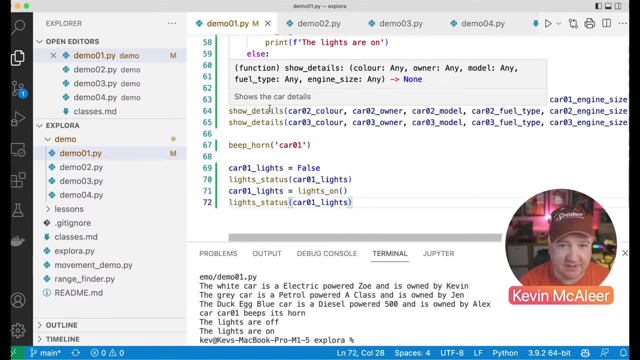 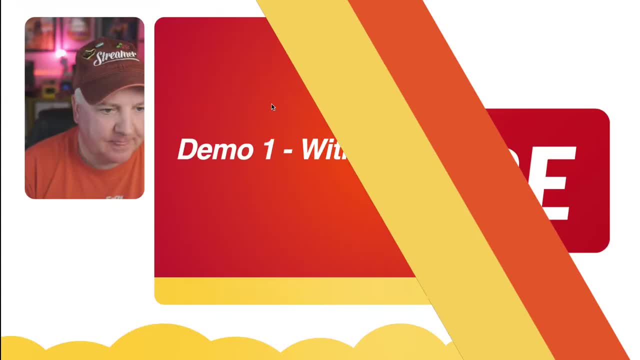 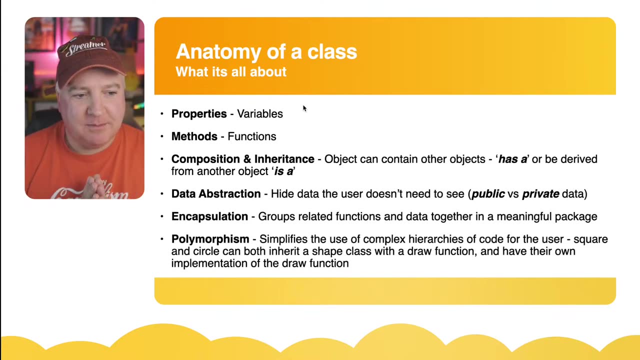 settings, some showing some variables, and again these are not connected to the variables, they're just standalone functions. that's what it looks like without. so let's get back over to our keynote and let's continue our journey. so so, properties and functions- uh, properties and variables. methods are functions we've talked about. 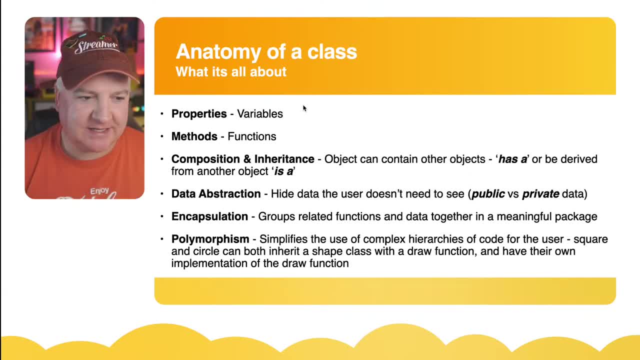 that a second ago. this is all about the anatomy of the class, the composition and inheritance. we're going to have a look at inheritance in a minute. so when we talk about classes, or and objects, they can be composed of things. so they're made up of things, or or and or. they can also be inherited. 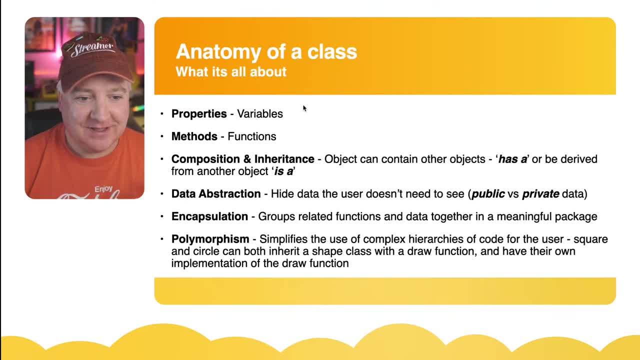 from things. so what we say is: an object can be composed of things, so they're made up of things. so typical of things we think about: contains other objects, so it has a another object or if it's derived from another object, another class. we say it is a. so hazard is how it's composed of. 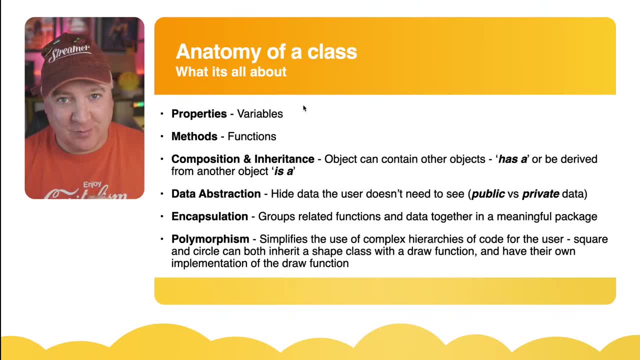 so if we're making a robot, the robot class might be derived from a base class of robots, and this one might be a specific one, with wheels instead of legs, for example. so, and then it has a. they might have a motors for turning wheels. it might have a. 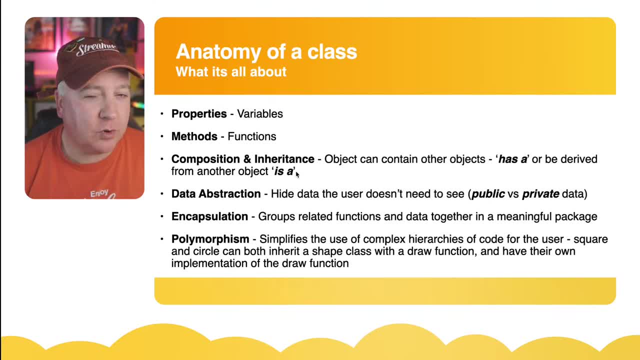 things, um, distances and so on, and that'll become a lot more clear in a minute when we get into some of the- uh, the modeling of inheritance- sorry, nice stomach rumbling there- data abstraction. so when we were creating our cars then we were creating all the different statuses of various different 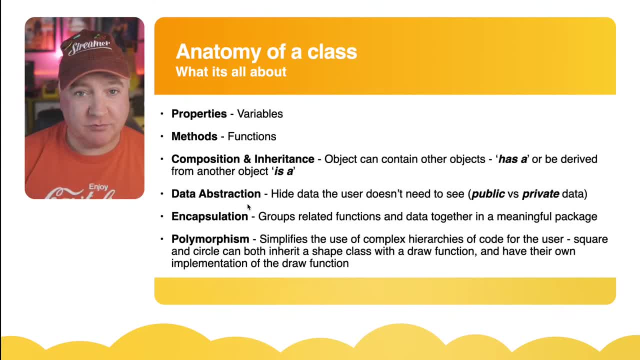 things. all that data is completely public. anyone who's writing, who's sharing our code, can see exactly how that works and they can also fiddle with them. they could also change the value of this and unless we've got really robust error checking, it could actually break our code. 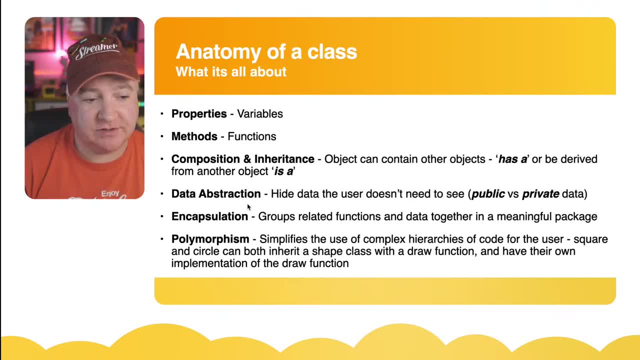 sometimes we don't want that to happen. we want extra error checking within our functions and then hide them away so that the user doesn't know that's happening. they just, if they pass bad values, it'll just return an error. so that kind of abstraction is a key part of object oriented. 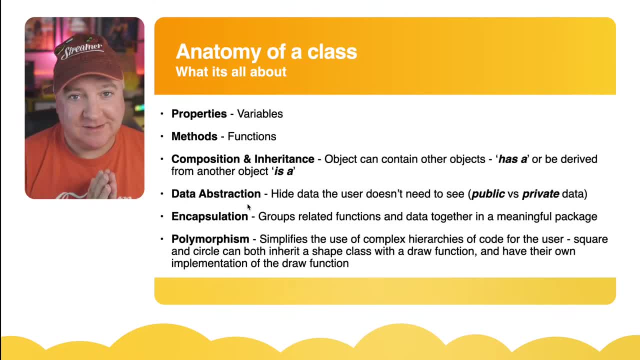 programming and we call this public versus private. so the very simplest level: we have public variables which we expose in our class and we say: you know you can change these, and we give them an api, an application programming interface, to do that. or we have private data inside our class that only we 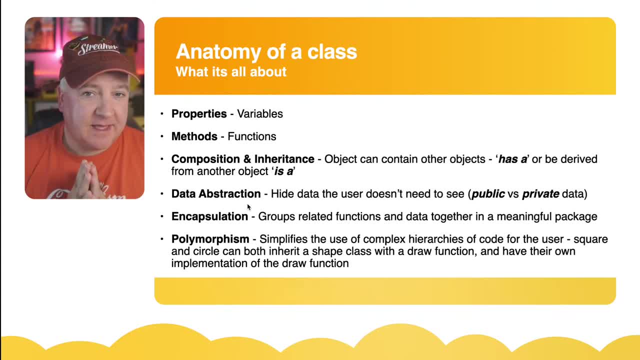 know about and that's just how we internally represent it. and that means that we can change how we do things internally. and as long as we don't change those public facing variables, those properties and methods, then everything will carry on working. so we can really change and 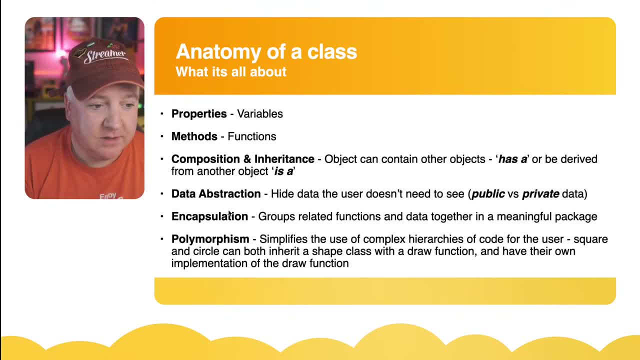 make our code more efficient without the user ever actually knowing about that. encapsulation is where we group together functions and data together to make a package which makes sense. so if we want to model a car, you can probably start to see what kind of things we will put into the class from a properties point of view and also from a method's point of view. 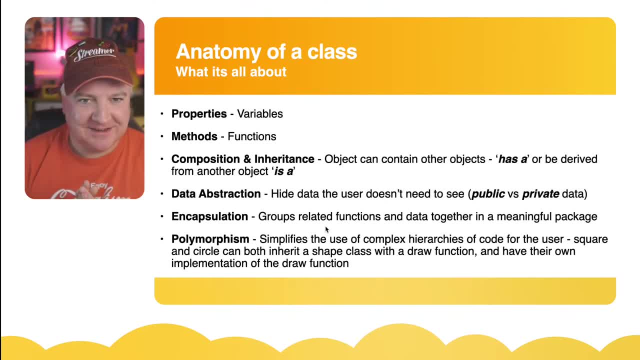 and then there's this really unusual word in object oriented programming called polymorphism, and it sounds really complicated and you can get your kind of knickers in a twist with this one if you've not come across this before. but simply what it does is it simplifies complex hierarchies of 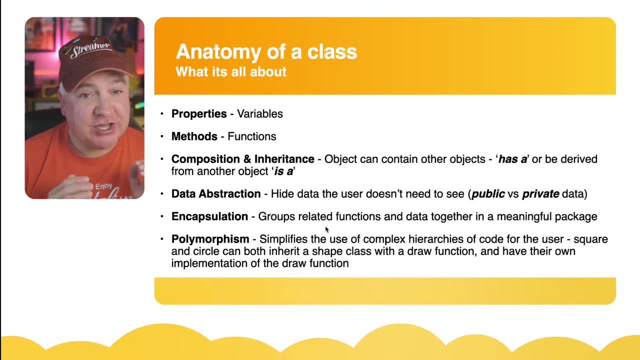 code for the user. so, for example, we could have a shape class and the, we could have a circle class and a square class, and they both inherit the common shape class. so shape might have an area, for example, whereas a circle might a very specific formula for working out what the area of a circle. 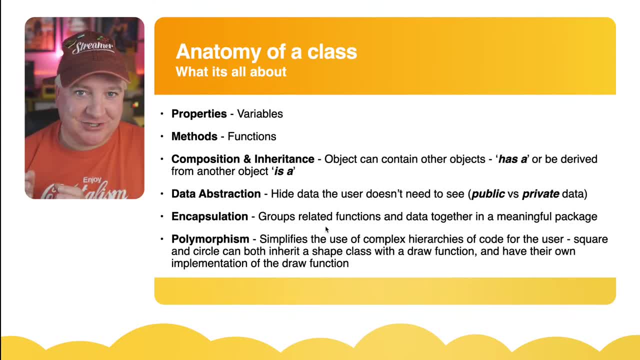 is- and not any points for people who guess what that is in the uh, the chat- and also, you know, an area of a square or a rectangle or a triangle or whatever. that would be very specific to that type of shape. so we can have a common class and then we can, we can have other classes which inherit. 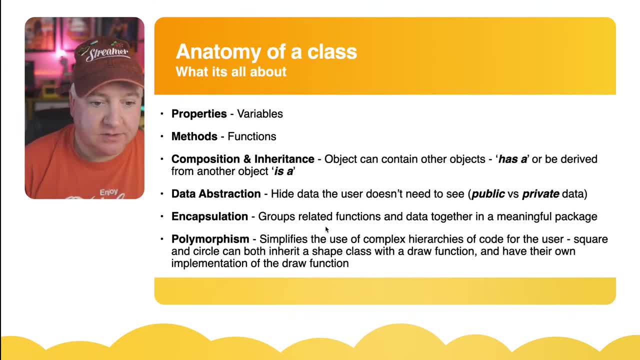 that, and they're subclasses of that sort of super class, so they can all have their own implementations for drawing, for example, but they all have that common ancestor, which is the shape class. it just means we can create code once and then the things that inherit it can just automatically pick that. 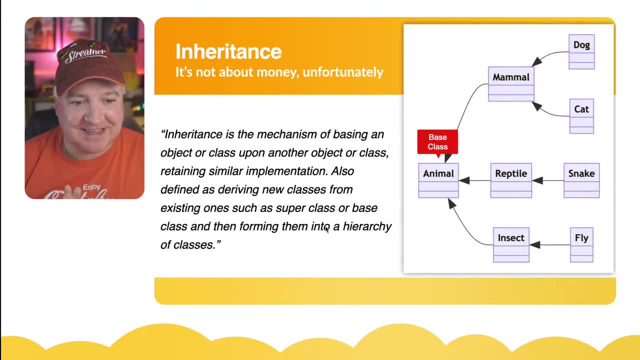 up. okay, so inheritance- let's get into this a bit deeper, shall we so? inheritance? this is from wikipedia. inheritance is the mechanism of basing an object or class upon another object or class and retaining similar implementation, also defining as derived from new classes existing ones, such as a super. 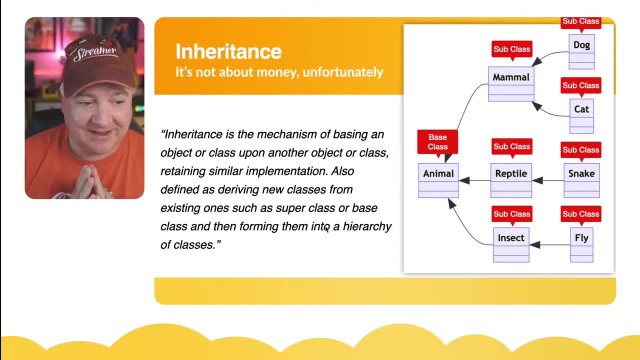 class or a base class, and then forming them into a hierarchy of classes. it is indeed pi r squared, richard. well done. so we can see: here i've got a hierarchy of classes. i have animal, which is our master super class. we then have mammal, which is a type of animal- i was like second guessing myself- then we have reptile, which 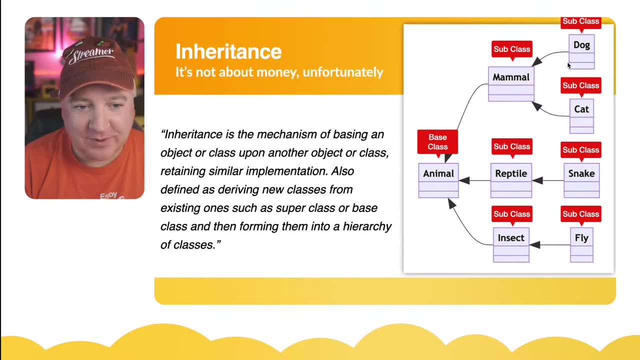 is another type of animal, and we have insect. and then we have a dog, which is a type of mammal, and cat, which is a type of mammal, snake, which is a type of reptile, and fly, which is a type of insect. i hope i got that right and we're going to have a deep dive into this. 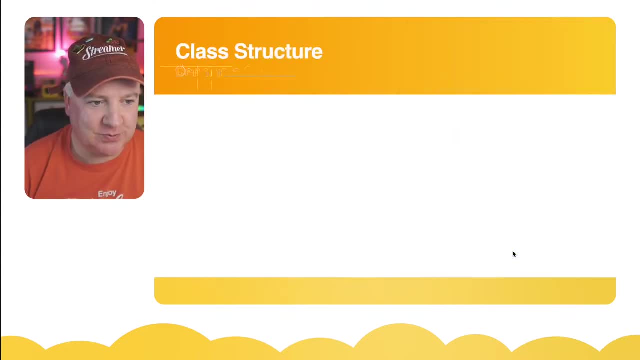 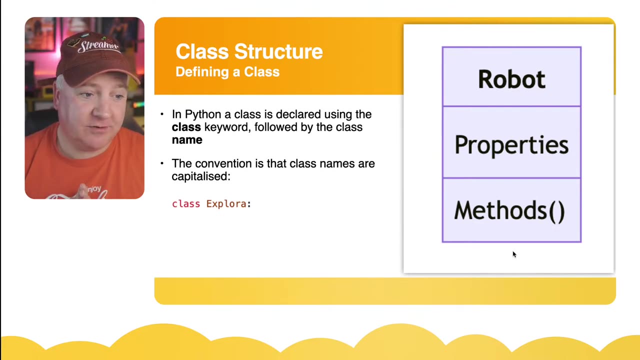 in some code in a minute, so we're gonna have a real good play with that too. so class structure: how we define classes. so in python it's declared using the class keyword, followed by the class name and the con. the convention there is that you have an uppercase. 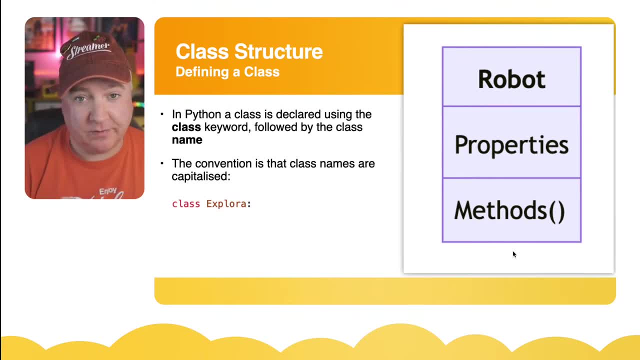 character, which we don't normally do in python, but we have an uppercase character with class names to differentiate them from everything else. so just the first letter is capitalized in the class. that's what we need to do. just say class explorer, for example, which will define our explorer class. 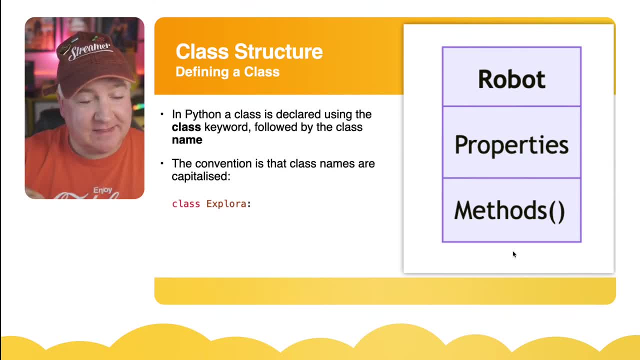 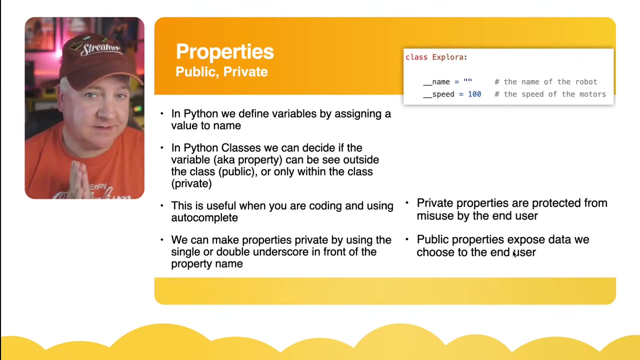 and then we can start creating some variables. under that we indent them as we would with the regular code, and we can also have some methods, some functions. so variables and functions. so we'll have a look at that in a moment or two. so the properties: they can be public or private, and 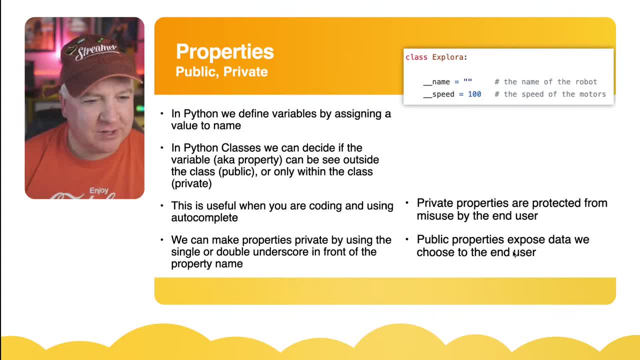 this is one of the more advanced things. i remember somebody saying a while back that they got really confused with why we had underscores and double underscores and some of our variable names within a class, and it's to do with how we make things public or we make them private. so in python we 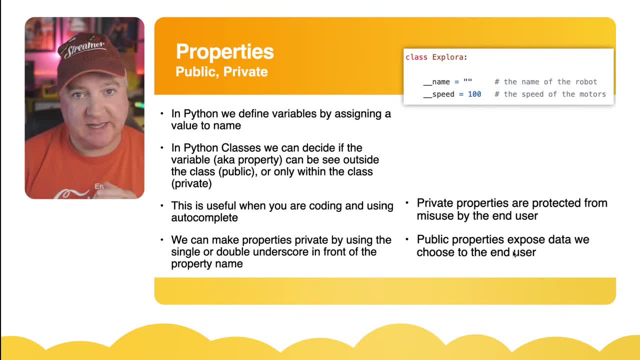 define variables by assigning a name to a value. so speed equals 100, for example, and in a python class we can decide whether that variable is that property, i should say can be outside it's public, or whether it's within the class- it's private. and the way that we do that is by using the double underscore or not the double underscore. 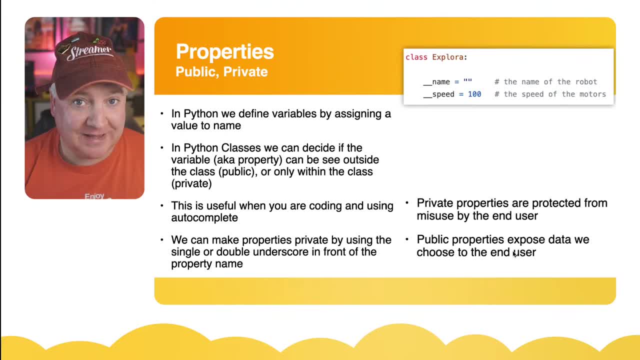 this is really useful when you're coding and using things like autocomplete or copilot, and we can make our properties private using that single or double underscore in front of the property name. so the single underscore is a way just to give some kind of weak protection and it's to do with namespaces. it's to do with when you're 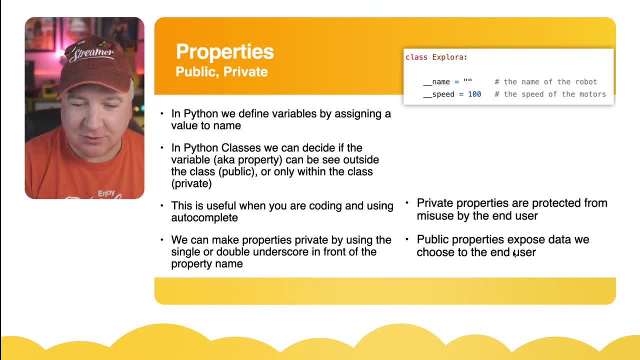 writing your code and how python puts them in a dictionary and so on. putting the underscore puts into a different place within its. in the sort of structures within python, the double underscore really does hide them away from users. so it's it's not a massively secure way of hiding your. 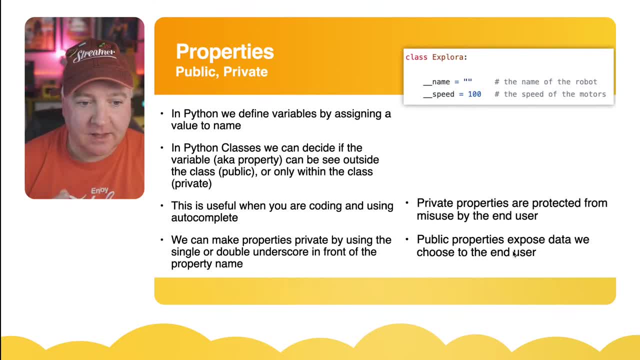 implementation, but this is the the way that we do it. so private properties are protected from misuse by the end user, and we'll have an example of that in a minute with the speed function we'll have. we'll put some extra code in there. public properties expose data to the end user, so 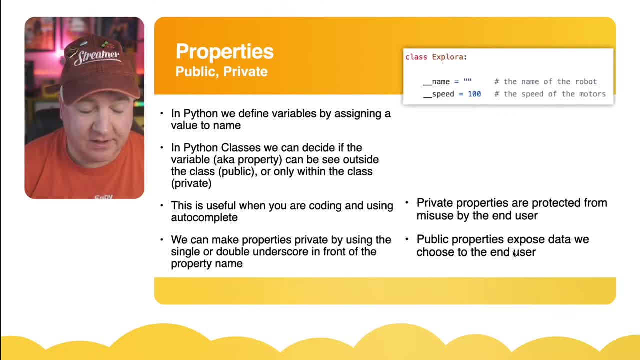 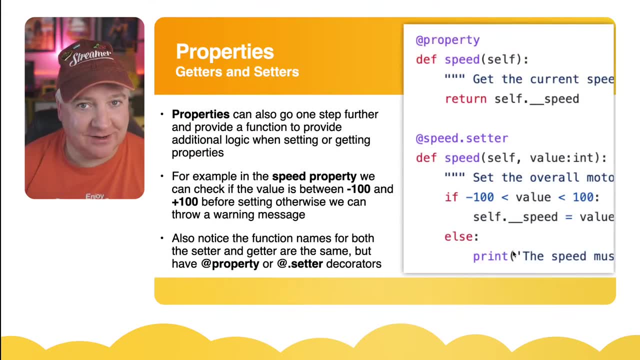 that's something we definitely want to share and we want them to let users do whatever they like. with that. we're making that nice and public. so, properties, getters and setters- this is a very common pattern in python programming. so if we want to create a, a property, a property is a function. 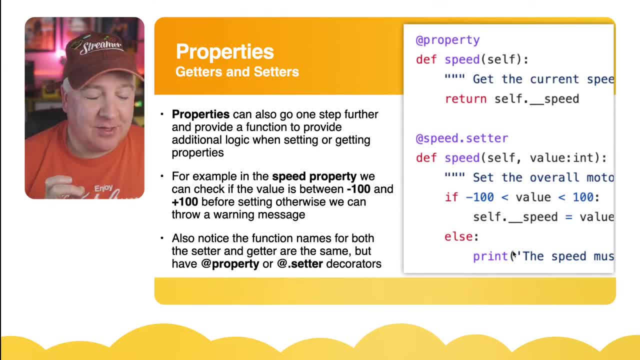 that behaves like a variable and a property is a function that behaves like a variable. we can do some clever logic within the function. you can't normally do when you just have a variable. so, for example, i could just have in my class a variable, a property called speed, and it's 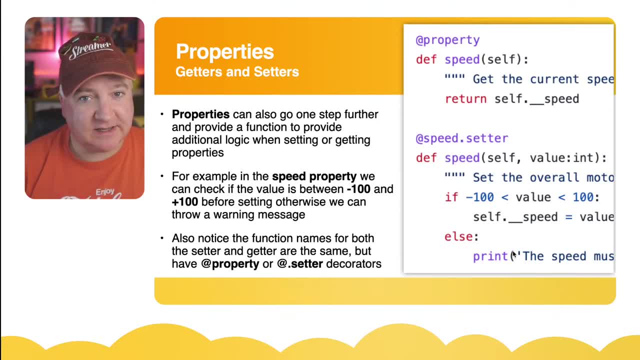 just a regular variable and if somebody's using that class, they could see that speed variable and just assign it whatever they like. they could assign it characters, numbers, whatever they like. if we want to restrict what they do, we can use the property function and we use that decorator. 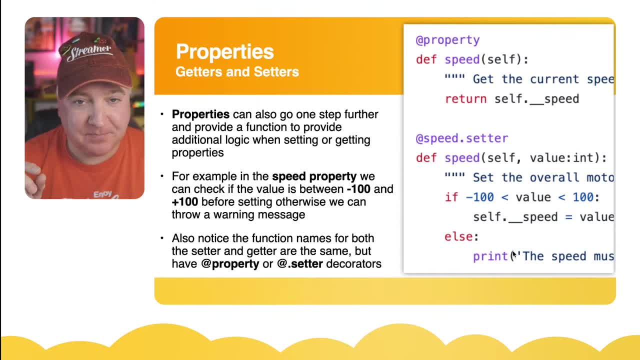 the at symbol above the at symbol. we can use that decorator, the at symbol above the at symbol. we can use that decorator, the at symbol. we can use that decorator, the at symbol. we can use the the function name and then that means to python that this is a special kind of function and it will use that. 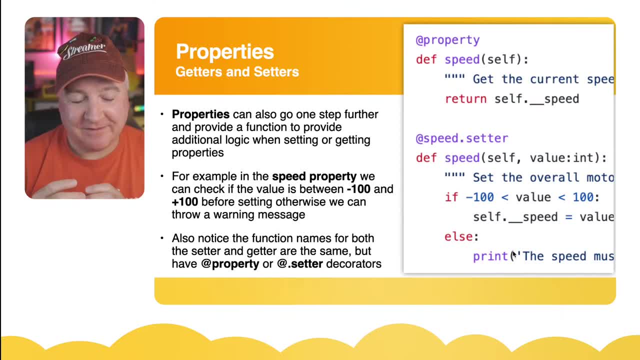 decorator to make the the code have extra functionality. so we'll get into that. it's easier to demonstrate and show you what i mean by that. so in this example here we've got the speed property. we could check if the value is minus 100 or between minus 100 and plus 100 before we set it. 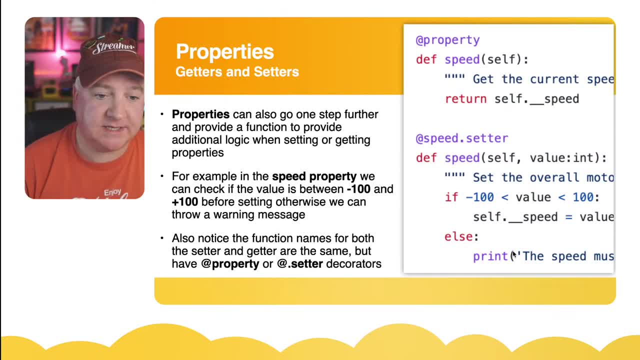 otherwise we can just say not within that range and we can throw an error message. so you can just see some of the code peeping out there. and that's what we're going to do. we're going to go ahead and see some of the code peeping out there. so we've got two things. we have the, the getter and the. 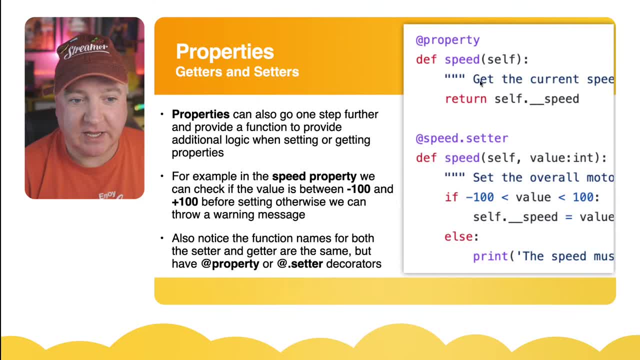 setter. so by saying it's a property, we're saying that this function here is just going to return a value and it's going to return the under double underscore speed variable. don't worry about what self means, we're going to come to that in a minute. so it's going to return the speed now when we set. 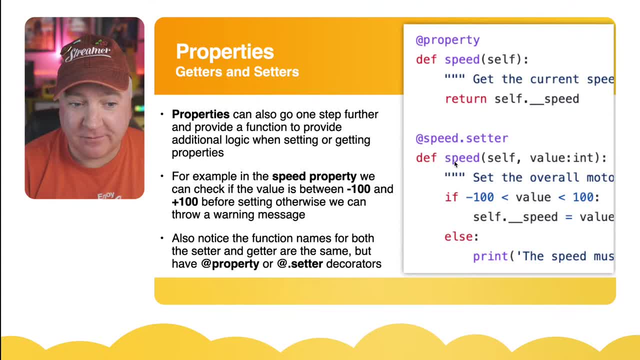 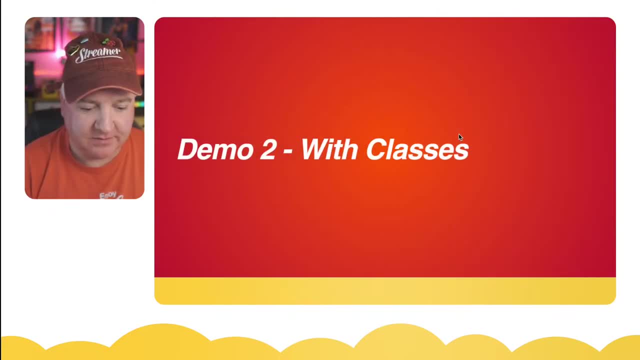 the value. we can use this other decorator and we use the function name, which is the same if you look at both of them. normally that wouldn't be a valid way of you couldn't have two functions, oops, with the same name. so i'm just gonna. 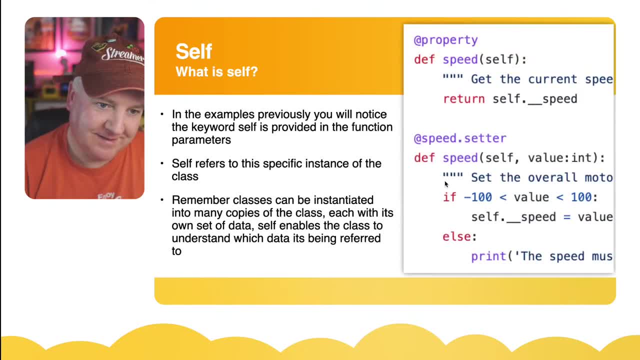 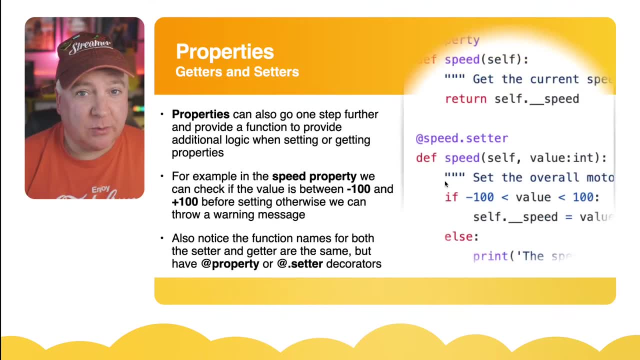 a bit too far, though. let's just back up, back up and just go back to that one there, okay. so yeah, normally we couldn't have two functions of the same name, but when we have that decorator, it actually changes the name and it becomes a different thing. so a property is something where it just returns a value and, um, a setter means 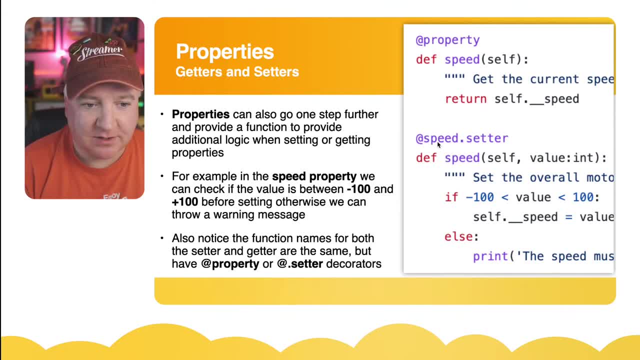 that we can set the value. so get and set. so by having that variable, the function name, dot setter, with the decorator in front, that means this is going to be a special function for setting values and the difference is when you normally have a function you have the brackets at the end. 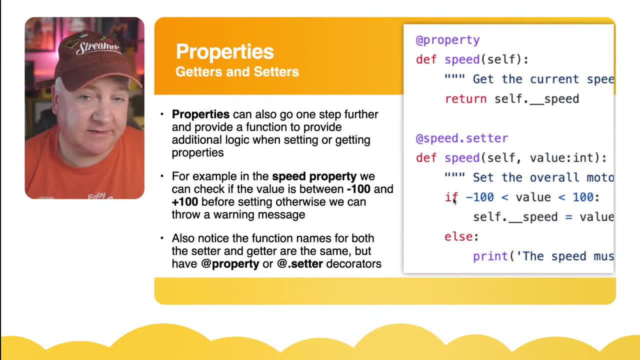 by putting that decorator there, it removes the brackets and it treats it as if it's a variable. so it's really quite clever. so, speed, we pass in self, which is something we're going to look at a minute, and then we pass in a value and i'm saying- i'm using this colon here to say the 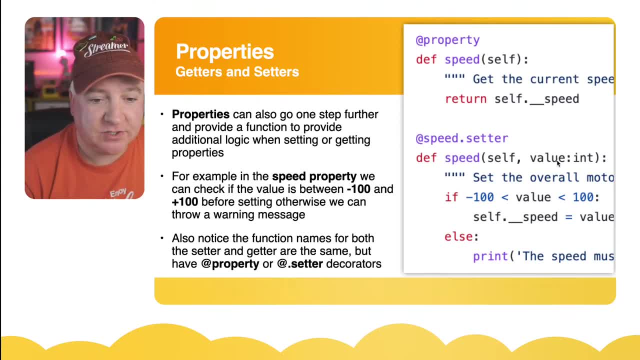 the value that i expect to be passed here is an integer, so we can give it a little type hint to say that this is an integer, and if somebody types something that isn't an integer, it will actually throw an error in the code. so it's a way of protecting our code to make. 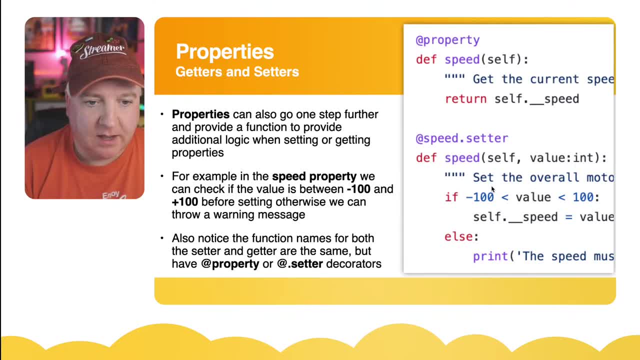 sure that it's actually the right type being passed through and what we see, and we could actually include that on the end of this speed one, for example. so if this speed is going to be an integer, i could do a dash and then a right arrow bracket to say that this is. 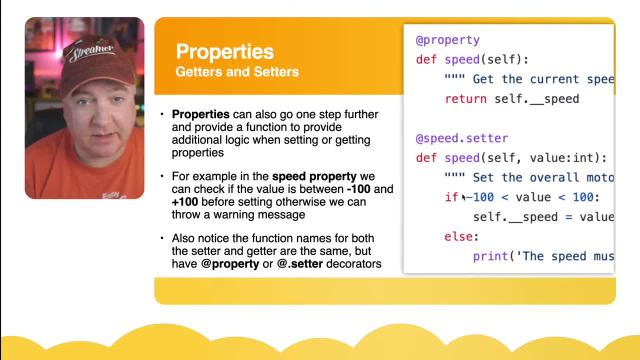 an integer. i'll show you that in a minute. so then we then do have a little code that just says: if the um- if minus 100- is less than value is less than 100. that's a very similar way of saying if value is less than 100 and is greater. sorry, if value is greater than. 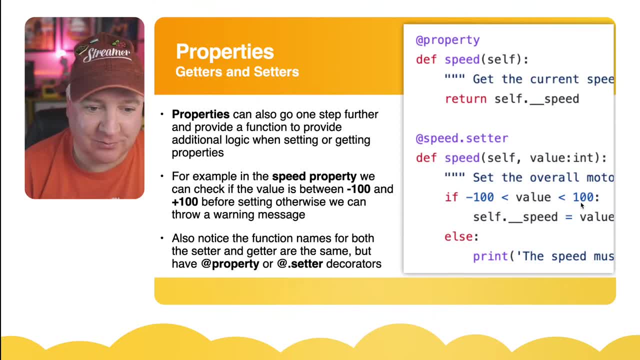 minus 100 and less than 100, then continue. that's what. that is a way of saying. that's another bit of advanced python for you there. and then we say, um, selfunderscore speed equals value, so whatever is in that value, if it's between those two values, within those values, then it's going to be okay to set. 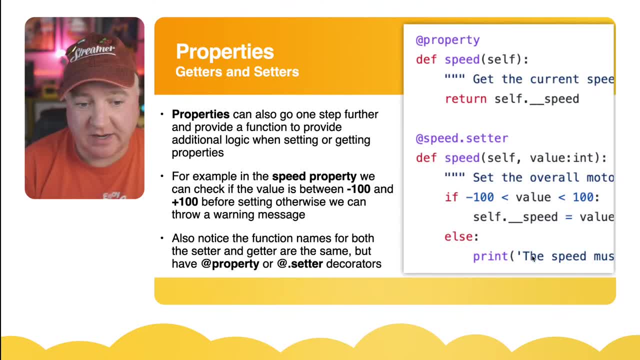 the internal value, which is underscore speed. otherwise print a message that just says the speed must be between minus 100 and plus 100. so that's what that's about and you'll also notice it says there the function names have. setter and getters are the same, so speed and 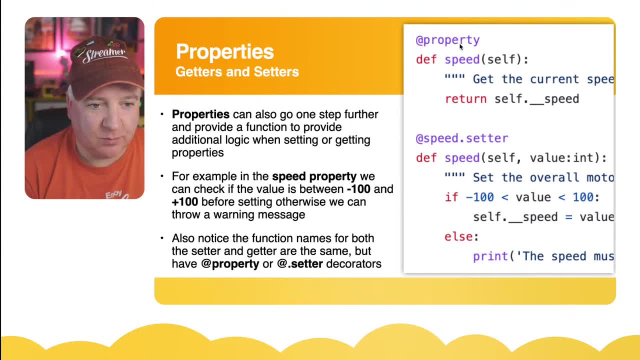 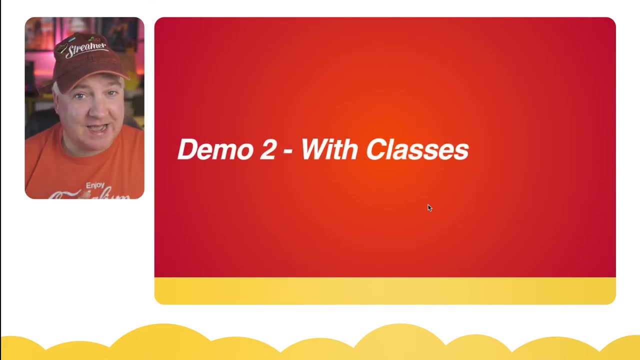 speed. but they have properties. they have decorators property, which is for getting variables, and the setter, which is for um setting them cool. so let's have a look at how we would do the same thing we did before with the cars, but using classes this time. now we've learned a little bit about. 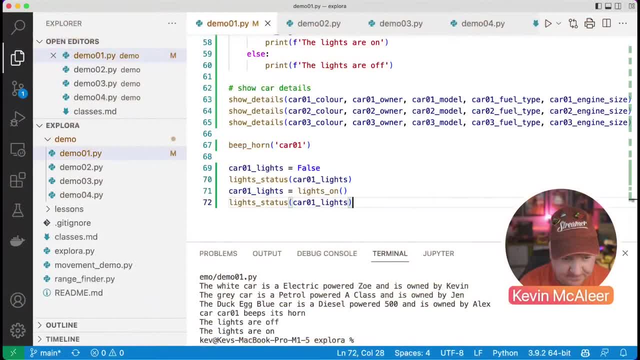 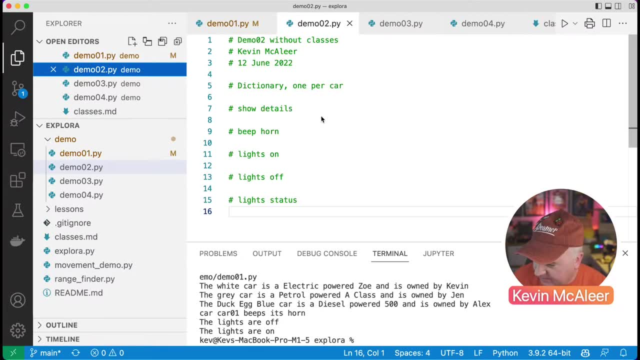 classes. so let me get back over to here and we can now go over to demo two, and i've got my uh skeleton code ready to go. so the first thing we're going to do is um, or actually i'm going to do is um. actually i'm going to do is um. 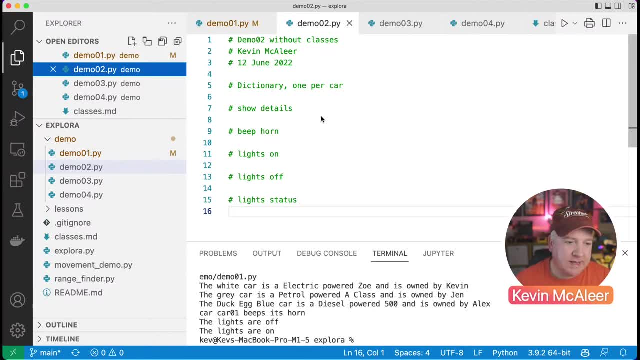 actually, um what i can show you. there's a slightly different way, um of of doing what we did before, but instead of using individual variables, we can just use things like dictionaries and lists, um just to make it a bit more efficient. i'll show you a bit of that, but essentially the 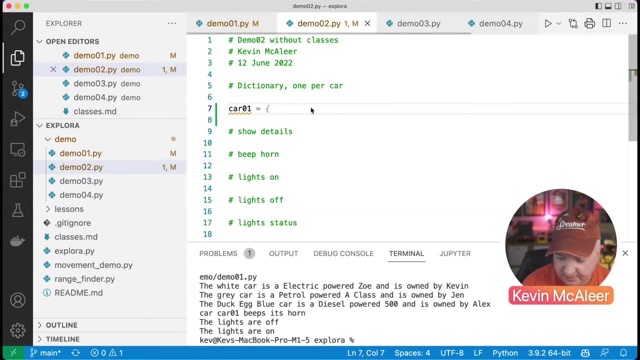 other code is exactly the same. so if we say caro1 equals and then we use um- this is going to be a dictionary, so it's got the squiggly brackets- we can then say color and then equals white, we can then say: look at that, it's guessing what i'm going to type there, which is pretty. 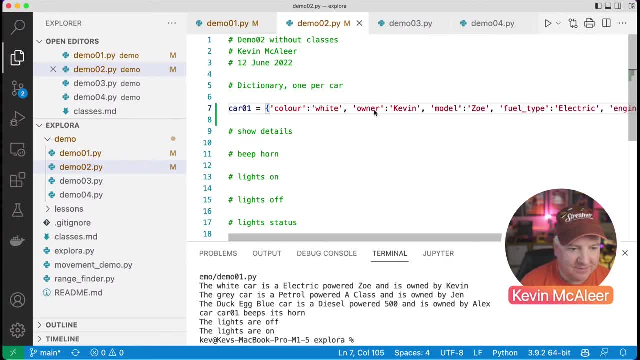 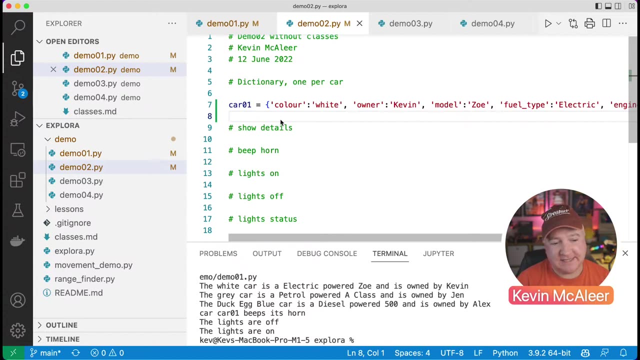 clever. yep. it's then saying the owner is kevin, the model is zoe, the fuel is electric, the engine size is 80 kilowatt. that is clever, that it's remembered that from the previous piece of code and what that means is we can keep all of those different variable values together in one variable. 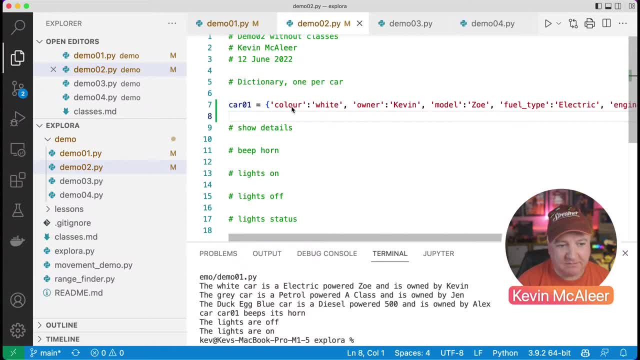 so it's a bit more efficient and we have got the- the name of the, the variable, if you like- in there there's like a key value pair. so that's a slightly more efficient way of doing what we did on the previous one, but it still doesn't bring together, it doesn't encapsulate or protect these variables. anyone. 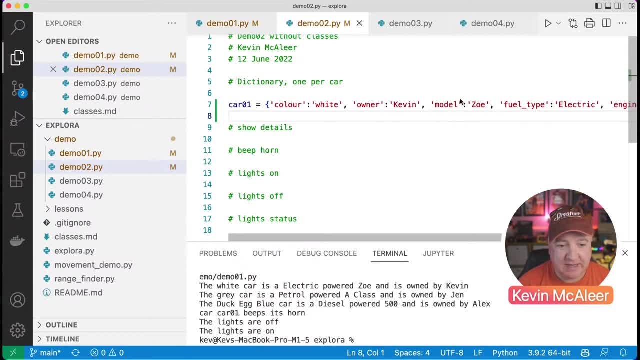 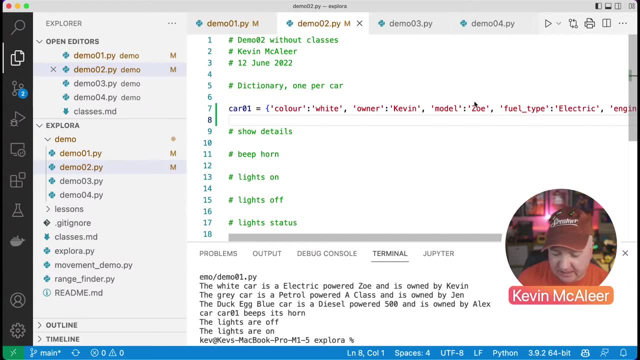 could come along and say color equals blue or speed equals 200, for example, and break all our code. so that's just another way that we could actually do that without um, without classes. so i'm not going to type all that code in, because i think we pretty much covered that off on the previous. 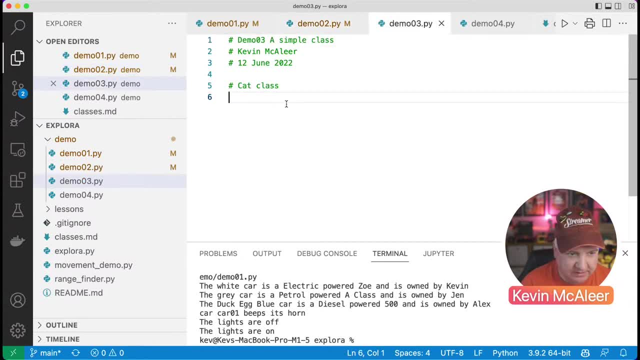 one, but we are going to look at with a simple class. i'm going to do- not cars this time, but an animal. so let's create a new class and this is going to be a cat. so now, interestingly, copilot is going to type out some extra stuff for me here, and we pretty much want this, so i'm going to press tab. 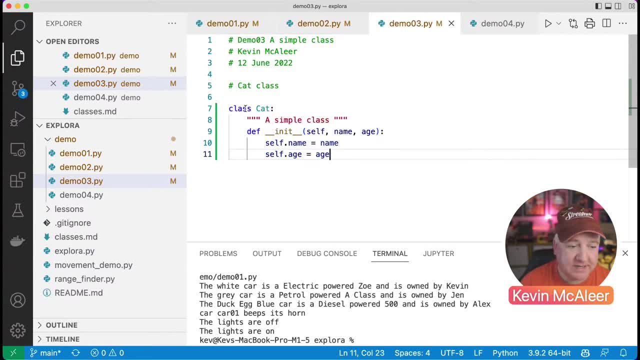 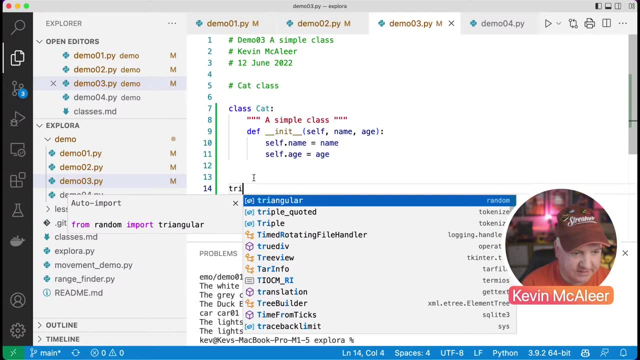 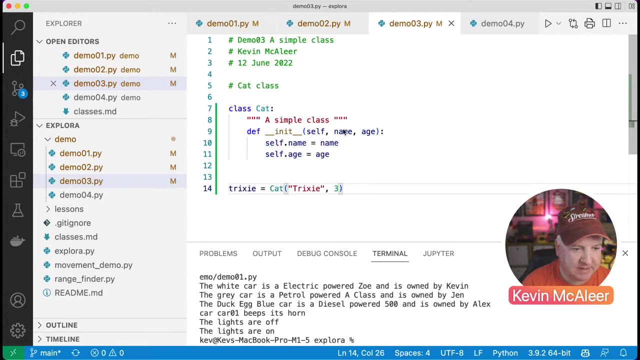 there. so this is a simple class. it's done that underneath the um, the class name. so if we come down the very bottom of our code and let's just type um- i don't know tricksy- which is the name of one of our cats, equals cat and let's just give it a name which is expecting there and an age, and it can do. 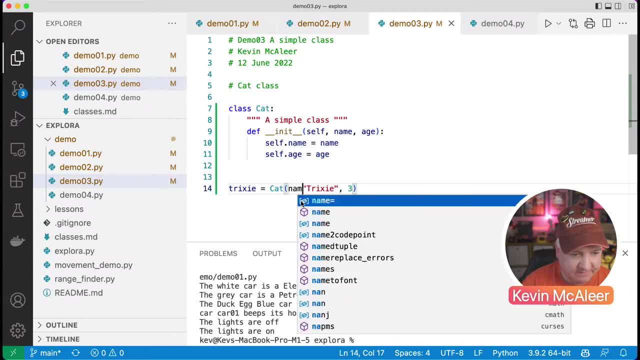 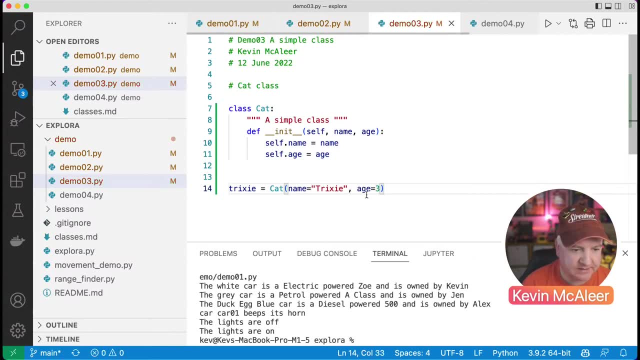 this with positions, or you can actually say what the variable name is, that you want it to be equal to. so you can say: name equals that and age equals that, and that also means if you're not using positional, as in, the first thing it's expecting is the name and the second is the age. 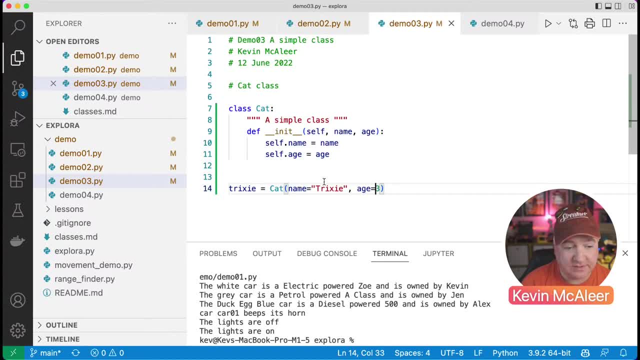 if you actually call out the um, the variable, the parameter that you're actually changing, you can put them in a different order. you could have age first and then. so we could do that. we could say: age equals, i think, trixie's. how old is she? about 16 or something. let's get rid of that bit there. 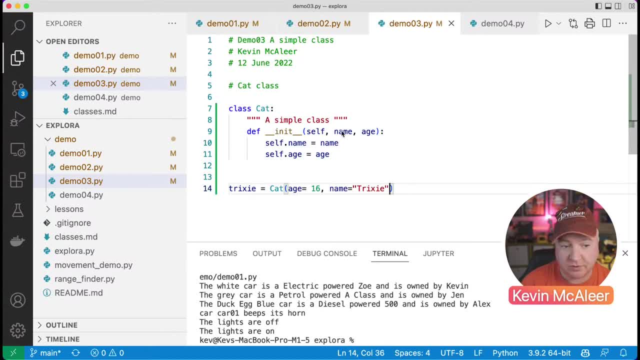 so we can have them in the kind of wrong order and that's fine. that's valid because we're using the name. okay, so that's the first thing we can do. we're going to. we're going to develop this a bit further. so what is this double underscore in it? 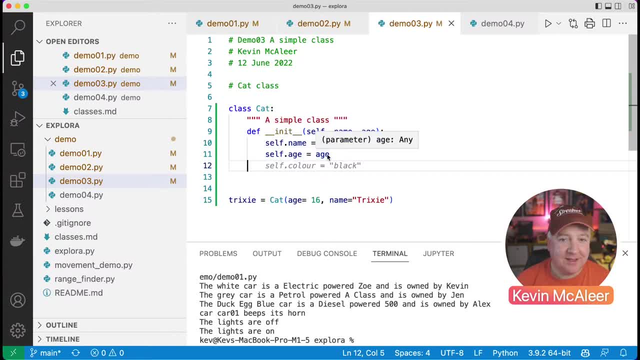 thing. so when we create a class, we say that a class is constructed. so the very first time we create a class we're going to use it, such as here: so trixie is a cat- the very first thing it will do is run this initialization block. we'll call that the constructor. you can also have a destructor at. 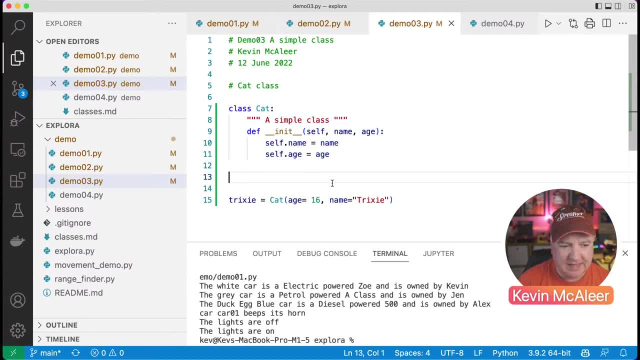 the very end when you get rid of it. but in python we don't tend to get rid of our objects. we can just use them and then forget about them. but you can have something that if you um don't need any more, it goes out of sight. 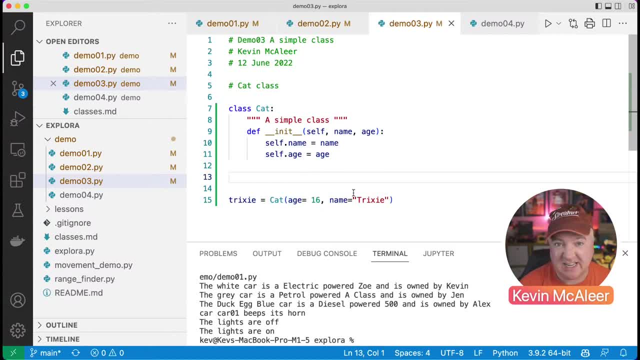 scope, for example, where you're not using any more, it can run like a de-initialization. but for now we just need to know. this is a new thing. it's got the double underscore. that means it's kind of a special internal python um function name and it knows to run that the very 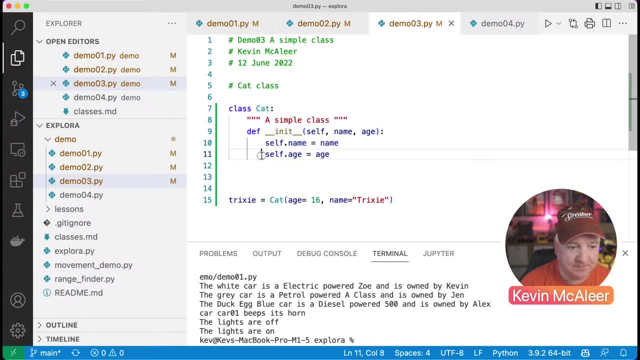 first time the cat class is being used, okay, so what we're going to do now is have another one, which is- i notice how these are slightly indented from our class name- and we're going to have um info. i'm impressed it's doing meow there. i'm just going to have the word self. we'll get onto what. 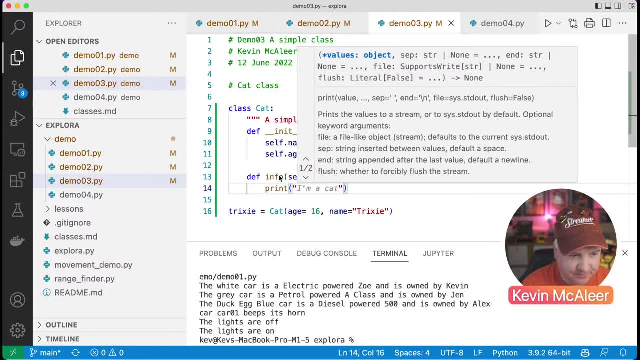 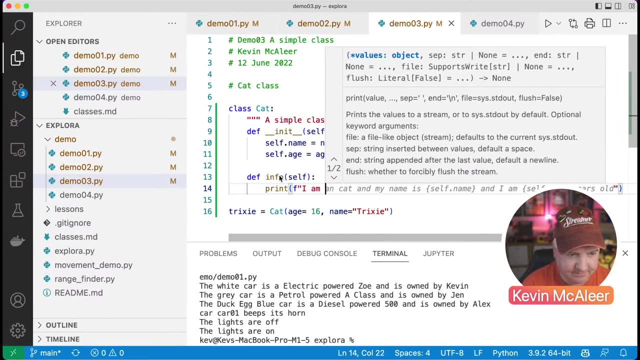 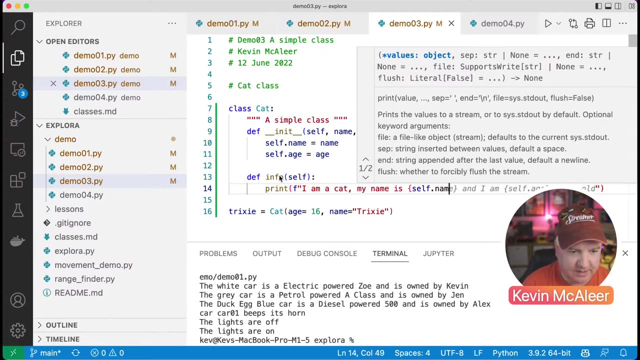 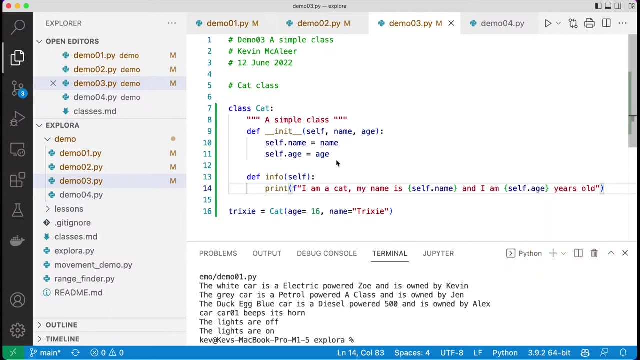 self means in a minute, and then we're going to print something which says i'm going to use our f strings once again. so i am a cat, i am a cat, my name is selfname, and look at that, it's even even typing what i wanted to type there. so i just hide out the way. a second: 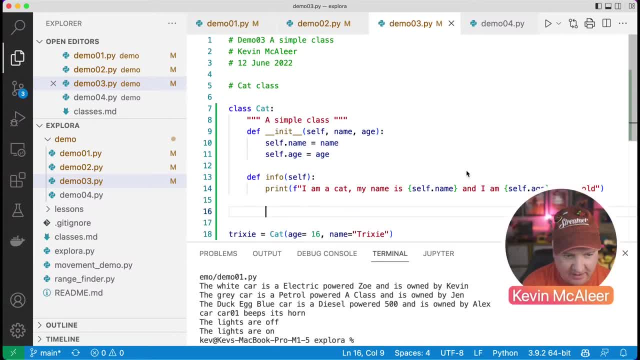 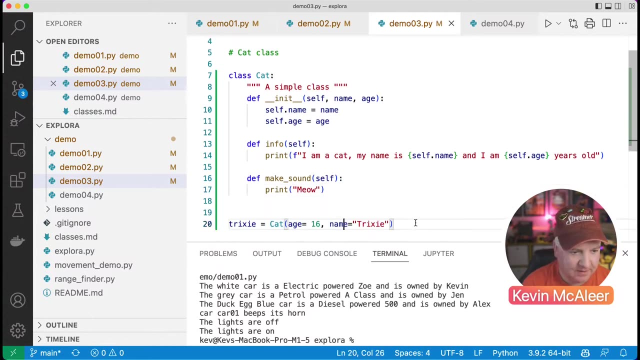 you can see that i am so many years old, right? and then the last thing we're going to have is make sound and print me out. there we go: perfect, perfect, okay. so we've got five cats in our household. so we have, uh, trixie, who's the oldest? 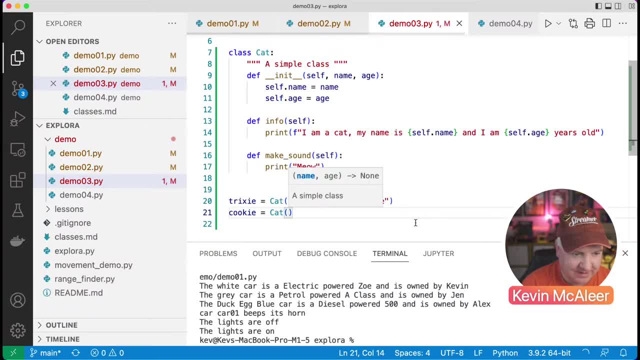 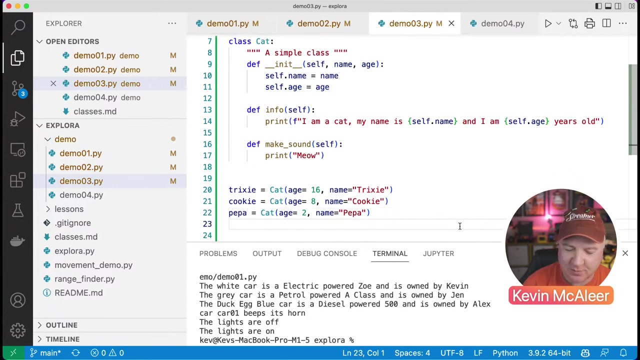 then we have cookie. so cookie. how old is cookie? do we think eight? so age equals eight and the name is cookie. we have who's next? pepper? oops, let's do a lowercase. just naming conventions. she's a cat, age two, pepper. it's almost as if it heard you, then that's creepy. then we have bella. that's a cat. how old is bella? 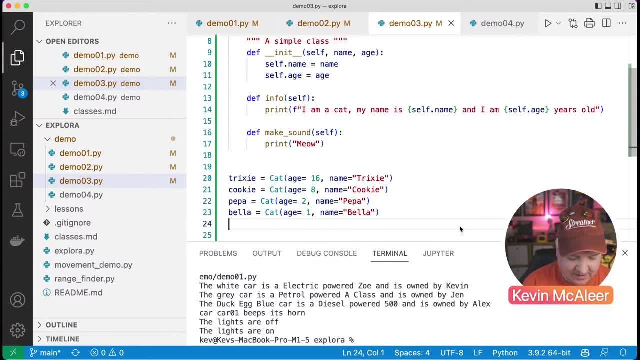 creepy. it knows that vela is one we have. i forget my own cat's name now, tigger, of course. tigger, our latest cat, and she's eight, nine months. it's nine months old, so let's do 0.6 of a year old, okay, um, actually, what i'll do, just to be. 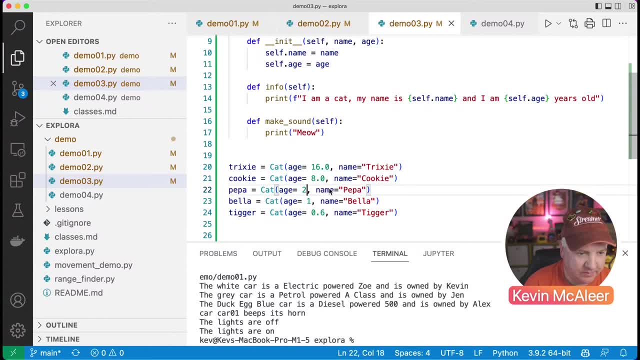 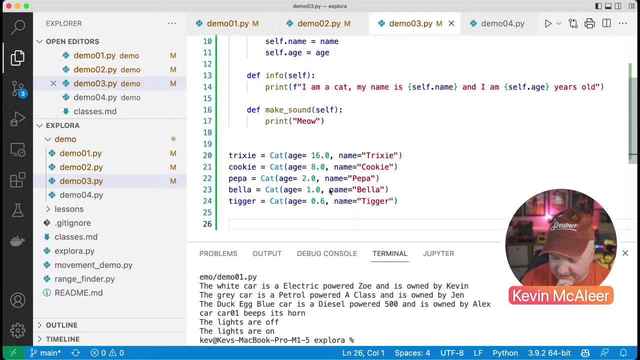 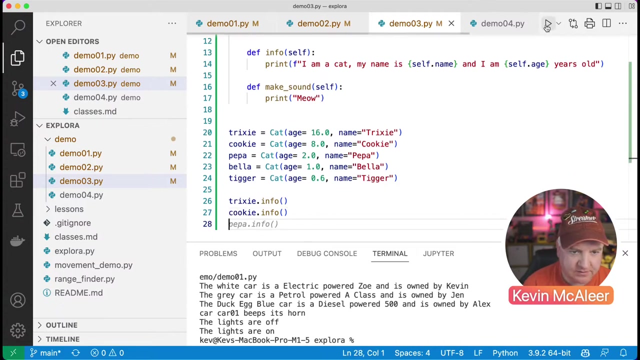 consistent. i'm going to make all these floating point numbers. so if you put point after it, it knows it's then a floating point number, otherwise it'll treat it as an integer. i want them all to be the same right? so if i now say cat tricksy, dot info and i then do cookieinfo, let's just run that. 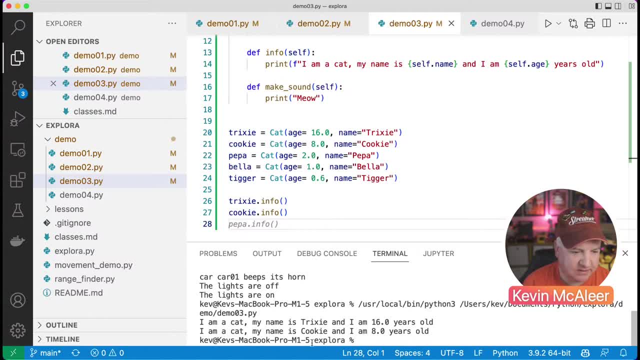 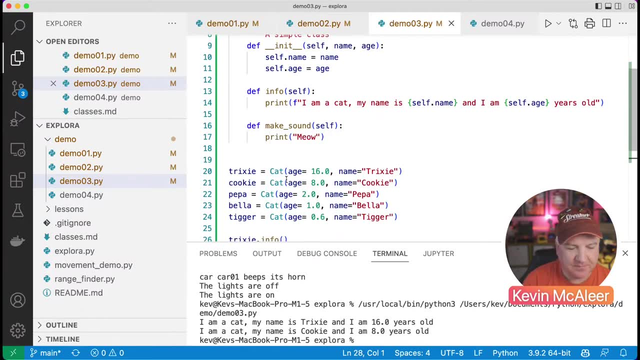 code. so i'm a cat, my name is trixie and i'm 16 years old. i'm a cat, my name is cookie and i'm eight years old. so you can see there, we've defined our classes. our class is simply just this small piece of code. we've defined our classes. our class is simply just this small piece of code. 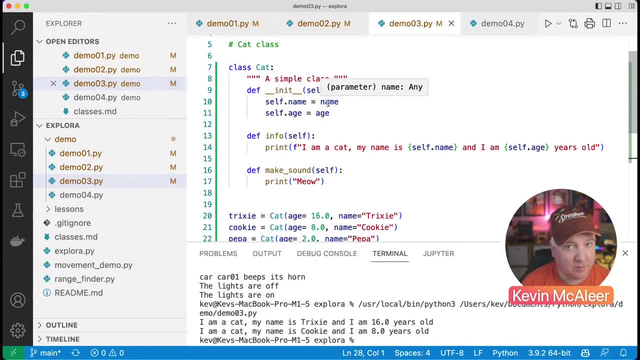 here. it's got two variables, two properties, and it's got two methods, two functions, if you like, within it. now this self variable, which we saw being used throughout here, means whatever this particular instance is. so you can see, trixie is the first instance that we've got the, the value of 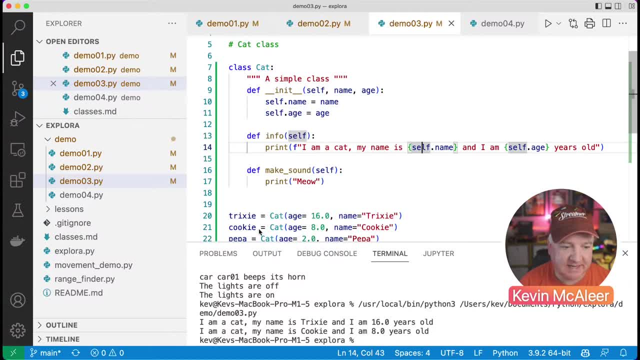 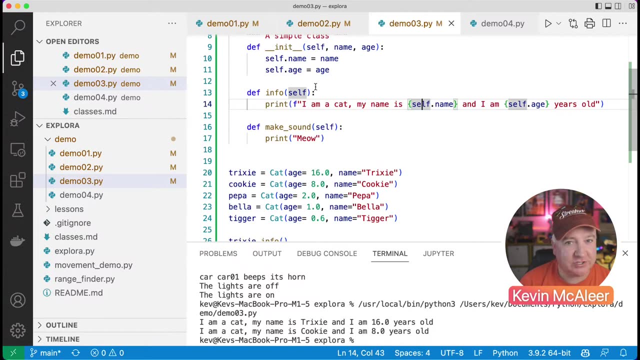 the name, which is going to be trixie, is going to be different from the second instance of this class. so, so that python understands which cat we're referring to, which class we're referring to, we have this thing called self, and it means the one that you are. so that's what that self means. it means refer to yourself. 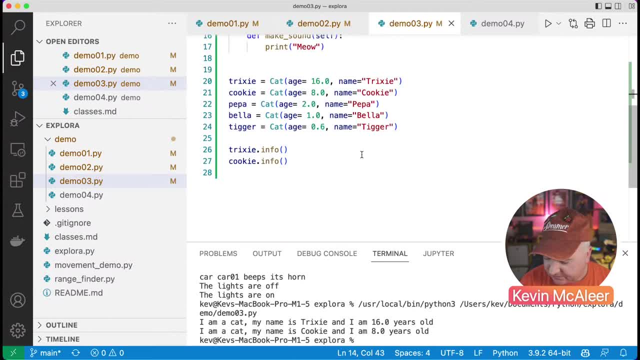 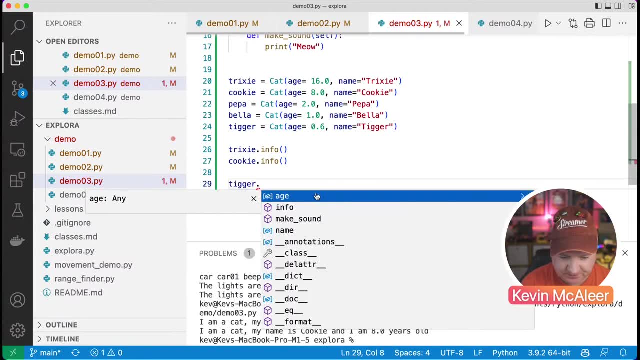 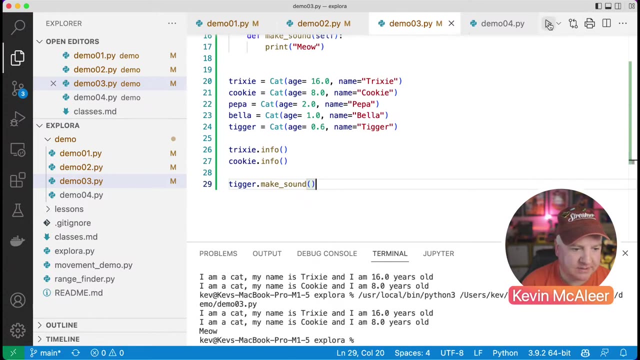 and whatever is stored within those variables. so that's that. oh, we can also make. make um, tickers are a noisy cat, so let's make a sound like so. so if we do that and press return, you can see. you know, we can use this for a number of things. so let's take a look at this class. 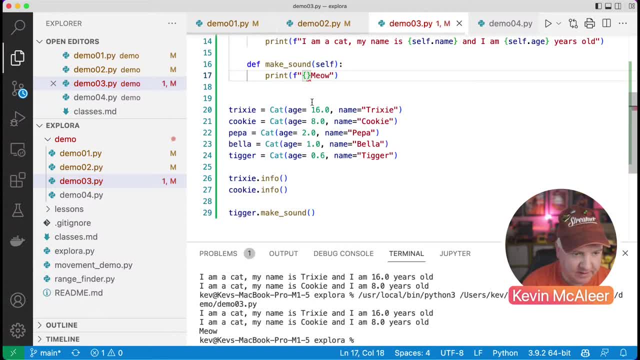 um, i told you we're going to make a crop, so here we've just set it up to say, um, so yeah, i could say: And Trail a Card may contents we've got. um, um, uh, we could also make our class. we can type: it's not my class. it says: yeah, i'm not sure, but you can do this, and oh, and, we could. 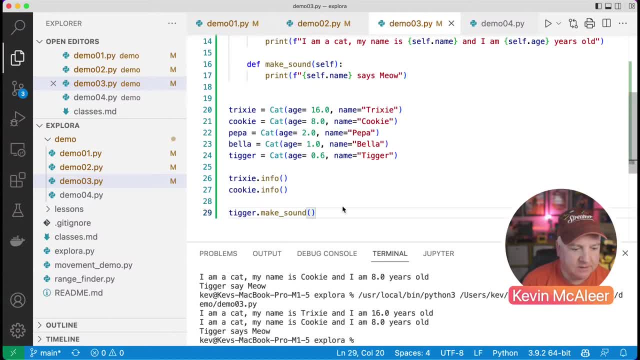 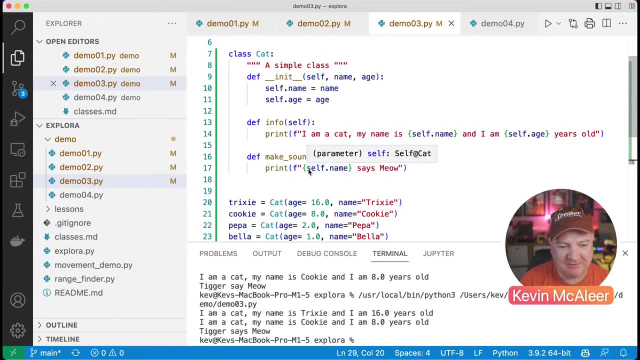 um switched to extra table, so now we can just run a card here. put your task on mouse and click choose. reads a lot more like english, um. the other way to do this is by having sort of um percentage variables, and then you have to- at the end of the thing you have to say what those variables was. 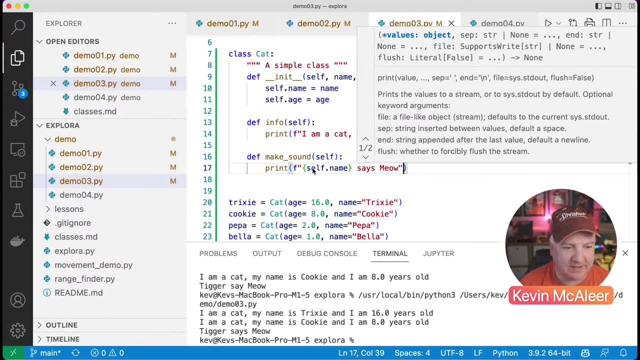 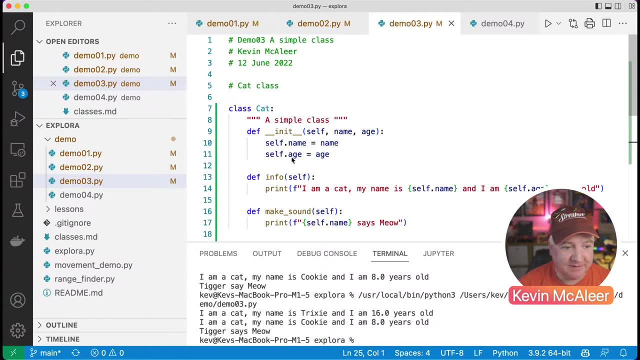 it's just horrible. this is a much more understandable way. it's just those brackets. the first time you see anything. what's that? what does that actually mean? so this is a real class we have. we've defined our class. we've defined an initialization, a constructor, we've set some. 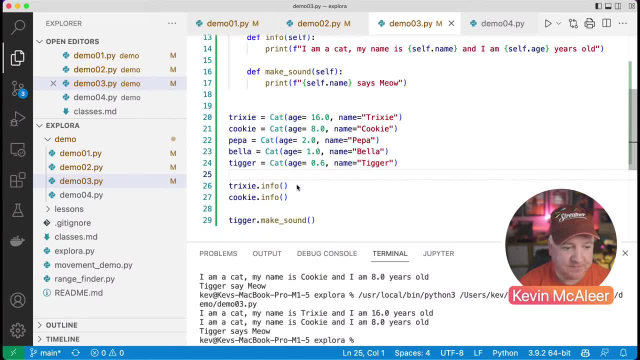 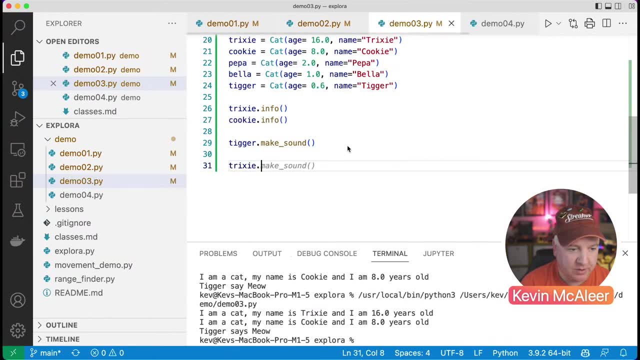 internal properties and then we've got some functions and then down here when we've actually started playing with this. so let's have a look at another thing. if i go to tricksyname, i want to show you if we do. if i type n for that, you can see there it's got this little symbol here. 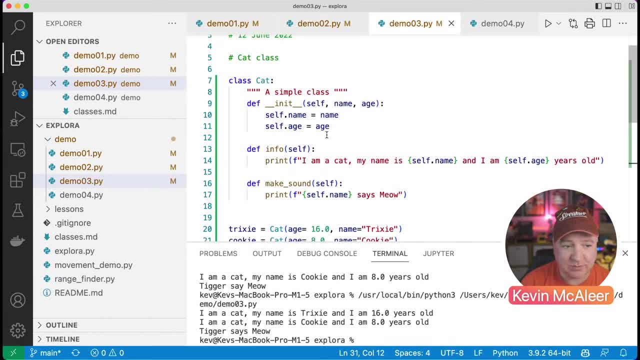 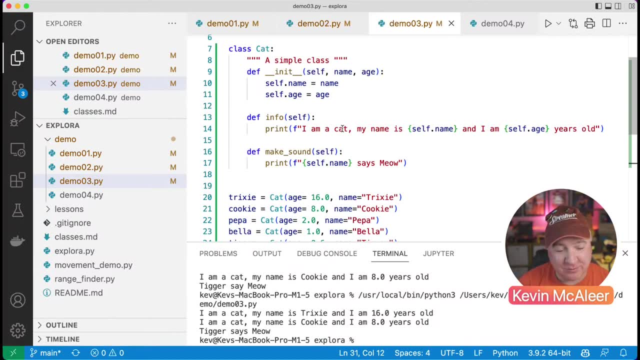 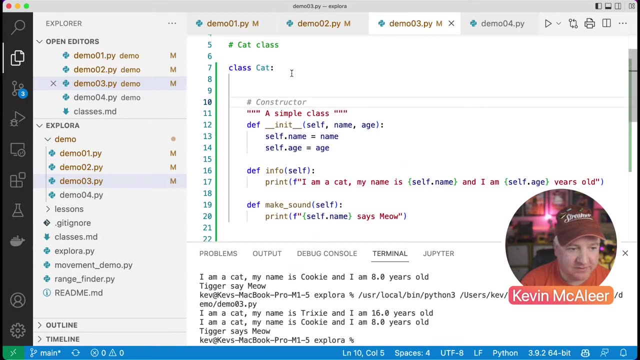 and it says name and it's any any is because we haven't actually defined what that is. we haven't. it doesn't know what. if that should be a string, an integer, a floating point, number, um, it doesn't know what it will be be anything, because we haven't defined up here what that is. if i actually come to the very top, 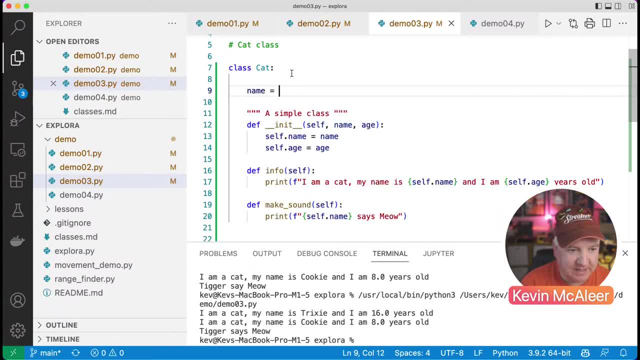 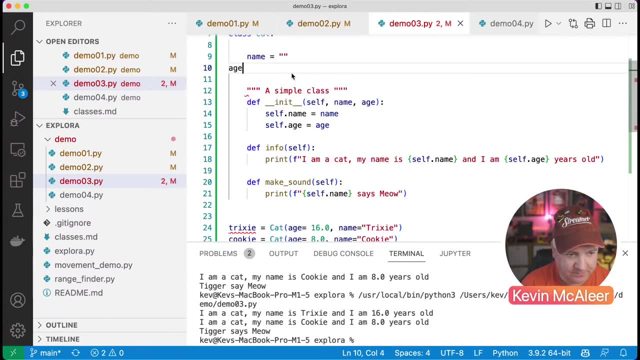 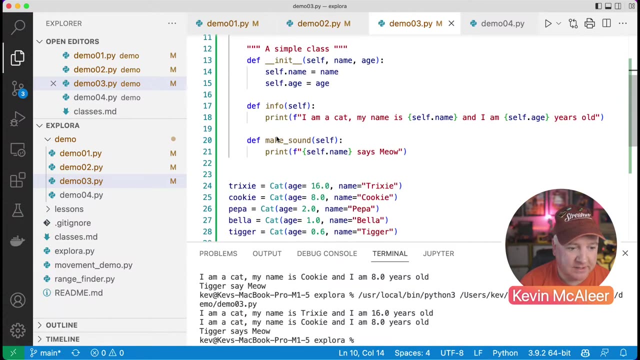 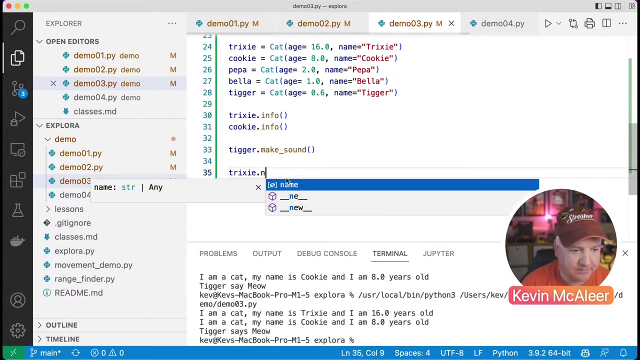 of the class here before the constructor, and i say name equals, and then do that, and then i do age, oops, and i do equals 0.0, for example. i've given them some default values and if i come down here now and i'd go back to name, i start typing it in again. now you can see, now it now knows that. 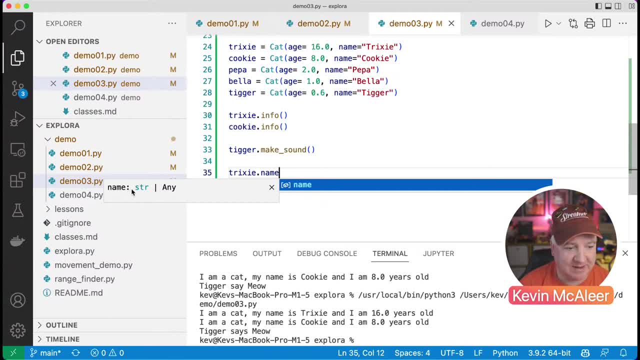 that should be a string, because we've defined further up that that's going to be a string type. but you can actually still pass it any value, so we can put whatever we like there. but you could put like a number and if we run that, let's see what actually happens. it's gonna. 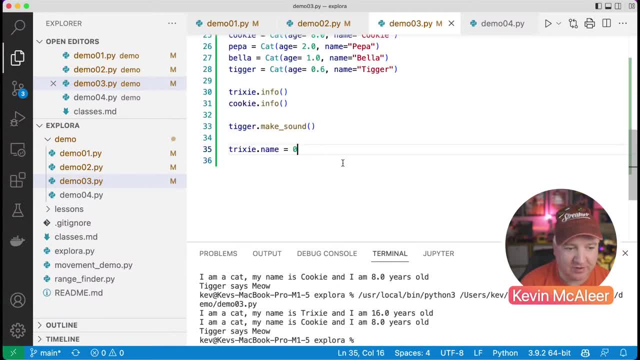 it's gonna run fine. it doesn't care that you've assigned that number. it's not treating that in any way, because we haven't got any protection around that. we've just simply set it as being tricksyname. so there we go. well, i think that's everything i need to cover off on. 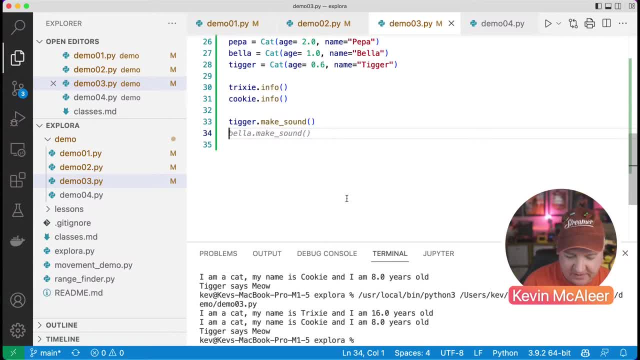 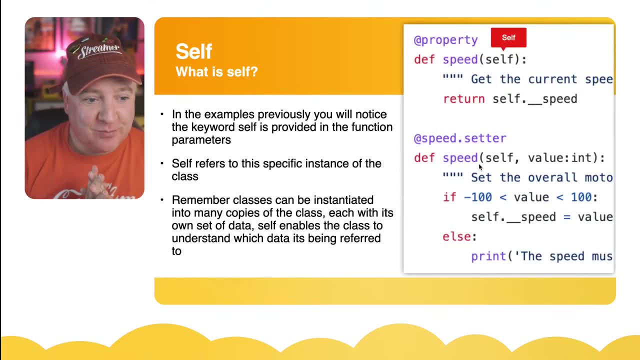 that particular one. yes, because we're going to get into, uh, some more in a second. so let's get back to our keynote and let's carry on so. self- we looked at that a minute ago, so in the previous example we noticed this word self, which is a it's provided in the function parameter. now in our 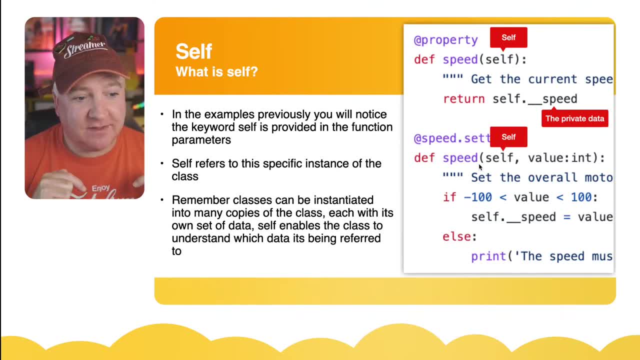 method parameter self refers to that specific instance that is being used at the time. so trixie or bella or cookie pepper are the other one tigger. so remember, classes can be in instantiated many, many times. we're going to have many, many copies of the class being used in objects and each one has its own set. 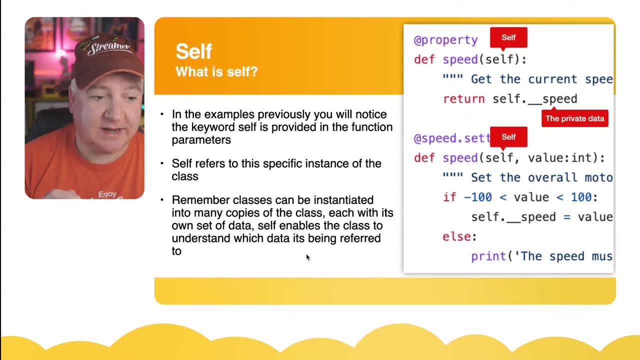 of data and the self enables that class to identify which piece of data it's being referred to. so, in there, self means whichever particular one you're you're currently using, and the double underscore is a way of protecting it by making it private. so we're going to create that in a second. 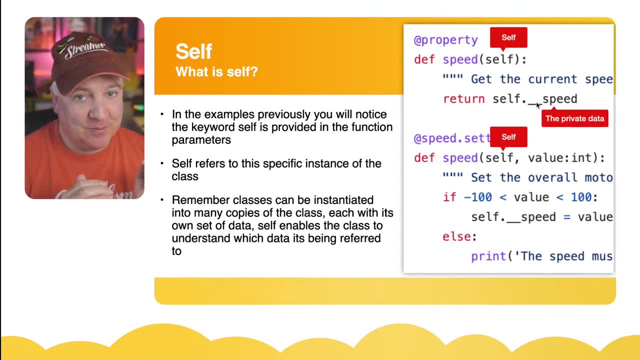 and i'm going to show you how to create some clever protection around your, your properties. we saw just a second ago i could create name, but i could assign that number. we don't want to be able to do that in every single case. sometimes we're going to protect what people 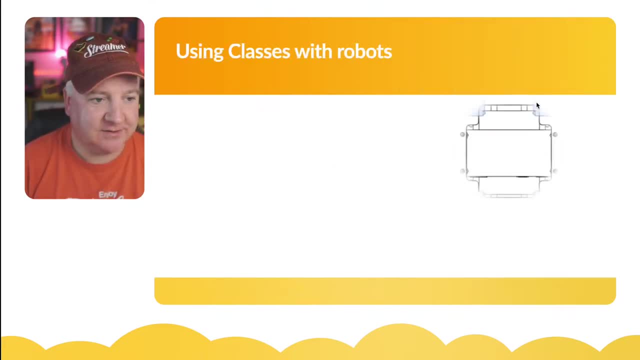 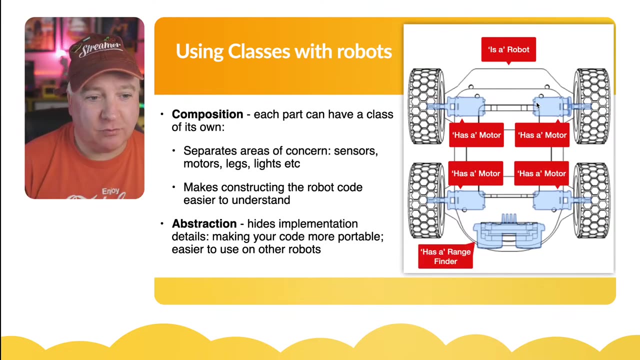 can change, so we're going to have a look at that in a second. i'm using classes with robots, so think about what you've just learned so far: composition. you can say each part of our robot can have its own class. so we can have a motor class, we can have a range finder class, we can have a legs class in. 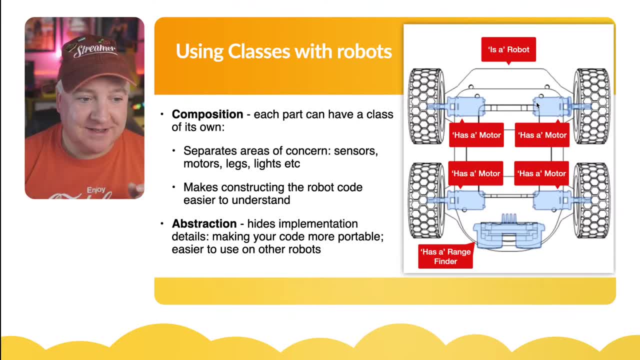 fact, when i created my uh, open cat, my pico cat, i modeled each section of leg because it was essentially just a servo motor. but i had like upper leg foot, um, i had like shoulder that kind of thing, and then i would like left leg and that would be composed of the foot and the leg, so i could have 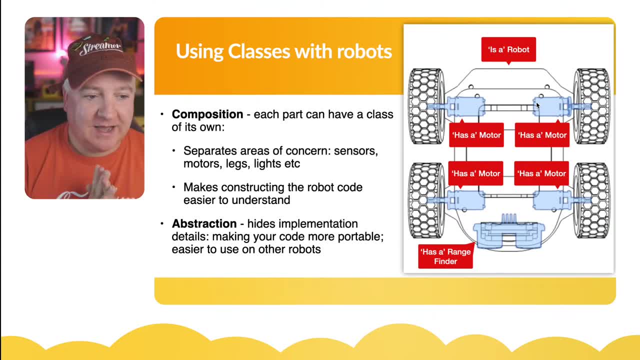 i could have hierarchies of classes within my robot and it makes constructing the robot code a lot easier to understand and a lot easier to debug when you've got problems and the abstraction of the robot. so i could write some code here, um, in python, and i can actually lift that and put that. 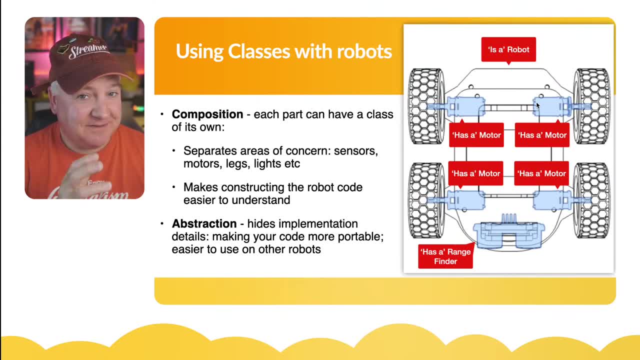 into micropython, as long as the actual end piece of code that does the. you know, the turning of the motor is just tweaked for that particular implementation, but everything else, all the other logic, will work just fine. so if you like what i do and you want to see more of this, um, 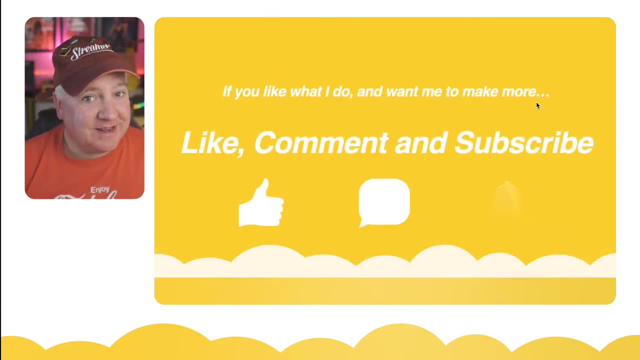 give me a like on this particular video. let me know that you're enjoying this. drop me a comment as well. tell me what you think about this video and i'll see you in the next video. bye, bye. if you've used this before, if this is um something that's new to you, whether you're going to use this. 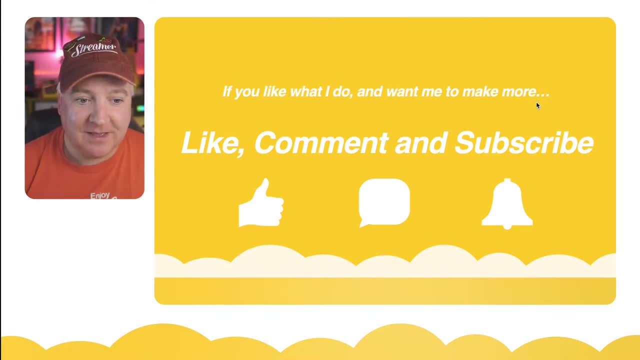 in micropython, circuit python or regular python and also subscribe to the channel if you've not done that already. that really helps the channel grow and become more popular. and we did breach the 7 000 um bracket of follow of subscribers, and most recently, on twitter as well, we got over a thousand. 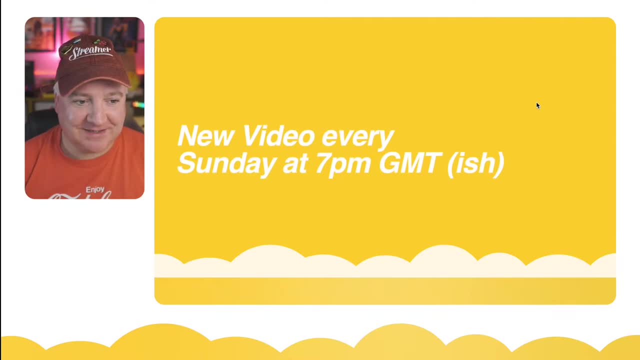 followers on twitter and i think we've got almost a thousand and a half there, so that's pretty cool. i do go live every single sunday and that's seven o'clock gmt um. so if you want to join live and join in the conversation after the, 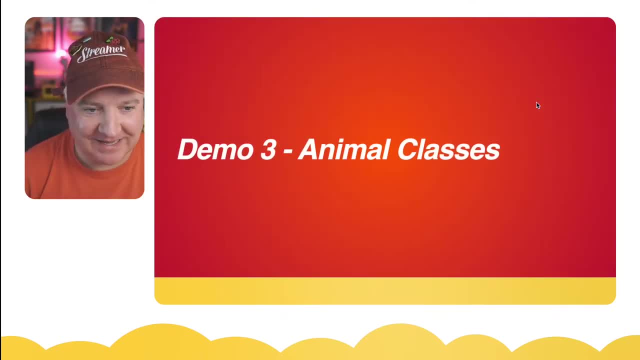 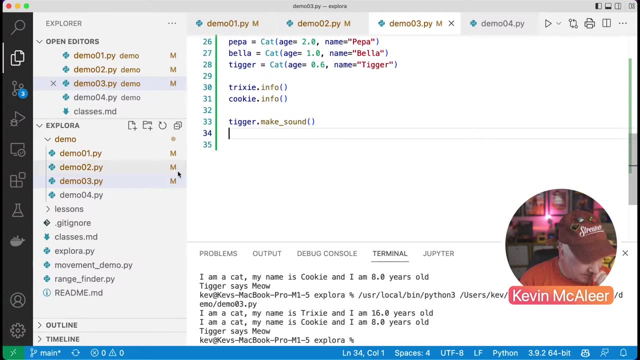 demonstrations, then you can do that too. right, let's go over to our animal classes. this is pretty cool, so let me get back over to uh, visual studio and let me find the next piece, which is: should we go for the car one off the animals one? i think we'll go for the um. go for the car one first. 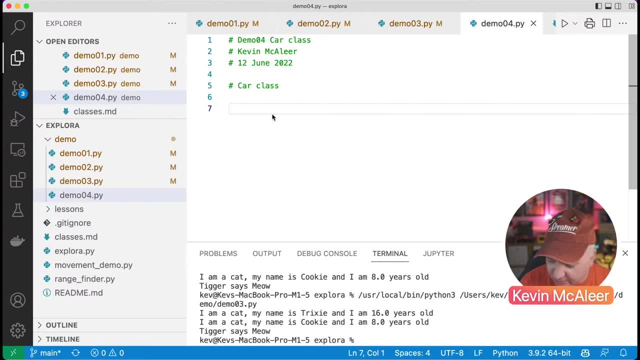 right. it said: i'm always go for car first, right? so what we want to do is we want to create a new class, which is car, and we're going to create um some variables which are for properties. i can't type um, so we're going to create um color. 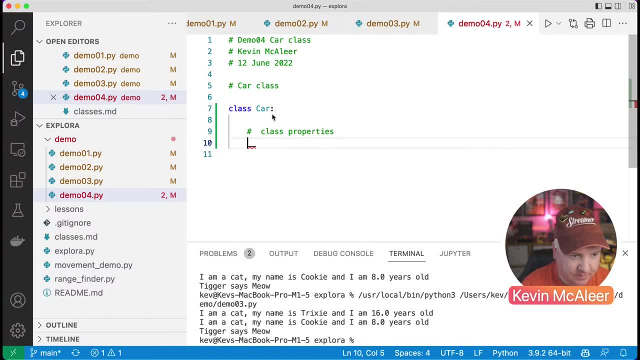 let's do owner first. let's do double underscore owner. i'm going to say no one to begin with, because no one actually owns a car to begin with. the color is going to be uh yeah, black's fine. then we're going to have model unknown. we're going to have fuel type. 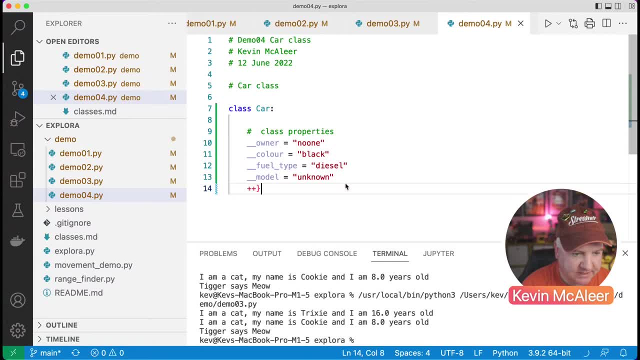 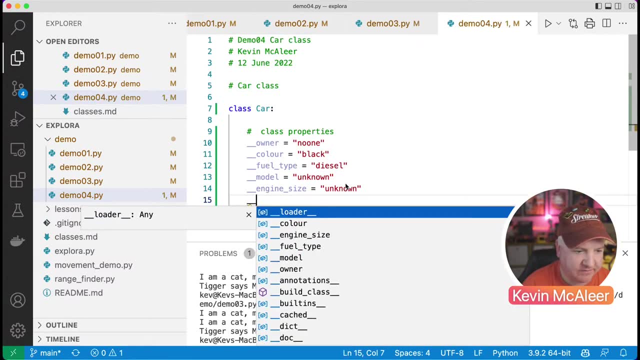 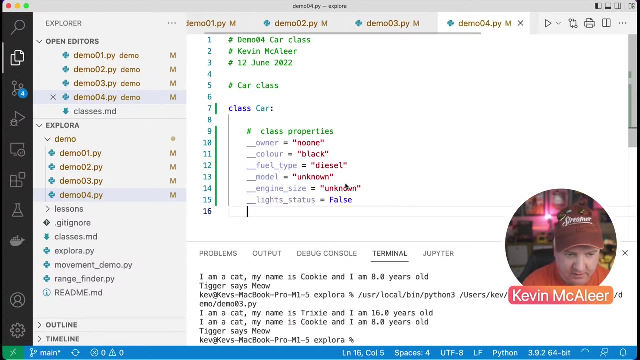 diesel's fine to begin with. what else do we have? engine size, and we also have the light status. remember we created an extra variable after we've done all that for the lights status. lights status: i'll set that to false begin with. the lights are off and we've got model there as well, right? 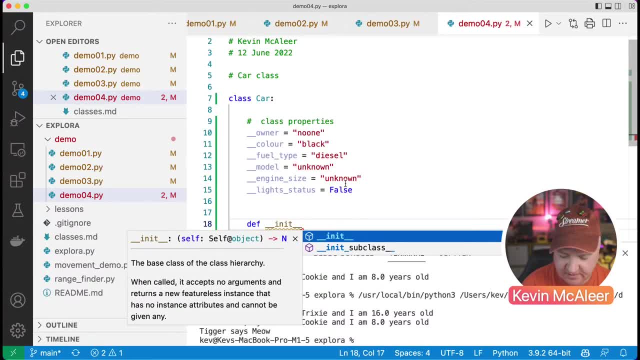 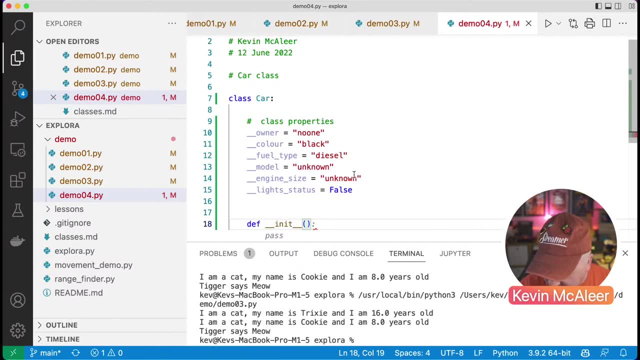 so then, the first thing we need to do is create that initialization thing, and what i'm also going to do on this one, um, i'm not going to do on this one, i'll do it slightly later on, right? so we're going to do self, first of all, because we need to make this initialize. 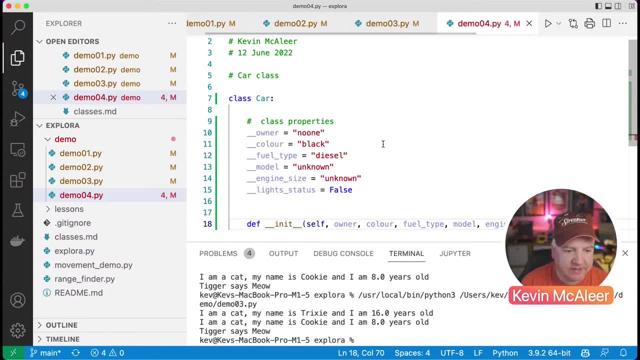 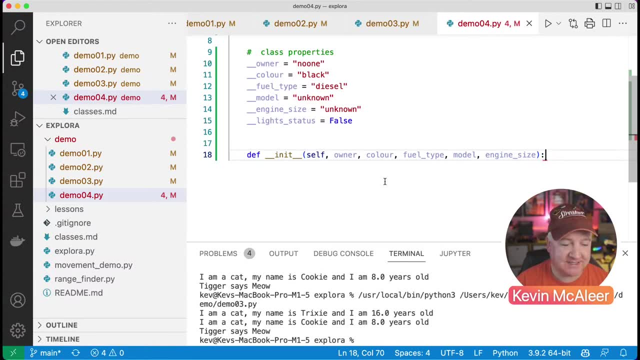 the current one. now, i could just do this and just say owner, color, fuel type, model and engine size. and what that means is, when you create a new class, a new object of this class, you have to provide all of those things. now, sometimes you might not want to be, you might not want to be. 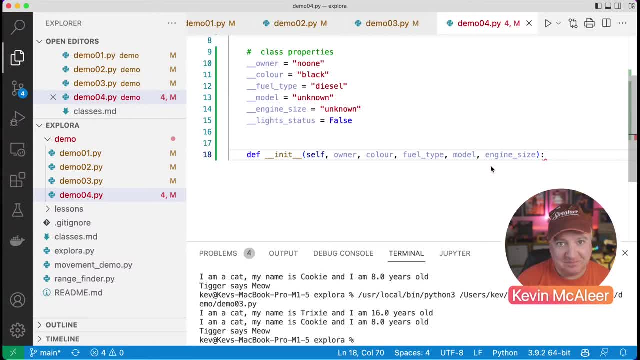 or you might not want to have to create all these things um, or have them ready when you create the class. you might want to provide them slightly afterwards, so what we can do is make them optional. the way that we do that is we say equals none, and we can do that after each of these. just 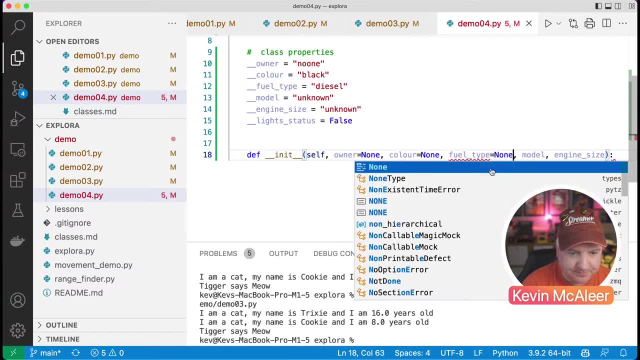 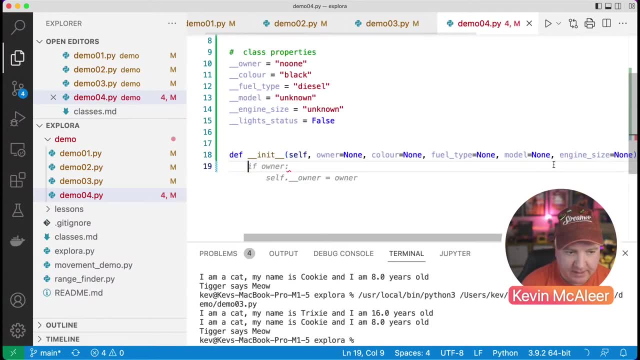 say, each of these can be optional, so model equals none, then engine size equals, not. okay. and then what we can then do is we can then just have our create our new car doc string and let's say, if owner, so if this variable here owner, if that's none, now we want to basically create a default value for that, but if it does have a value, 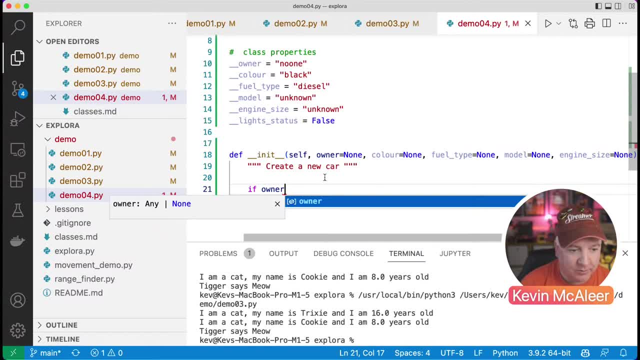 so if owner is passed in, so say kev is passed in there, and we'd have to say: is owner equal is true? we could write that. but you can also just do something a bit more advanced. you can just say: if owner, so that is it assumes it's true, so if owner. and then we can say our double underscore owner. 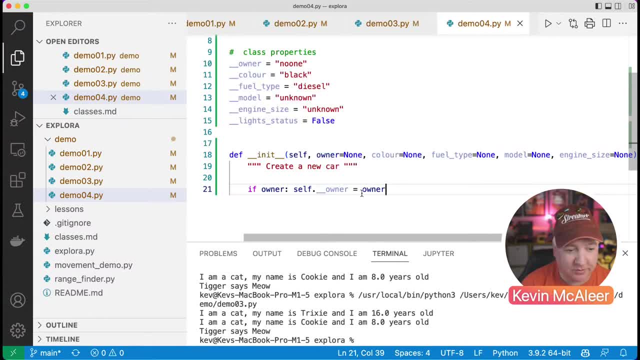 which we have to refer to using the self thing. so self dot double underscore owner equals whatever we pass in there, and then otherwise we can say, um, it's no one, for example. we could do that. i'm not doing that because i've already actually set those up here, so that's fine, so we don't need. 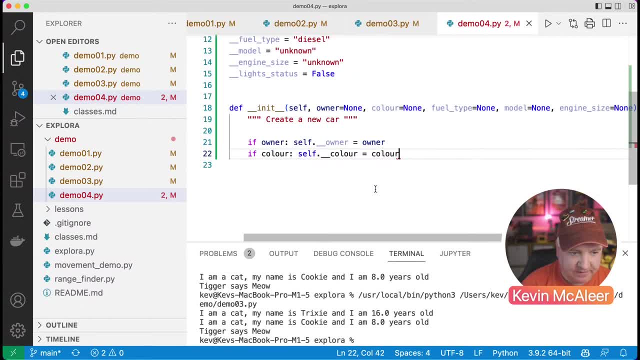 to have um um an else name each of these, so we can basically just do this for all of these. so, um, fuel type. i'm just waiting a lot to guess everything for me. model model, if engine size, and it's the one more. any size, model, fuel type, color. oh no, that's all good. 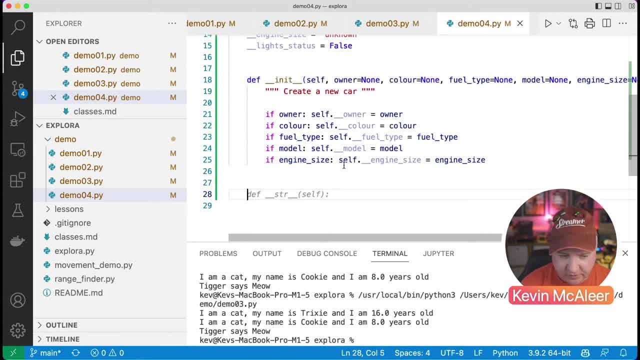 right now we're going to do something new. now we're going to, we're going to create a property using that decorator function. so we say app property and then we say the name of the thing that we want to be the property. so in this case, we want it to be um owner. we need self in there, because anything that's inside. 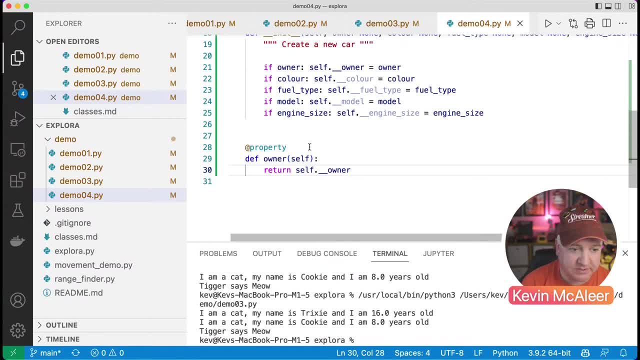 a class needs to have self as the first variable so that it has that link back to which particular it's actually a memory address. that's what it's actually providing there, and it does this kind of behind the scenes and it basically just says this is the block of memory that's got. 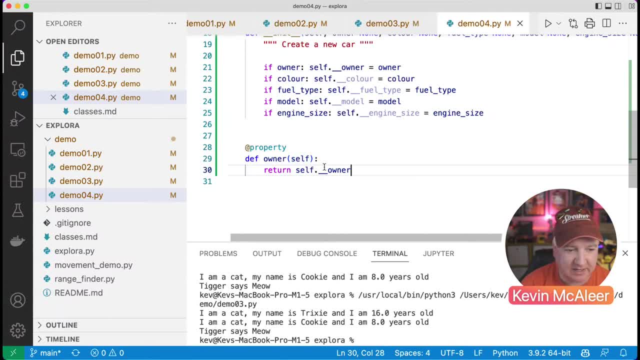 all the variables in for this particular class. so that's really what self is doing. it's like a pointer to some memory and what we're really doing with this one. this is going to be a getter, so what we need to have on there is just those three things and then to say: gets the value. 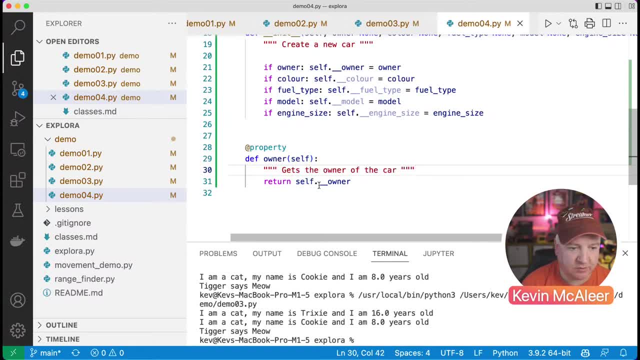 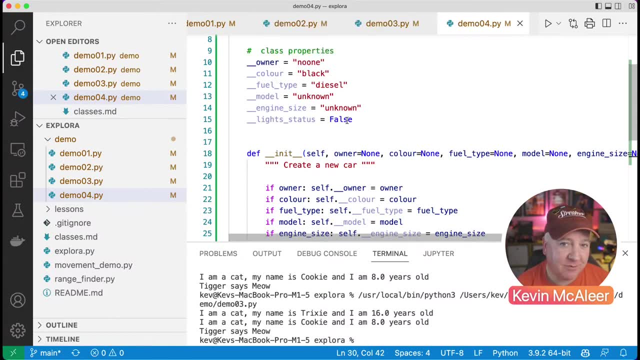 gets the owner of the car perfect, so returns self dot double underscore: owner. so whatever is in that variable up there now the other cool thing with visual studio is it will tell you if your variables are being used or not. so you can actually make your code more efficient. so you can see there. 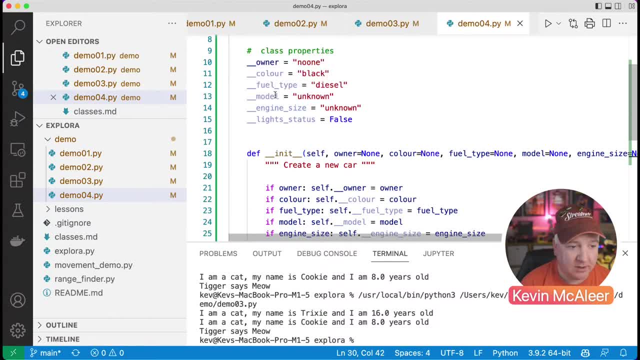 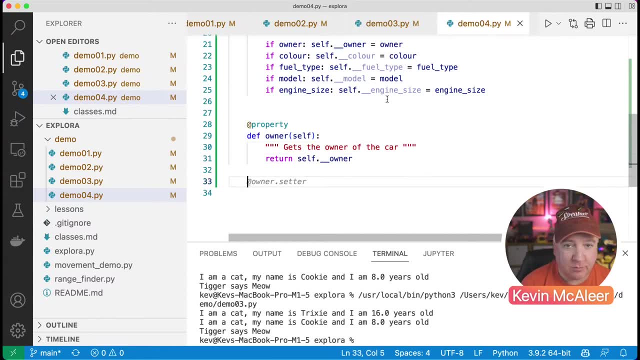 double underscore. color isn't used anywhere in our code, yet same for all the rest of them, whereas owner is actually being used because we've used it here. so that's a really cool way of seeing whether your variables are actually being used and whether you can actually get rid of that code or. 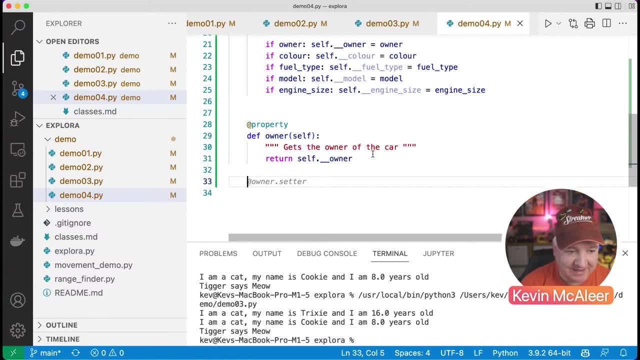 not, so the next thing we need to do is a setter. it's already guessing there. this is co-pilot guessing for what code we need to have. so def, def, owner- and i don't like to use the actual name that, i like to use value instead it just i think it makes it. 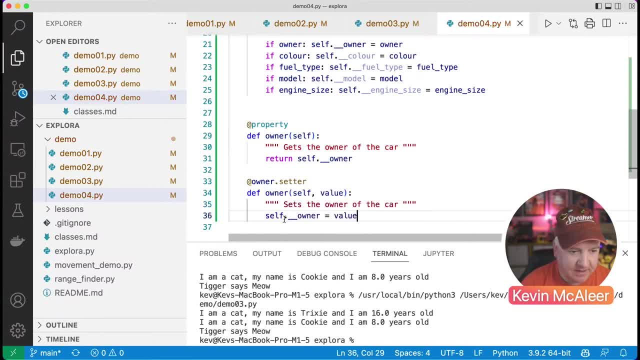 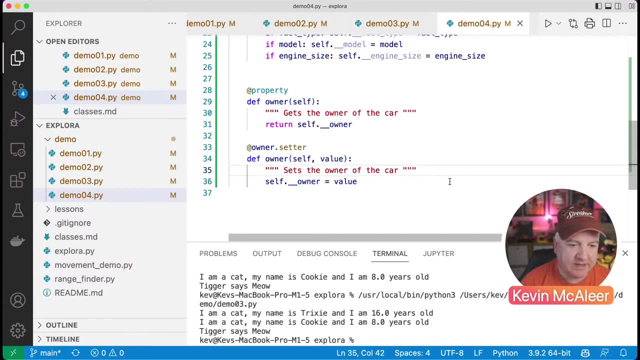 more understandable for me. so sets the owner of the car and self dot double underscore: owner equals value. so whatever we pass in there now, we could make an extra piece of logic in here that says like: um, so say my brother stephen, so if value equals stephen, something like that. 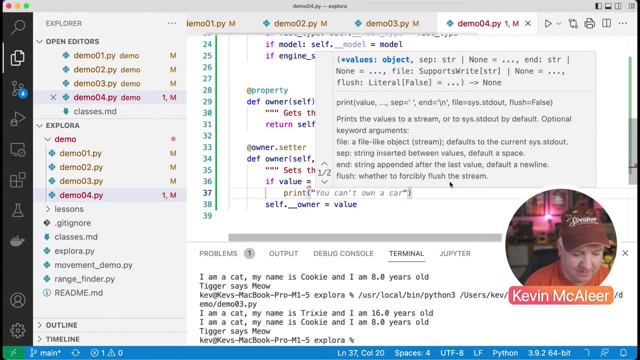 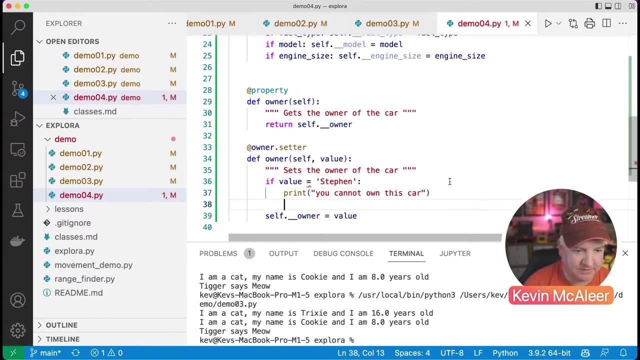 uh, then print such as that and then we could just say else like that: um, we need double equals because comparison, instead of saying equals, we could also say in, which is another cool thing you can do in python. you can basically just pass it a list of things. so we could have stephen john. um, i don't know. 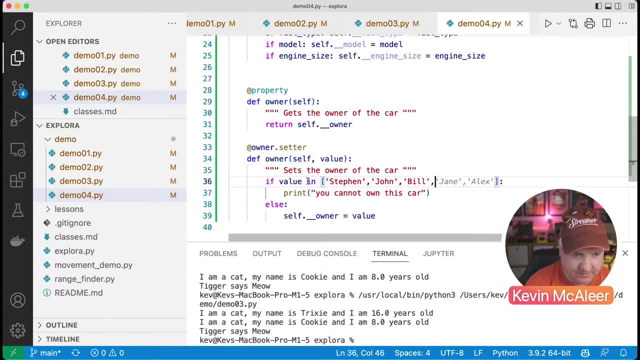 if you signed in here, but i think phil's right off but it's called alpha dot. god, i don't know. um, think about it. haha, i've looked at a bunch of värden and oly instead of prep. it looks perhaps on just yours. it's not quite the case exactly, but we can press all of these times. 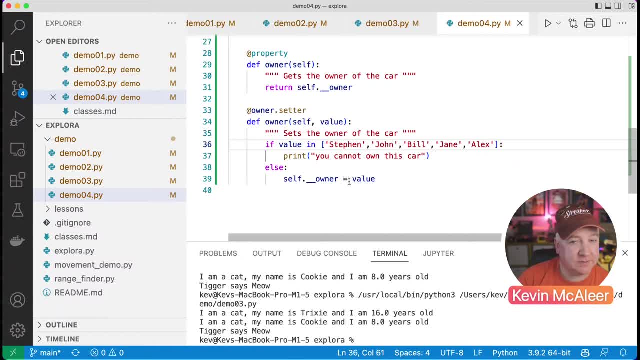 different variables. can we compare hunting courses through epidemiology? but empire book your trade content. andapping that case you'll be surprised to see it's actually pretty good. you know真 z a good для sorta implement this game. you'll баб子 bill, surely, jane and alex? there we go. all those people can't own cars about like onto this now. 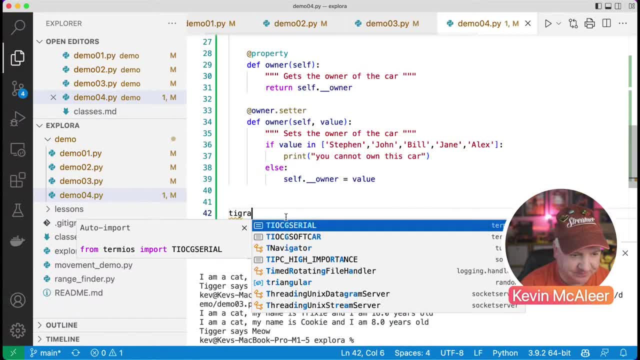 um, so if it's in there, you can't own the car, and it will basically just break out that point. if it's not within that list, then it it'll basically set that value. so this is a way that we can introduceue tigra and let's make that a car, and i'm not going to pass any details, i can just do that, so i can. 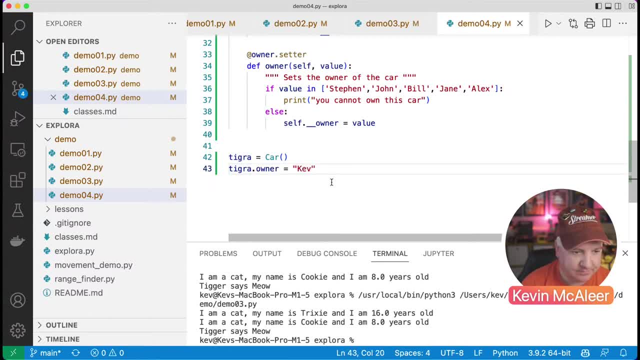 say that the owner of this car is kev, let's run that and it'll not do anything because i've not put any extra code in there yet. but let's try making john the owner of the car. you cannot own this car, so we've got some extra protection in there. look, owner doesn't have brackets, even though 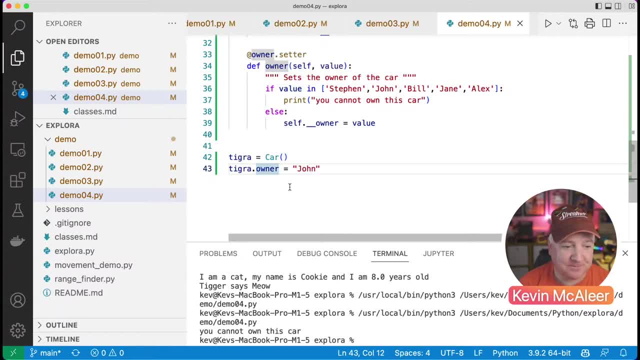 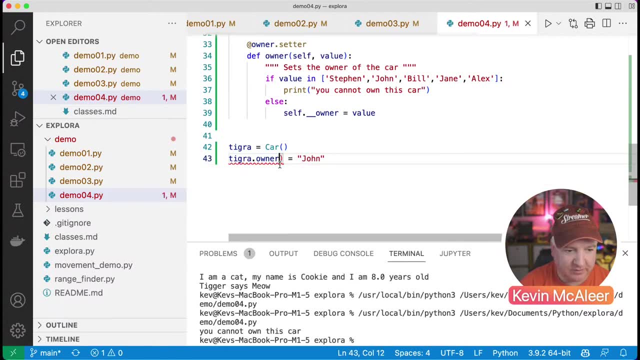 that's a function, because it's treating it as a property and that's what that decorator at the top there does. it means that we don't need to put brackets around that and pass in like the variable. like john, we can just assign it as if it was just a regular variable. that's one of the really cool. 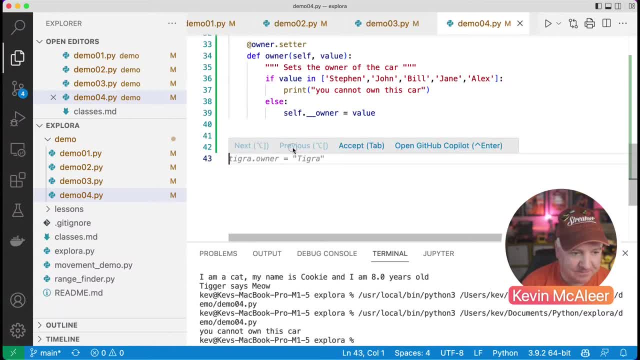 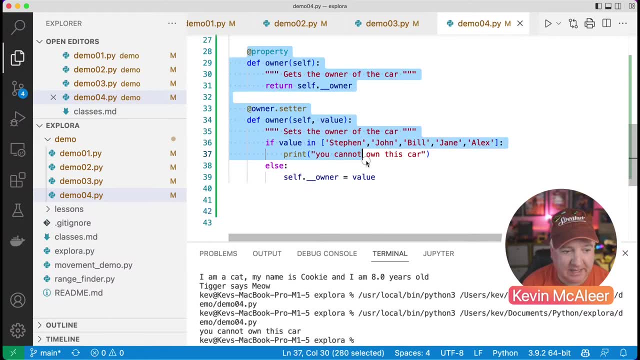 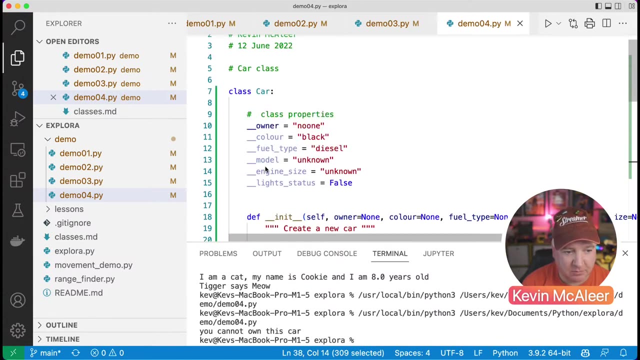 things about classes. so let's just get rid of that and let's have a see if there's anything else what i need to do. so, really, the next part of the code would basically be me replicating properties and setters for each of the variables. internal variables: i've got there color, fuel type, model, engine size and light status. 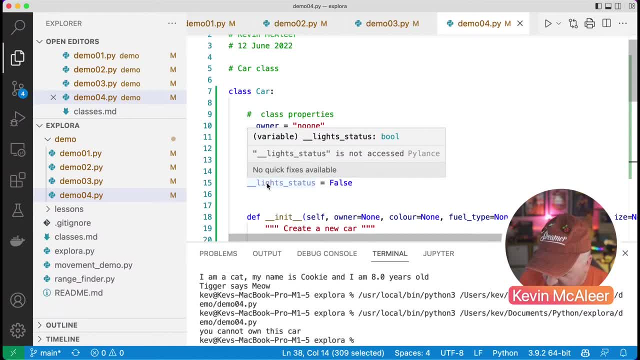 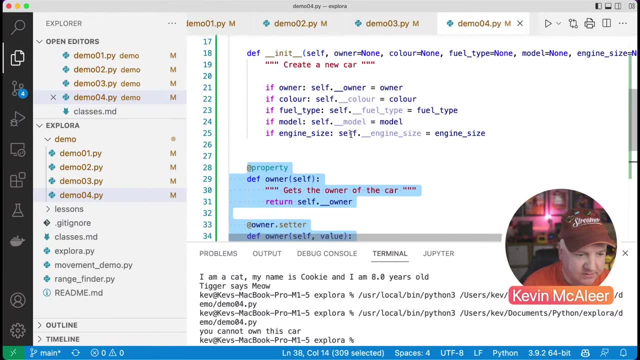 so that would be quite a boring thing for me to type out for you, just looking at time as well. but what we can do is we can have some other functions in there, such as that show details, so we could just create that one at the very bottom there. let's just do. 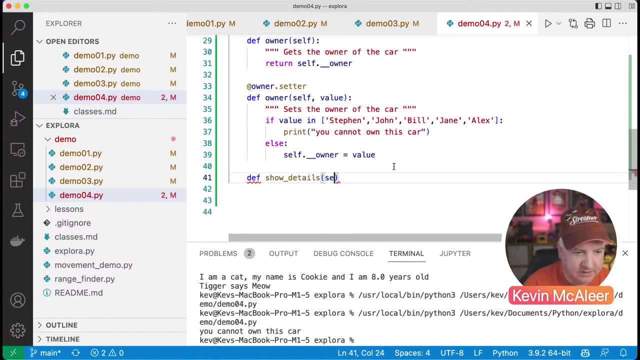 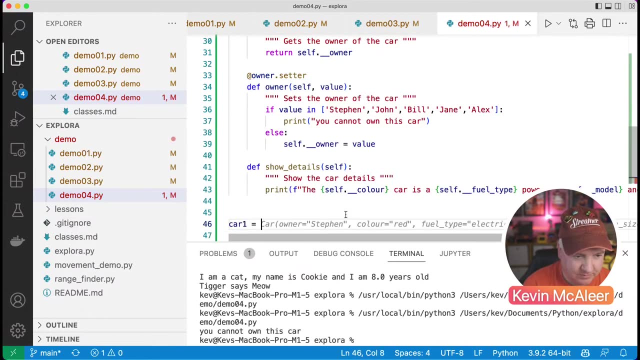 that. so def show details. we can just have self. we don't need to pass anything else in, because we can refer to all those variables that we have already. look, it's even guessed what i want to do there, so let's just run. let's create that car again. so car1 equals car. 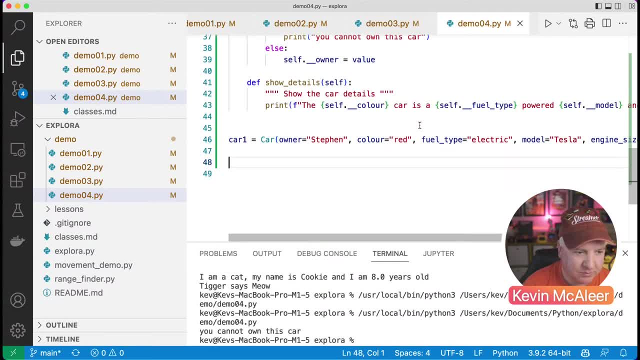 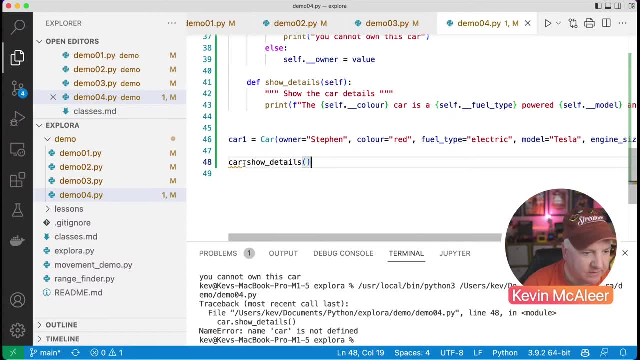 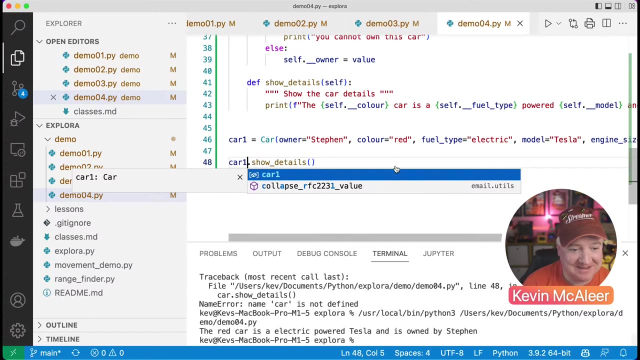 i'll do, and then let's just do car1.show details like: so let's run that. so car is not defined, car one we need there. so the red car is an electric powered tesla. it is all by stephen, apparently. that's cool. so if you're wondering how it's completing all this code and writing it for, 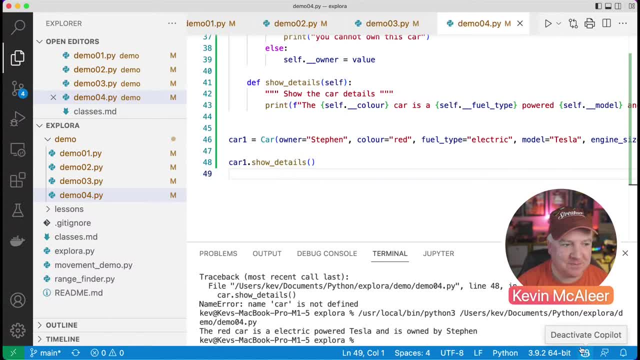 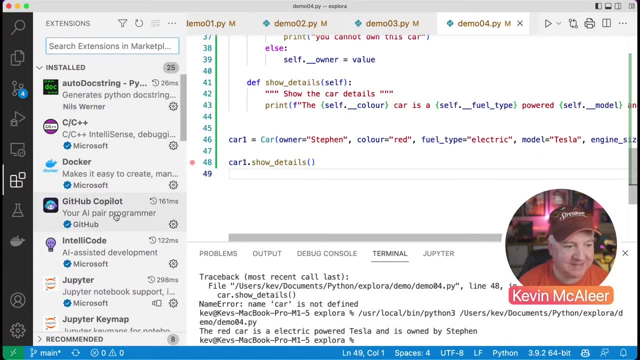 me. this thing down here is called copilot, so there's a new functionality that you can hook into. if i go to the marketplace there and search for github copilot, it's like an ai paired programmer, so there's an ai working in the background trying to guess what it thinks. the next line of code: 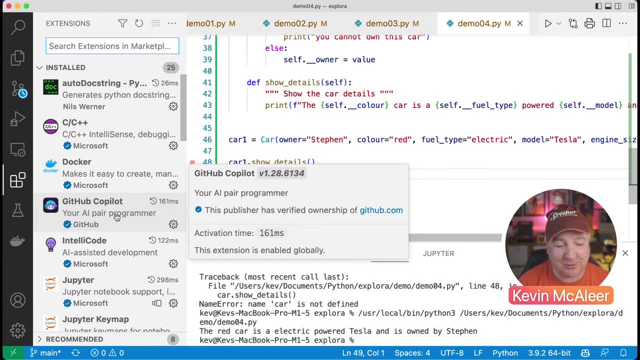 you're going to write is and it suggests that and all you need to do is press tab to auto complete it. so this is, uh, currently in beta and i don't think it's widely available, but you can sign up for it and mine was clearly accepted quite recently. so you just go to github: copilot, google. 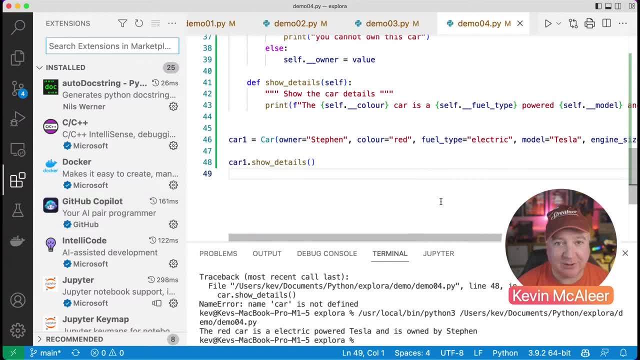 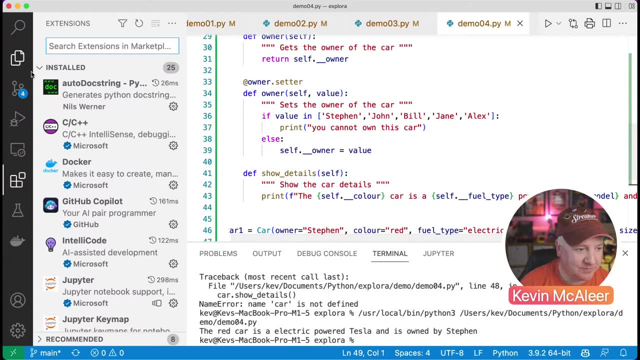 that you'll find on on github how to sign up your interest for that, and today it just popped up and said that it's working. so i've now got copilot working, which is pretty cool, okay, so let me just see if there's anything else i wanted to cover off on there. um, i don't think so. 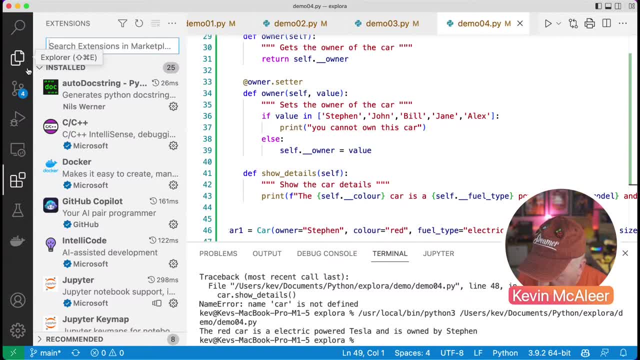 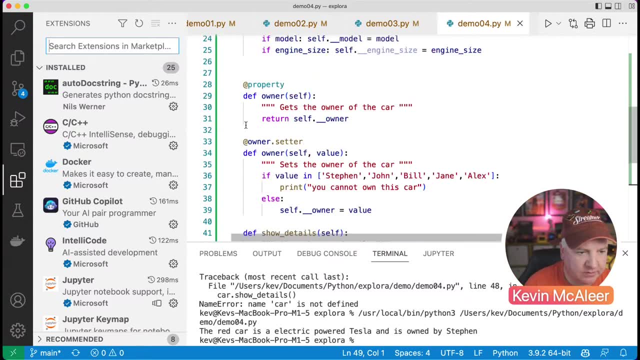 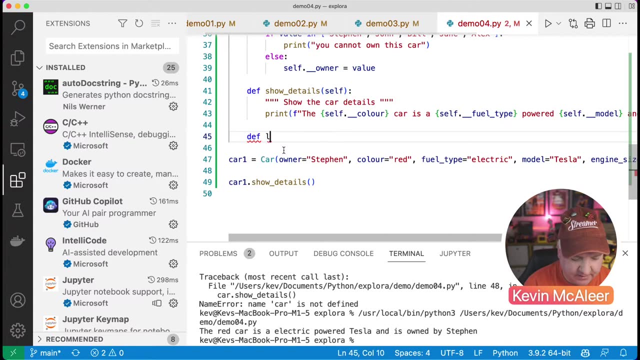 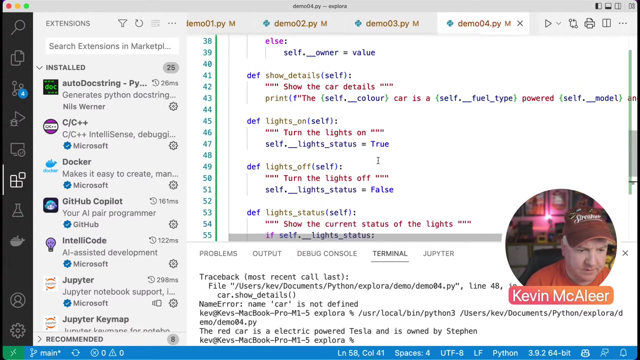 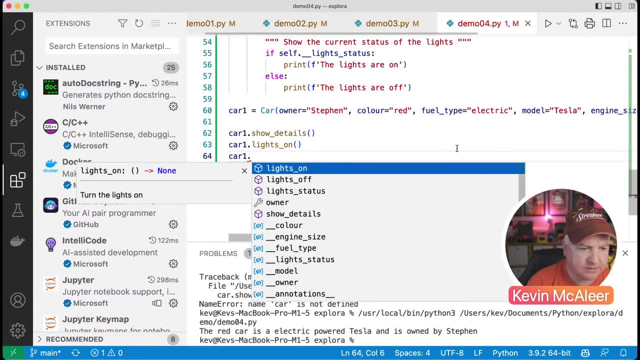 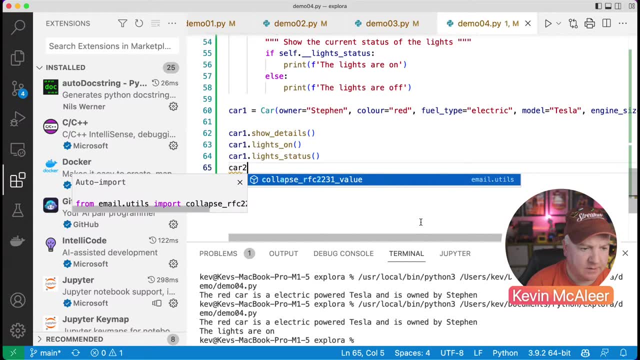 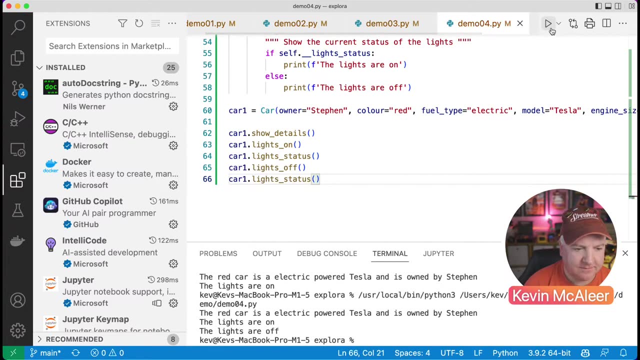 like so, and then let's do car one dot light status, so lights are on. if we then turn them off, car one dot lights off and then do light status again, we can see the lights are on. the lights are off. it works the way you'd expect it to. 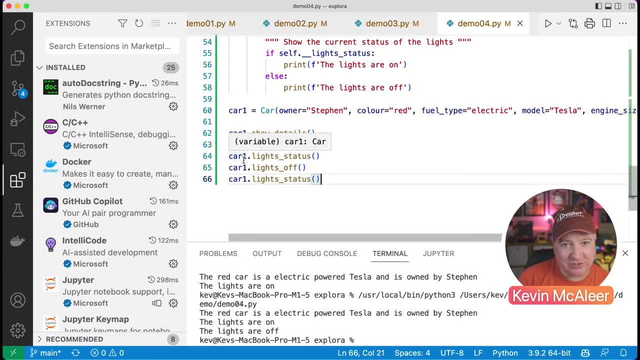 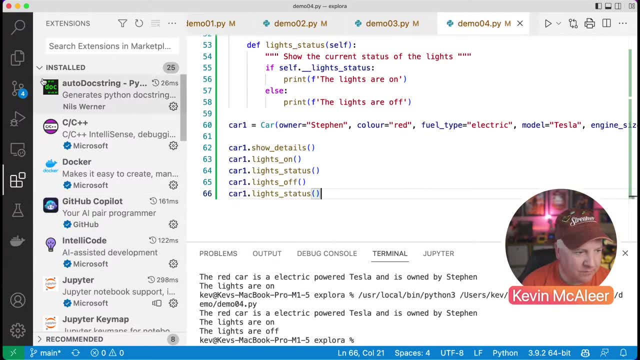 but they're related to car one. so all them variables, all those functions and parameters, they're all in that one class, which is called car. awesome, and if we can also go over to our explorer of code down here, if we click on this outline, you can actually see there the car class. 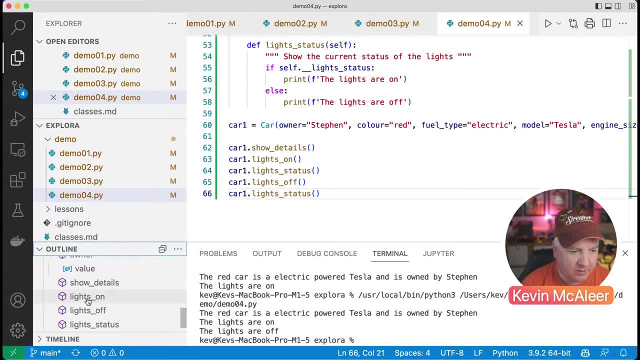 and then we can see that we're in the car class, and then we can see that we're in the car class and all the different properties that are available to you and also all the different functions available to you. if we click on one of them, i think we can also hover over, perhaps. 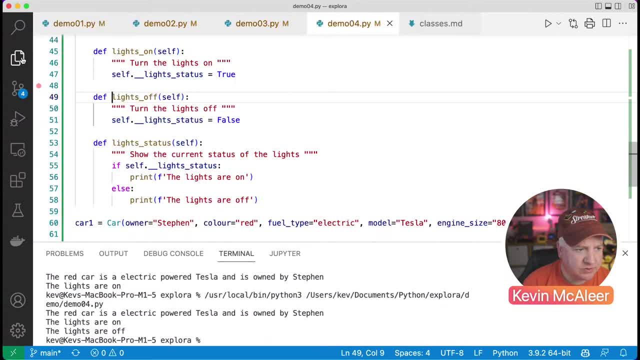 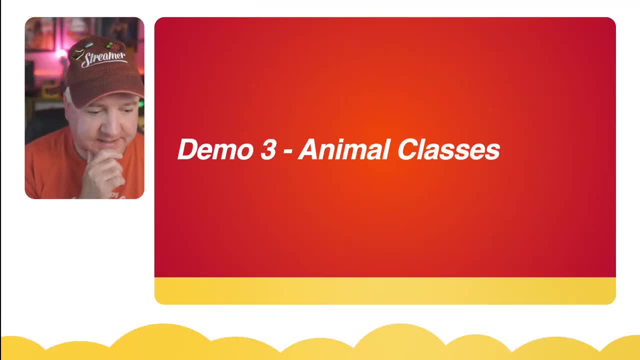 get some of the doc strings if we provided them. so, yes, it's good to to comment in your code, right? i want to go back over to the keynote. so we talked about animal classes. yes, i want to. i want to go through that, but before i do that, i also want to show you something really cool, so let me. 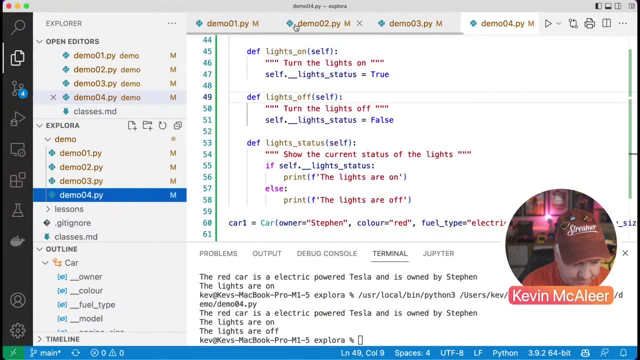 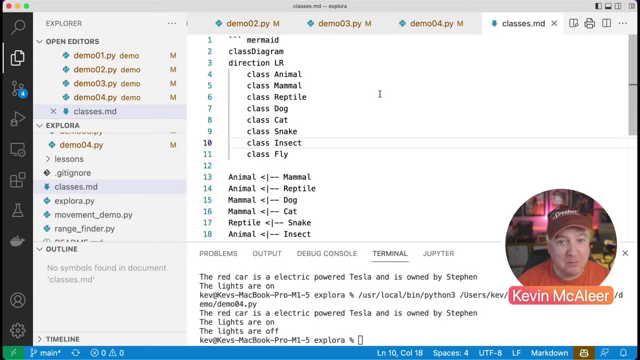 go back over to here. let me go into classesmd, right. so there's a really cool function in visual studio and github that's called mermaid and it's a way of creating documents but diagrams, but using code to create the diagram, so on. here i've got the um, the fence block, which is these: you have three. 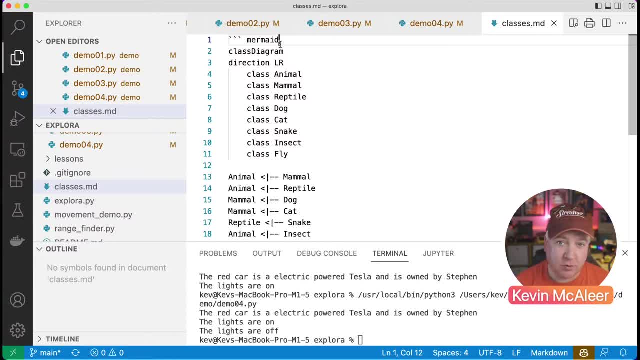 back ticks and then the word mermaid, and that tells it this piece of code is now going to be some mermaid and this is a mac down file. so, md, we tell it's a class diagram and the direction is left to right, and then we're. 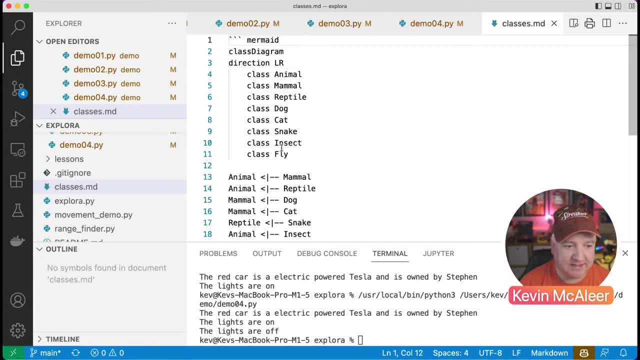 going to create a lot of classes- animal, mammal, reptile, dog, cat, snake, insect and fly- and then we're going to tell it that animal is derived from mammal, animal, sorry, rept. mammal is derived from animal, reptile is derived from animal, dog is derived from mammal and it will work out the tree. 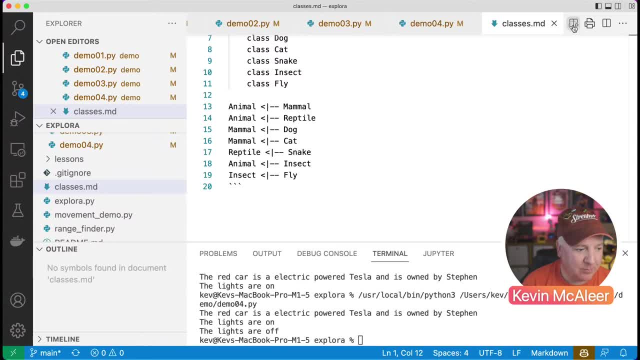 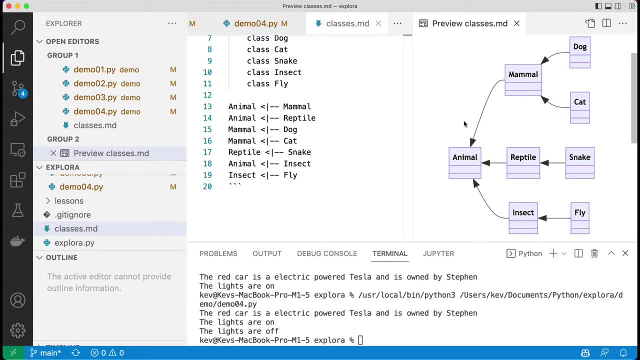 structure of this and i click over here on this little um preview. you'll see there that this, uh, let's move out the way there. you can see that it's created this diagram for us, and github also understands this and will create the exact same diagram within. 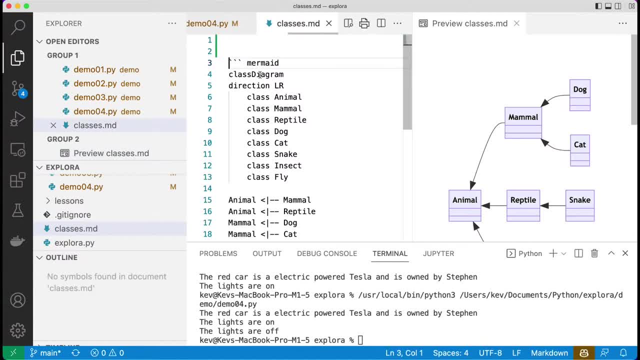 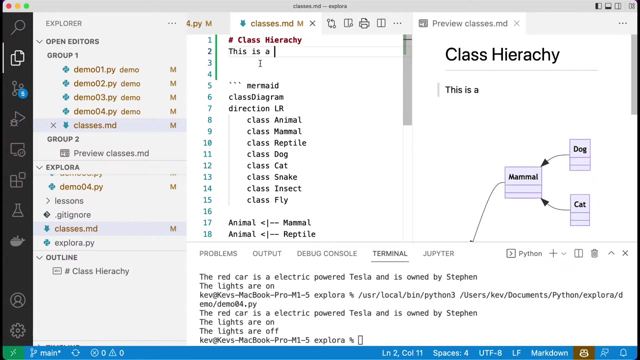 your code. so, because this is markdown, i can create um some text if i do heading one and just call this class hierarchy. i cannot spell it, so is that right? and then i can just say: this is a, this is a self-generated diagram, like so. and then we've got the, the diagram beneath it there, which. 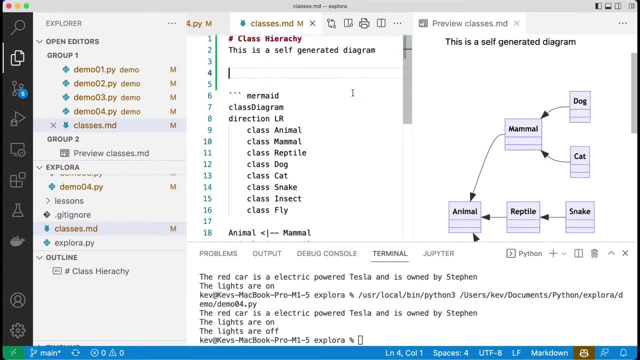 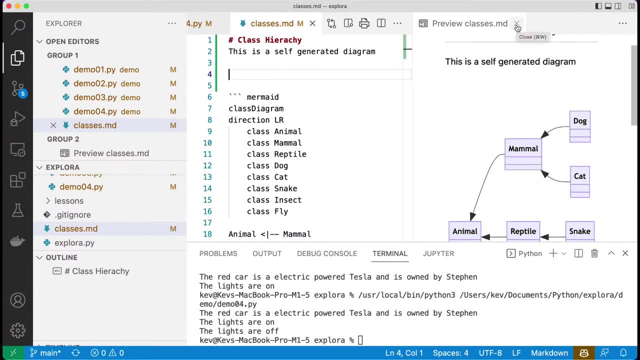 is just in this code block, and this is just using regular markdown but mixed in with it, we've got this diagramming thing. you can do all kinds of things with mermaid. it's very cool. it's something you should probably look into cool. so what i'm going to do now is we're going to go over to our 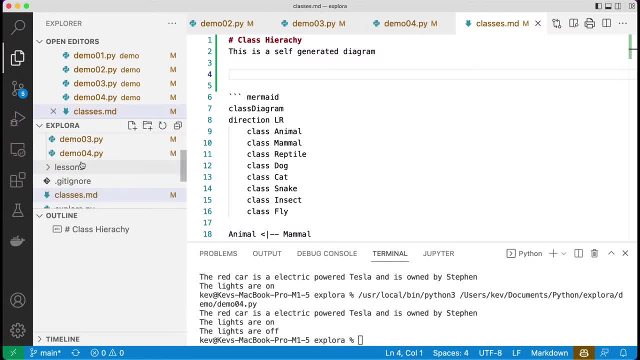 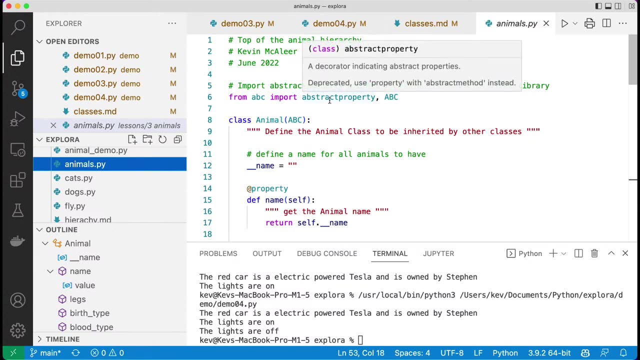 animals demo. so i've created these already so that we don't need to go and create loads and loads of things. so the very first thing we're going to look at is our animal class, so let me just find that animalspi. so again, this is an advanced python thing. we're going to look at abstract properties. 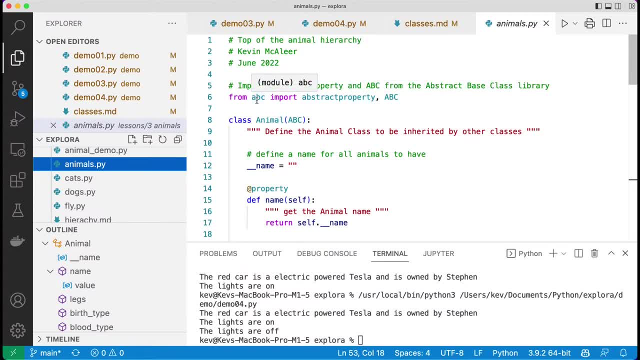 and abstract base classes. so abc is our abstract base class and we can bring in from that things like abstract properties and abstract methods. what we mean by abstract? when we create something that's in our class, we call that a concrete method or a concrete property. and if you're creating the 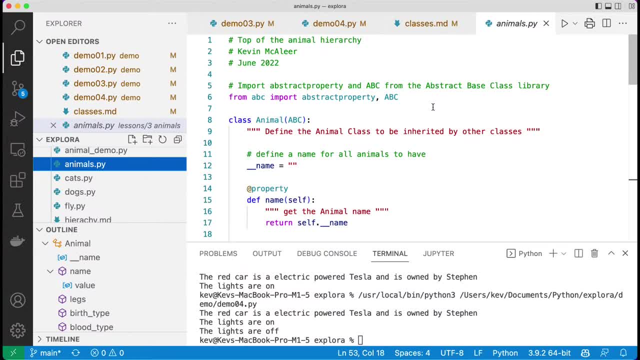 structure of class. so say you're like, oh, authoring a template. um, come back there, say you're authoring a kind of template class that you want everything else to follow. you can define what you want to be in there without actually defining how that should work, and that's what an abstract class is. it's kind of like you're. 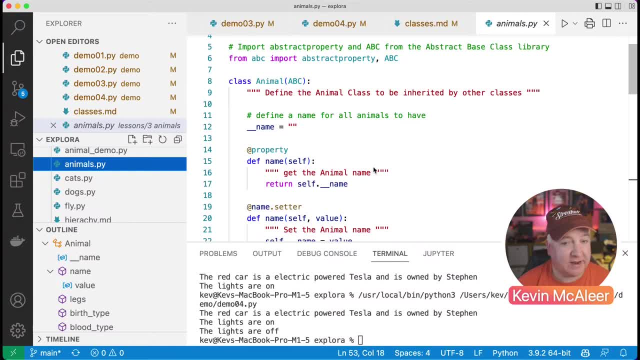 creating the skeleton for a class uh, without actually providing any details, and because we're defining it as a an abstract base class, anything that's then inherited from that has to provide that, otherwise there'll be a compilation error. so what i'm doing in here is i'm saying that 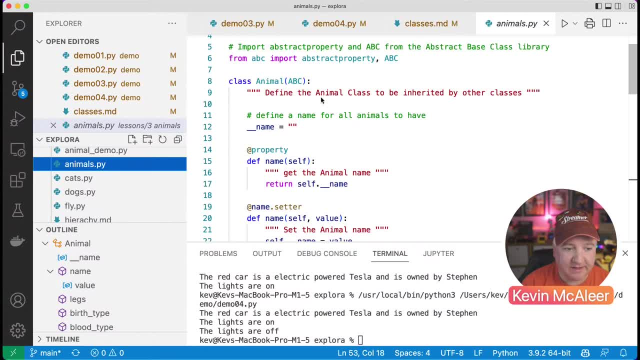 we're going to have a abstract base class that's called animal and we're defining the animal class to be inherited by other classes. every single class that's derived from this has to have a name, and we've provided the getter and the setter for the name and we've also got the number of legs. 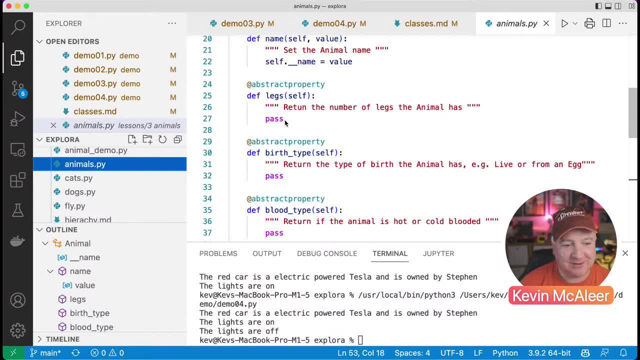 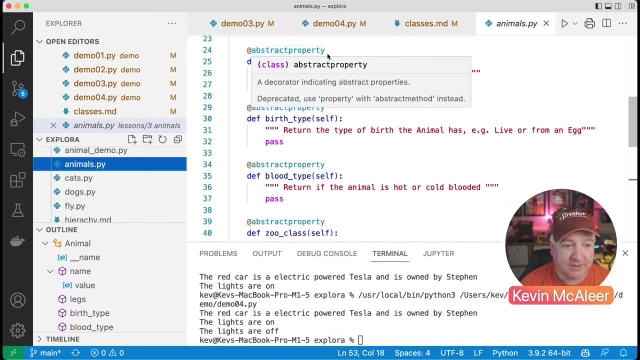 that the animal has, and i'm using pass there basically just to say these are not the droids you're looking for. move along, don't worry about what's going on there. and we've got these decorators that say abstract property and they mean you have to provide this, but this particular 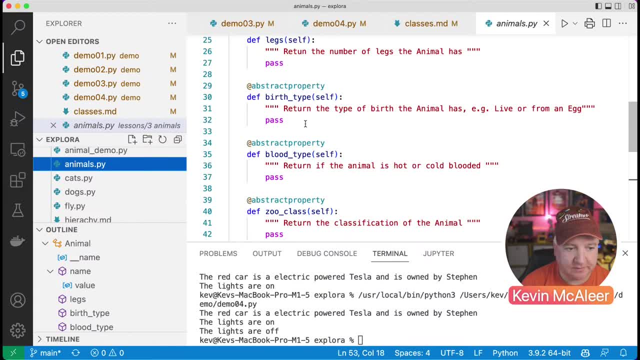 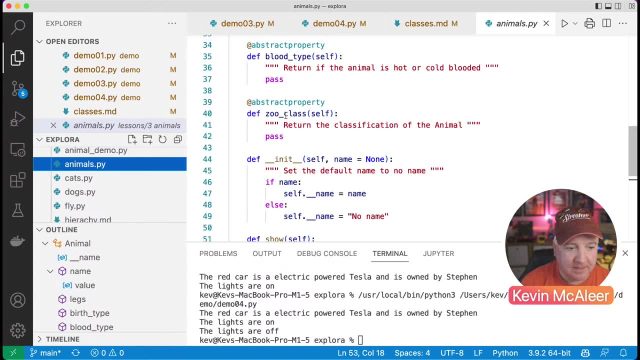 instance, doesn't have anything in it. it's just got the, the placeholder there. so we've got legs. we've got birth type, like is it a live birth or an egg blood type? is it hot or cold blooded? what classification is it so? is it an animal, is it a, not genus and all that kind of thing does it? 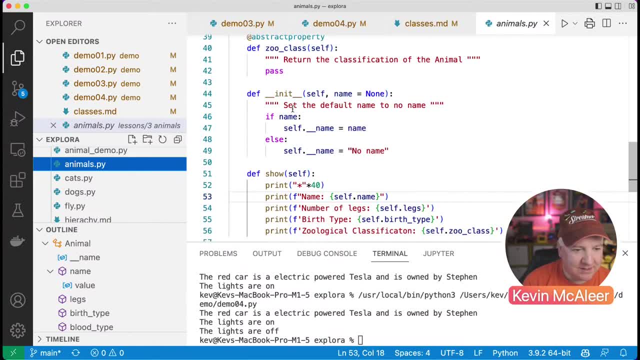 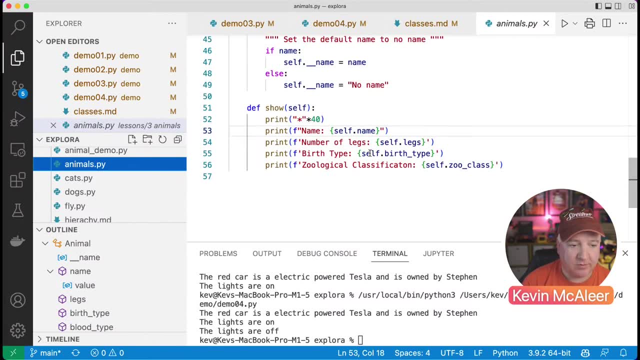 come from domains and so on, and we then say: if name is provided, then set the name to name, if it's not provided, then set it to no name. and then we've got a show thing a bit like our show details earlier on. we're on and we can use this. this is a bit more advanced python if we want to draw 40 stars in a. 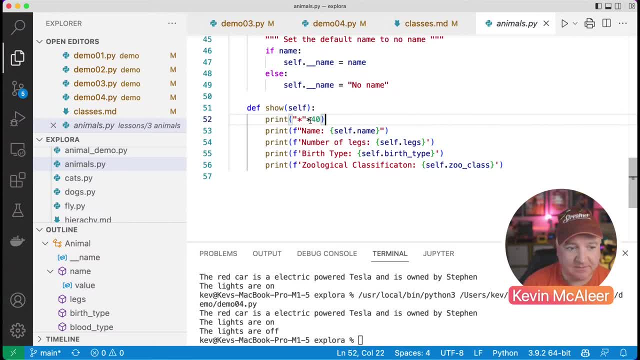 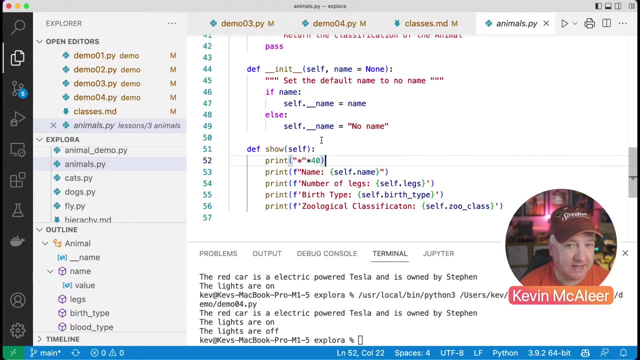 row. we can basically just say: the string star times that by 40, so do that thing 40 times. it just gives a nice underline. and then we say, using our f string, name is selfname, number of legs is selflegs, and so on. so every class that inherits this will have this function automatically built. 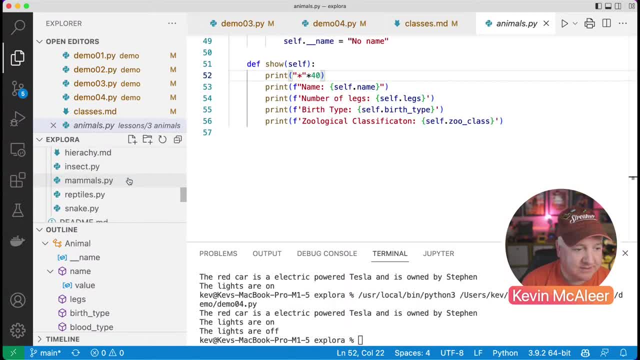 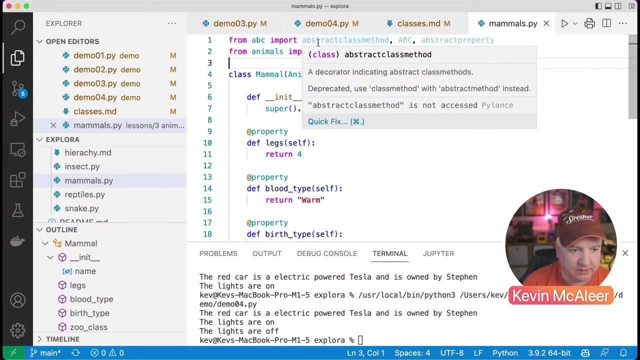 in. so that is our animals class. so now we're going to have a mammal class. um, notice, we don't use the abc. so we can actually take that out there. i can tell, because these are all in lower case, in sort of faded out and not being used. so i can actually get rid of that. and i'm saying from: 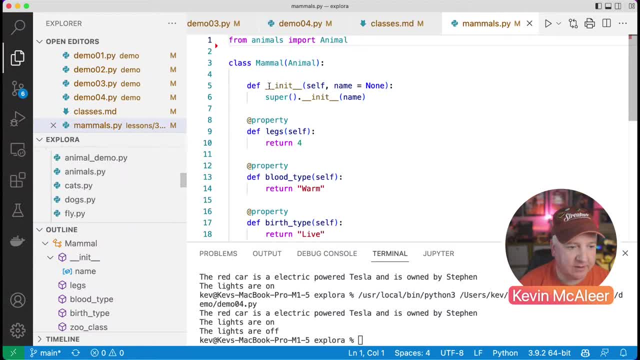 animal, which is that one we've just created a second ago here: import animal, which is the, the class that we want to use, our base class. so the class mammal inherits from animal. so everything that we want to use is our base class. so the class mammal inherits from animal. so everything. 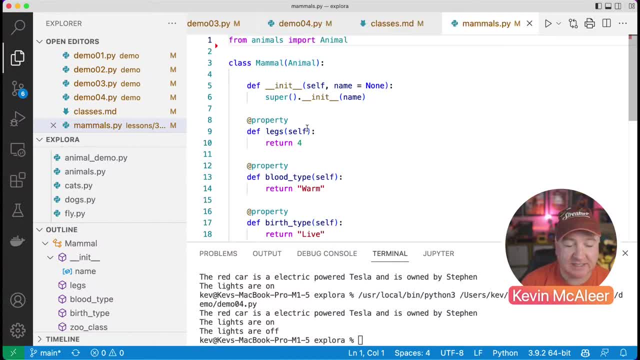 that animal had, mammal also has, and it has some extra things too. so when we create our constructor such as this one, here we're passing a name in optionally, we're also using super, and super means. call the initialization, the constructor of the, the class, the base class. 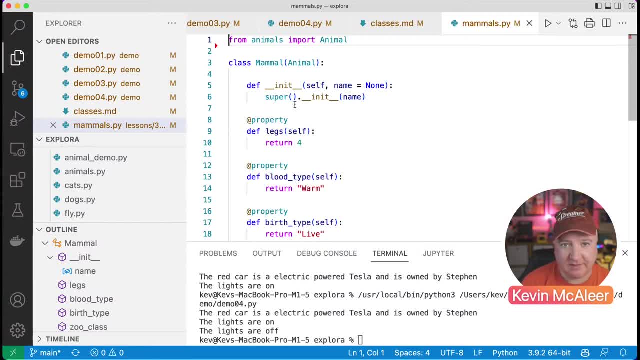 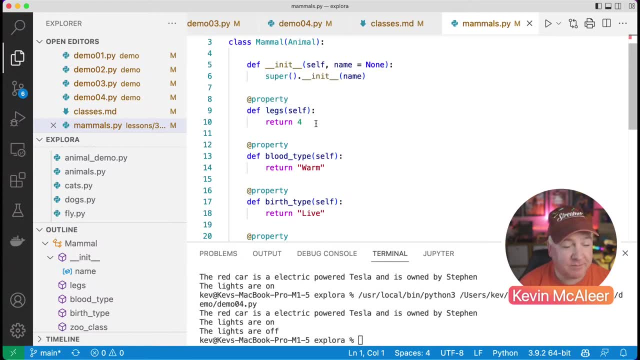 if we don't include that, it won't do that automatically and we won't get anything. any of those values are passed in properly, constructed properly. so then the, the properties that we have to have because they were defined in the abstract base class legs. we can say: return four. so mammals, in this case, have got four legs. i don't know if all mammals. 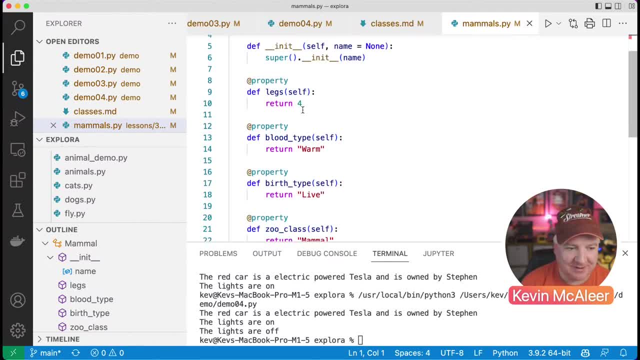 have got four legs. humans don't, uh, but in here i've just uh, overridden that. uh, blood type warm. i think all mammals have warm blood. they all have live births. the classification is mammal and if we show that, we basically just pass it up to the super whatever is in the one above it, show that. 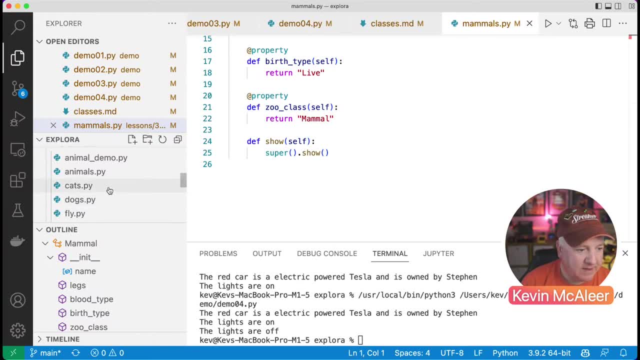 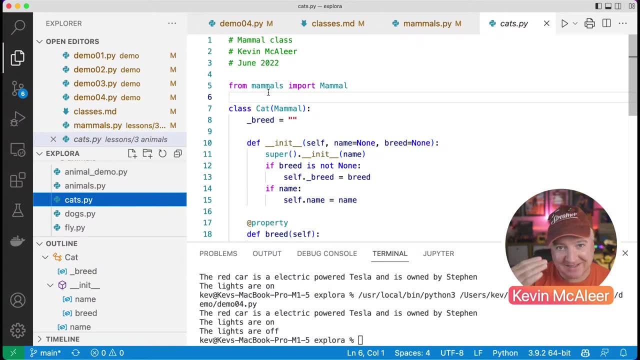 thing there, so that's mammal. we then got cats and dogs, so let's choose cats. so that's going to import from mammals. so again, this is the hierarchy in place here. we don't need to import animals because mammals already imports animals, excuse me. so then we say class is cat and cat inherits from mammal. 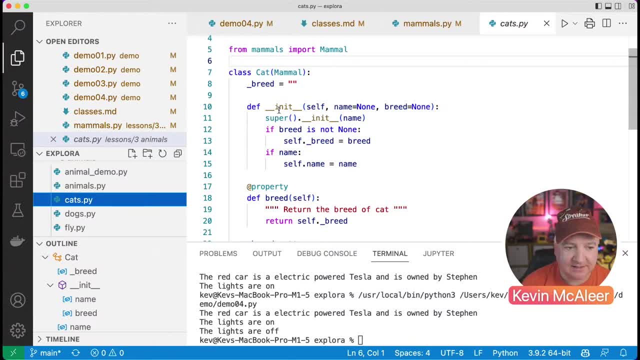 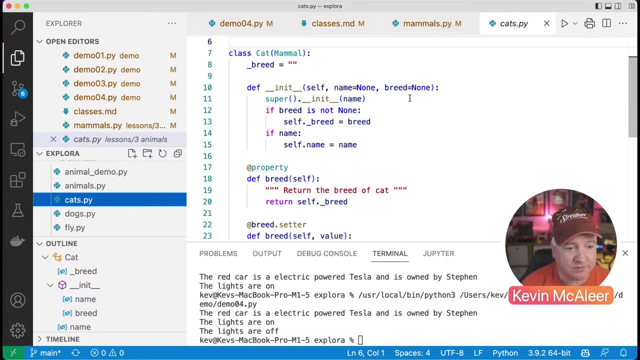 we can then say what breed of cats? this is the thing i'm enhancing in cats. so what kind of cat breed have we got? we've got our constructor there, so we're passing in, obviously, name and breed as well. if we want to pass that in when we create it we're doing the superinit, so whatever. 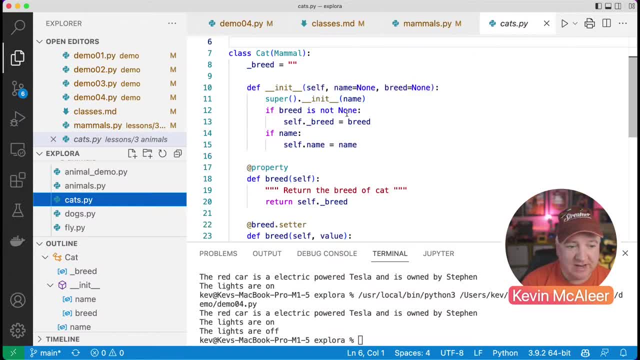 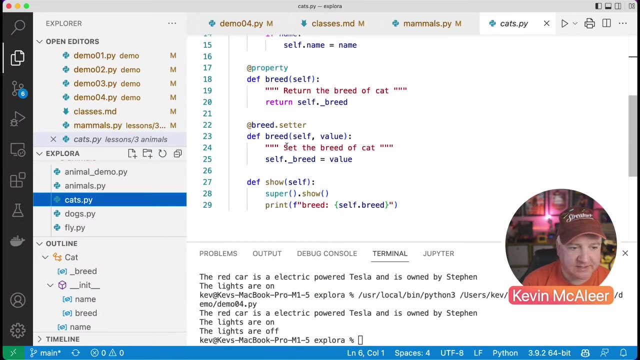 is in the mammal class. we want to run that as well. if breed is not none, then set the breed to breed, otherwise don't do anything. if the name is passed in, then set the internal name, the private name, to name as well, and then we have these getters and setters. so return the breed and set the breed. 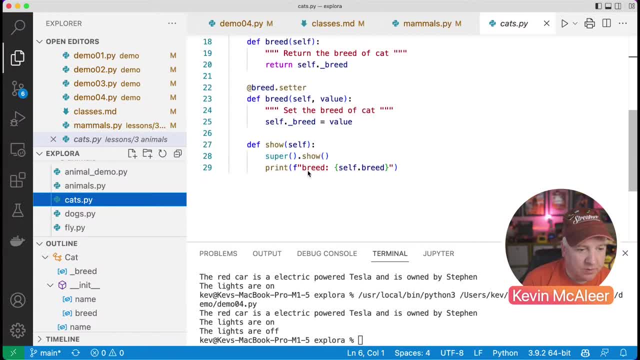 and we've also got show the breed. so, um, that is that. just got a question there. is this going to be available after the stream ends? yes, i'll. i shall post up the um. i think it's actually in the explorer. if you go to um the show notes, there is actually a link to the python library that's used and the youtube and. 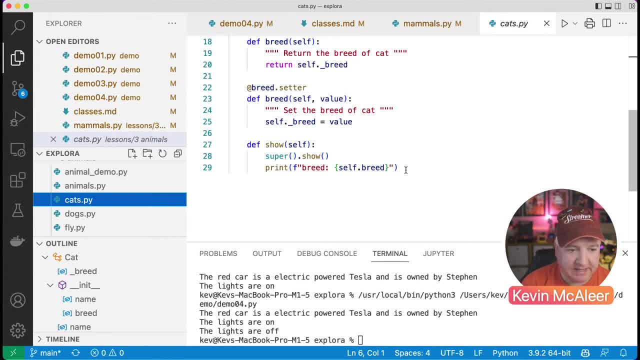 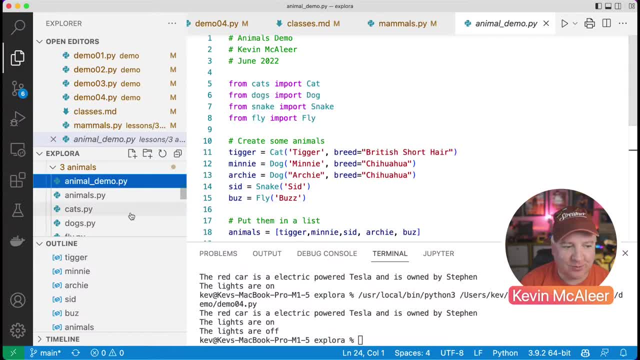 cats, dogs, snakes and fly. um, these are all ones i've created, basically just the same what you've seen before. i'm going to create some animals. so we're going to create a cat called tigger and the breed is a british short hair. is that right? is she a british short hair? yep, minnie is a dog, so minnie's. 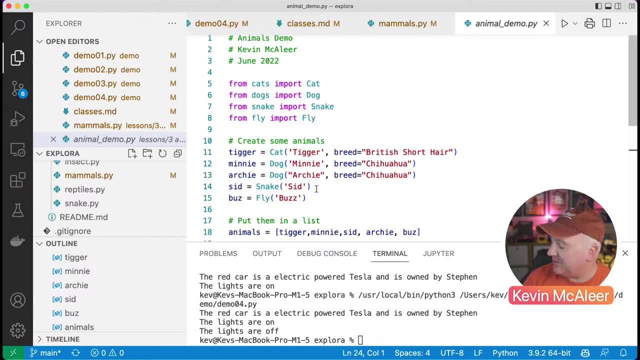 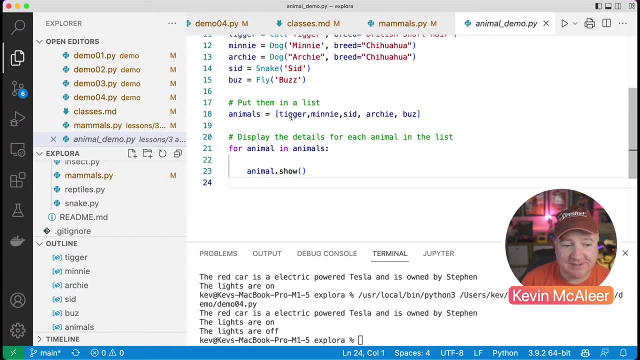 a chihuahua archie's. a chihuahua sid is a snake. we don't have a snake, but i wanted to create a snake and we've got a fly called buzz so we can also put them in the list. so tigger mini sid and archie and 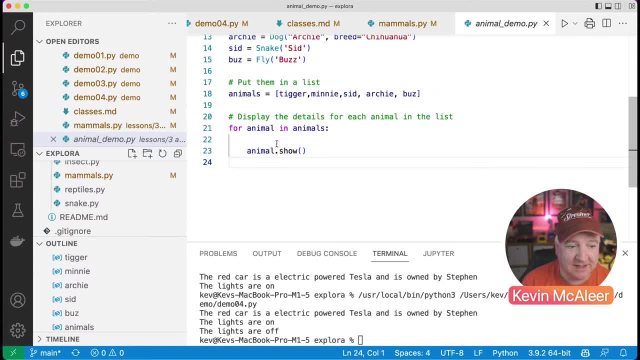 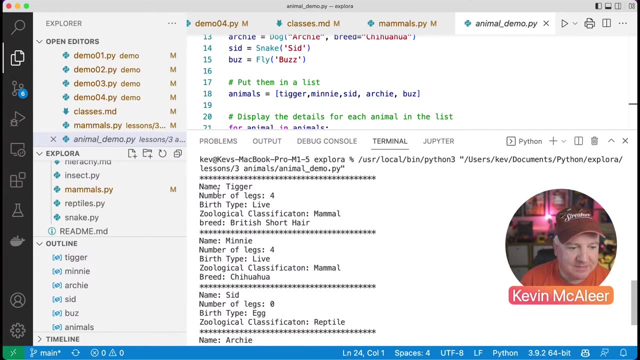 chihuahua- minnie is a chihuahua, and then we can just do a loop through those um so for each animal in animals show. so let's run this and see what happens. so we've actually got quite a lot of things going on here. so name, tigger, number of legs- four, birth type, live zoological classification. 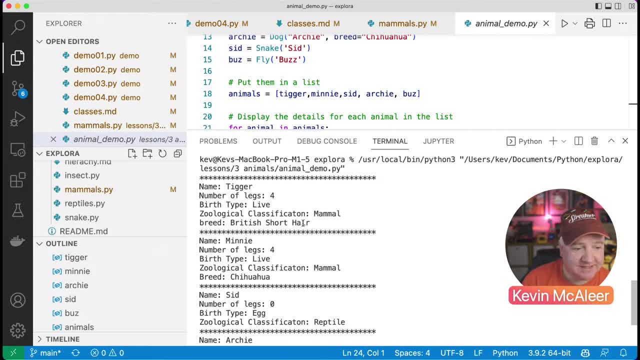 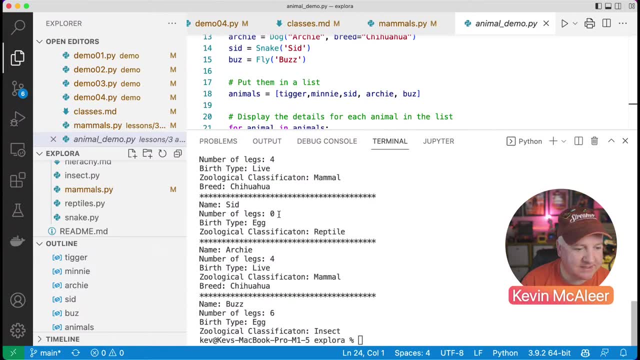 mammal breed, british short hair. it doesn't say it's a cat. actually on there, which we probably add in mini, is a chihuahua. it's mammal live, four legs. sid has zero legs because he's a snake, the birth type is egg and the classification is a reptile. and we have another four-legged animal which is a chihuahua. 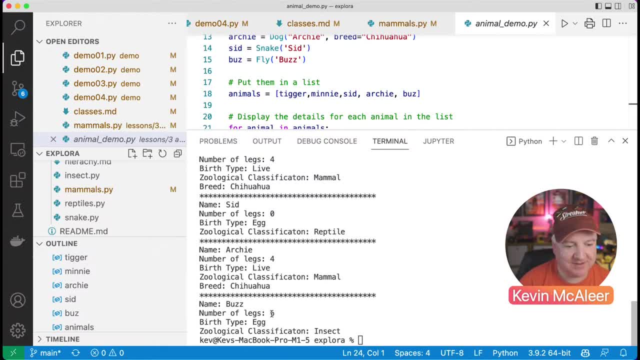 which is archie, and then finally buzz, which has got six legs because it's a fly, birth is egg and it's an insect. so you can see what happens when we we run these various different things. when we say animalshow, it's, it's going through each of these and saying: whatever the 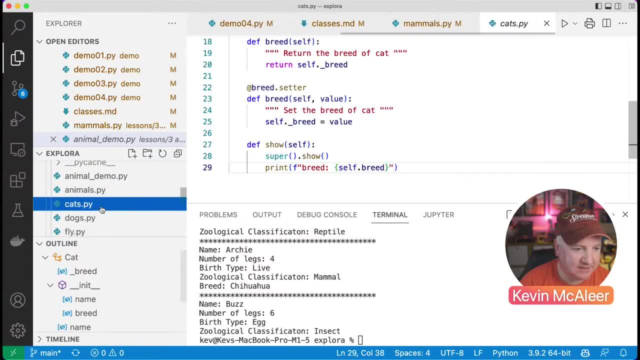 catshow function is and it has to go find the cat library, has to find the show. it says breed is self-breed, so if we have a cat it will show the breed, which the other ones don't do. so see there, british short hair is on cats, um, but sid the snake doesn't have. 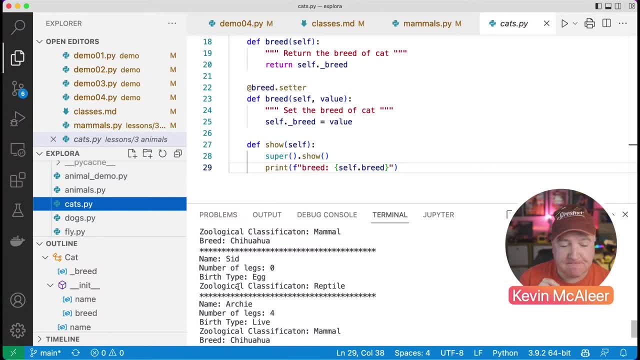 a breed. we haven't included that in that particular type of- um, uh, that particular class. so we can make our classes more and more refined and more specific the further down the go. but they all inherit everything from the previous one and we can see that when we're. 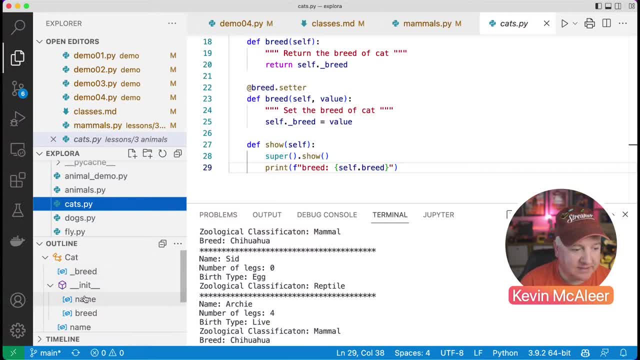 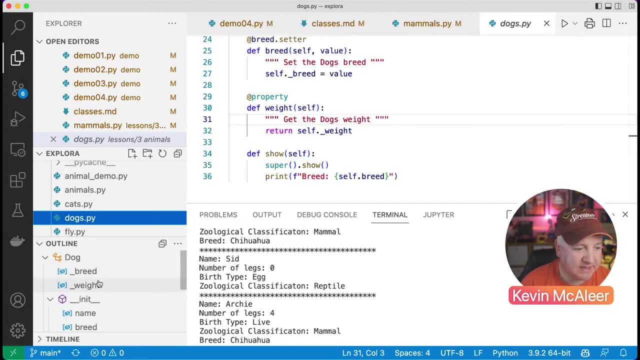 looking through here. so cat has got breed, it's got a name and it's got a show function. if we go to the dogs, we can see dogs have a weight that's different than the rest of them and that dogs can wag the tail as well. so if we go back to our animals demo, we can make one of our dogs, so we 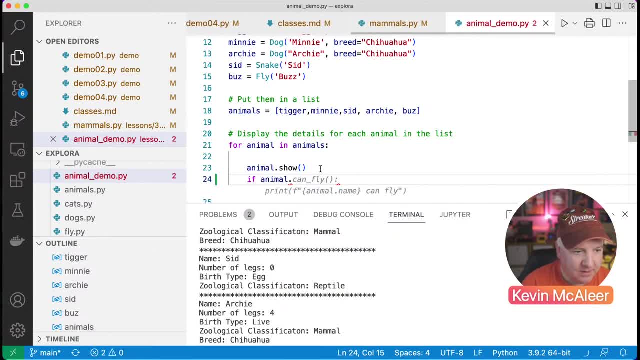 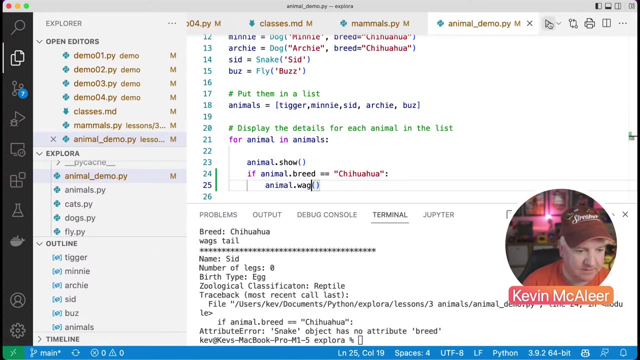 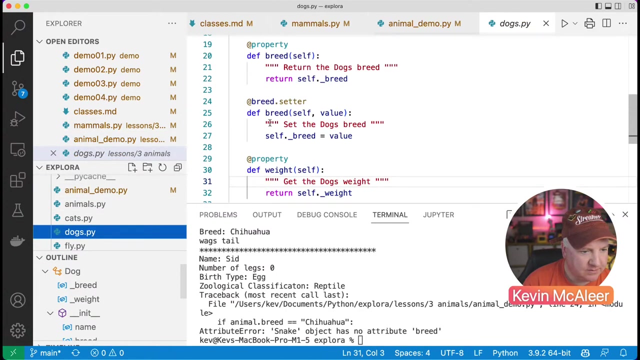 could say: if animal dot breed, uh, equals chihuahua, then we can say, wag, is it wag? let's try that. um, no, it doesn't have the thing called breed. so what do we call that in dogs? um, what do we call that? i thought we called it chihuahua, so it was breed. 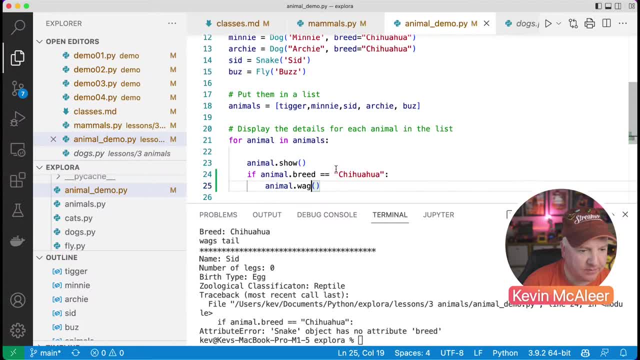 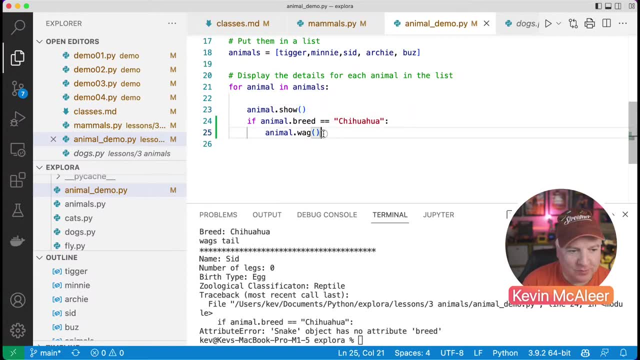 oh, snake has no object breed. yeah, there we go. so that's that's the problem that's happening there. so so that that breaks my code there. so that's something to think about there. um, we can have all kinds of different things depending on what the type is. now, yeah, we can. 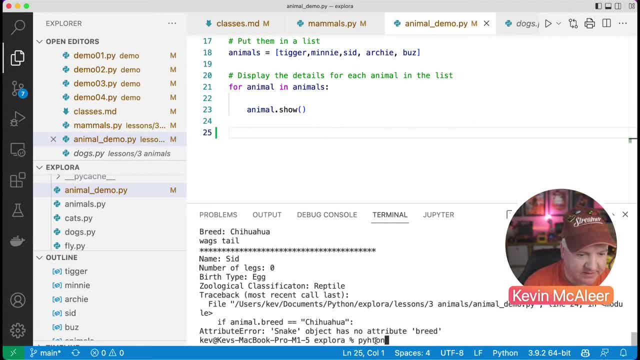 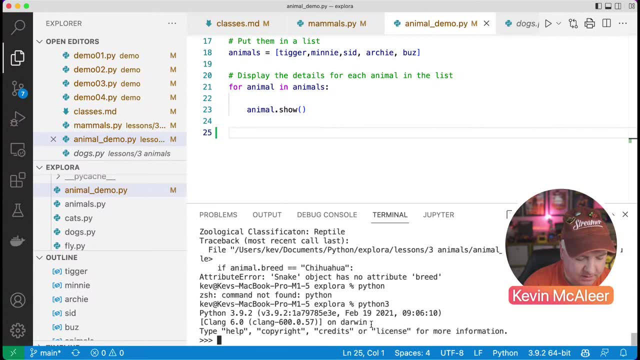 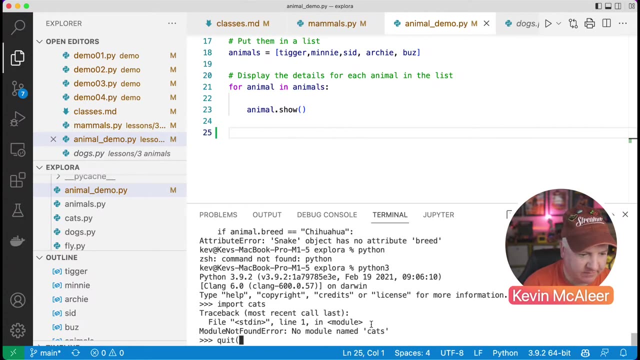 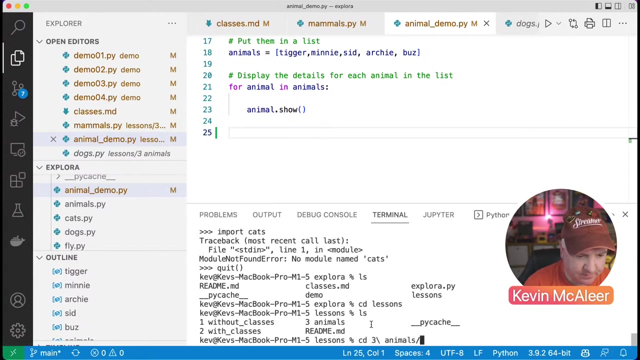 actually look at types as well. so if i go into the interactive python editor here and, oops, python3 and i'm going to import, um, cats, i think i need to be in the correct folder, which is actually lessons and then animals. yep, so if i now run python3, i can then do it from cat. let's import cat. 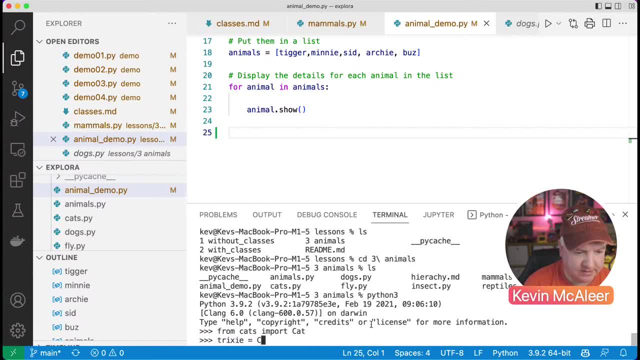 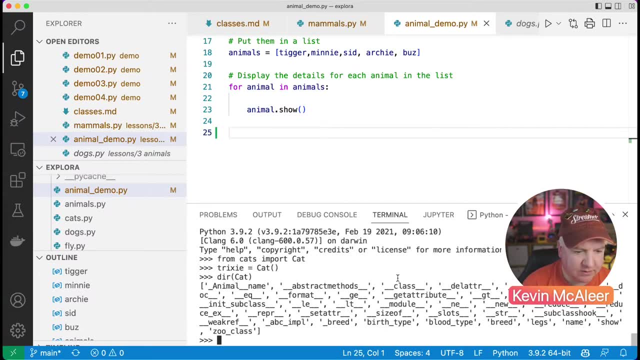 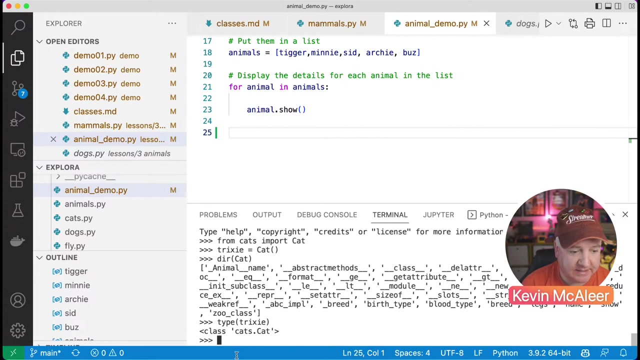 like. so i can then say tricksy equals cat. so i can say cat and then if i do dir cat, i can see all the different things within that class. so i can see the breed, the birth type, all that kind of good stuff. and i can also say type. so what type of thing is tricksy? and it will say it's a type class of cat. 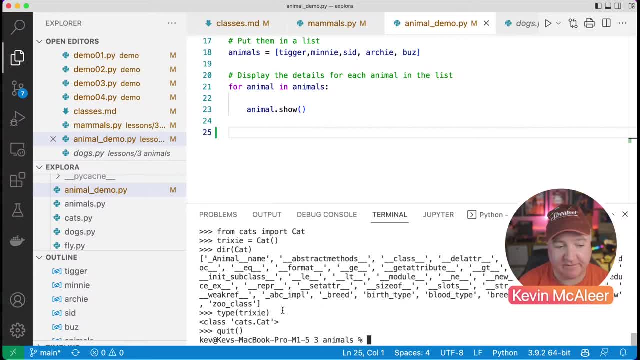 so we could use um, we can use type to define and to check for things as well, cool. so i think that's all the code there i wanted to show you for animals and mammals, just checking through if there's anything else that was cool that wanted to look at. so your abstract base classes concrete. 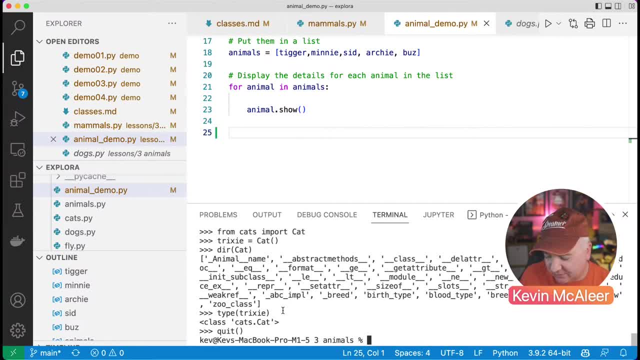 base classes, sorry, concrete classes. that's something to look into if you've not looked to those before, and it's a way of sort of defining your classes and what you want this thing to do and kind of creating like a skeleton. for that there is another technique that's called protocols. 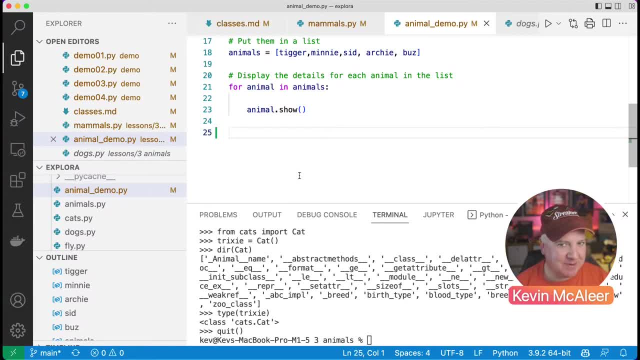 which, um, that's called duck typing. so if something looks like a duck, sounds like a duck, then it probably is a duck. that's what they mean by that, whereas when we do inheritance, we're actually saying it inherits the values and protocols, basically just says it has to have these. 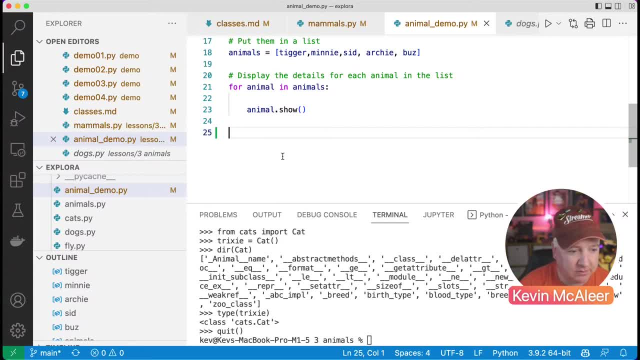 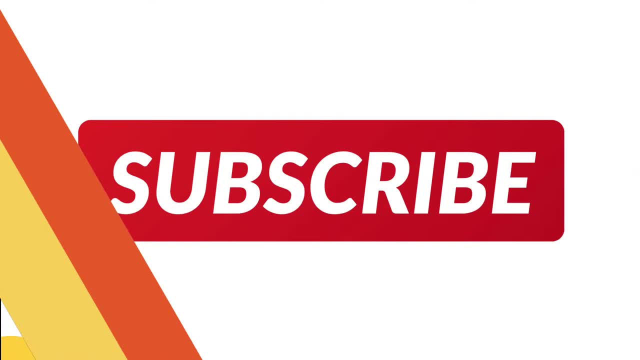 variables and these functions for it to adhere to a particular protocol, but it doesn't actually inherit the class, it just has to have those. okay, so let me get back to my keynote. i think we are nearly done on there now. so yeah, if you want to join me on discord, you can head over to 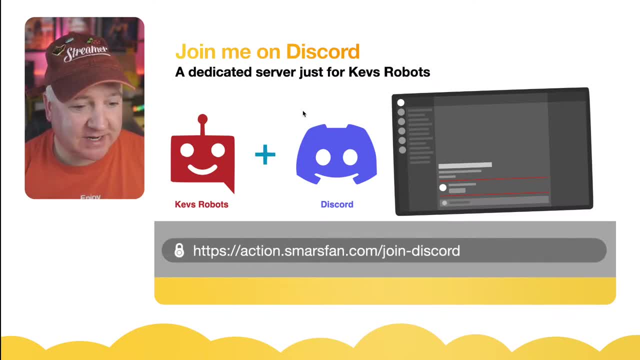 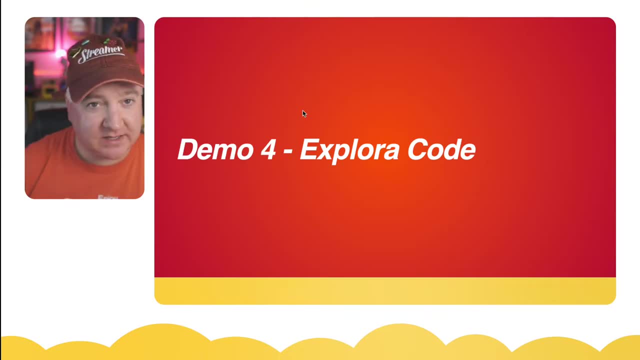 actionsmilesfancom, join discord and you can join our discord server and continue the conversation at deeper level. and finally, we'll have a look at the explorer code. so the robot i have that's called explorer, which is um, sat over there. so the yellow and the white 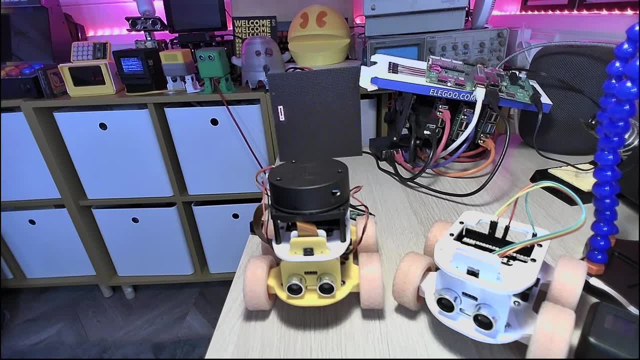 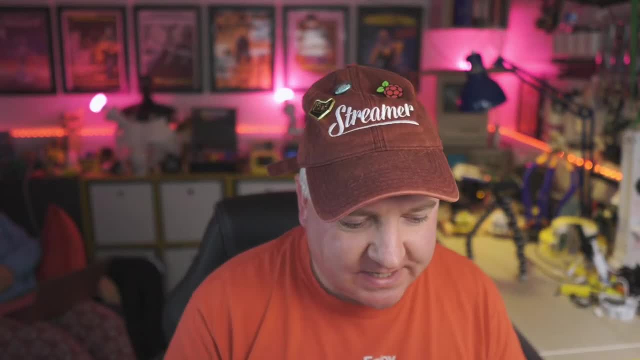 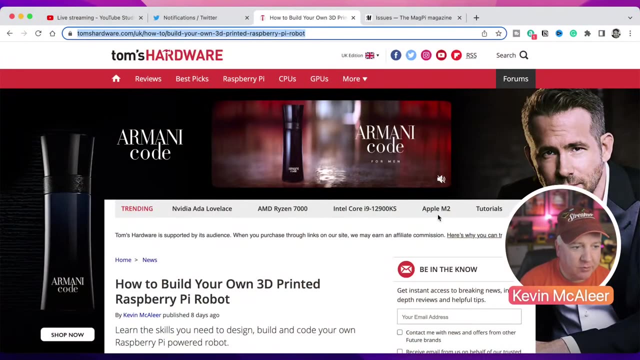 robot. they're both explorer robots. they use the uh the explorer uh hat from pimroni and um, they're a robot i've been working on for for quite some time and recently- let me just find on my uh, my browser here- i wrote an article for tom's hardware about how to create. 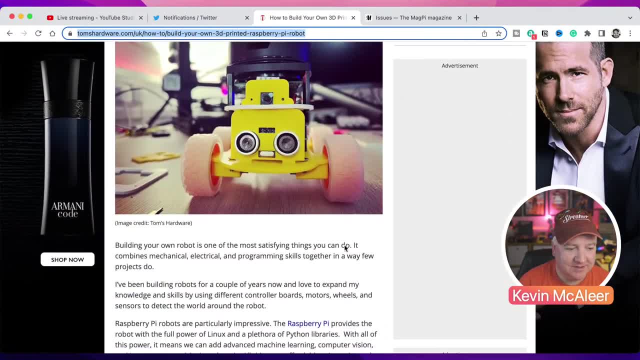 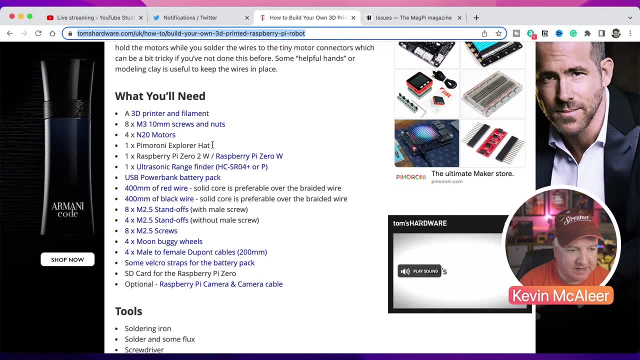 your own 3d printed robot and that's the explorer robot. so part one is basically how you print out. so you scroll down there all the all the bits and pieces you need, such as the explorer hat, um, all the different tools you need, and it's got step by step how to create that and how long these 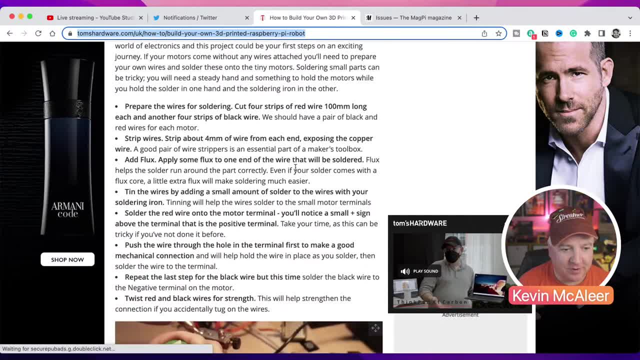 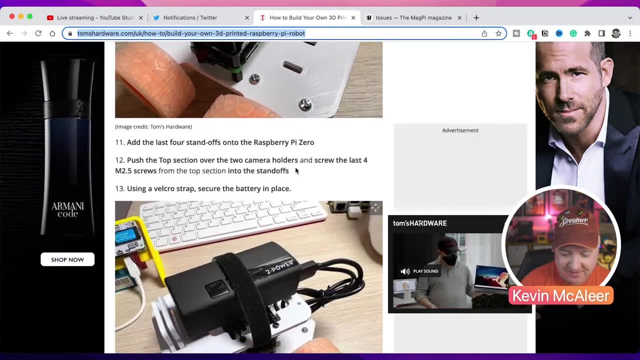 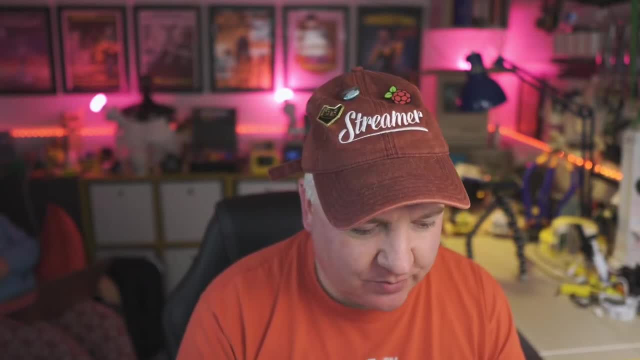 things take to print and so on, but basically you can print your own robot and join along. so that's going to be the code that brings this to life. so that's what this show is basically about today and, um, if i get back over to visual studio, i can give you a bit of a sneaky peek of what the code. 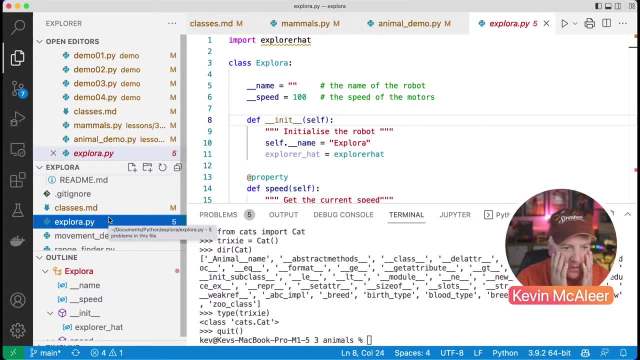 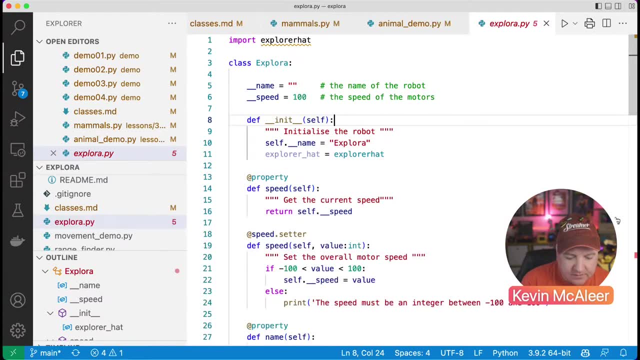 looks like there, okay, so let's go back over to um visual studio. so what i have on the screen if i just um move this out of the way, let's just uh, get rid of that. so the first thing i'm doing is i'm importing explorer hat, which is the pimaroni. 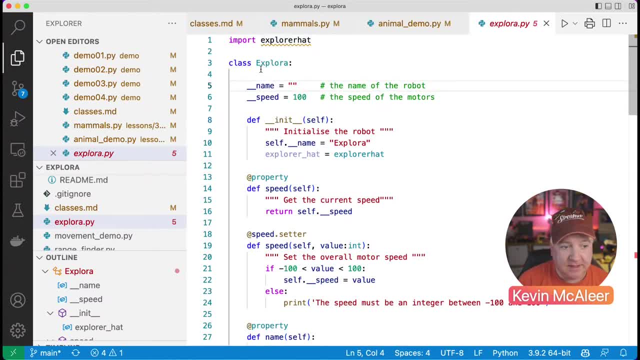 python library for using the explorer hat. i'm then defining my own class for my robot, and my robot only needs a couple of variables, so i'll let it have a name, so you can name your robot, and just having a speed, so we've got an overall. how fast should the motors be turning, if just as a default? 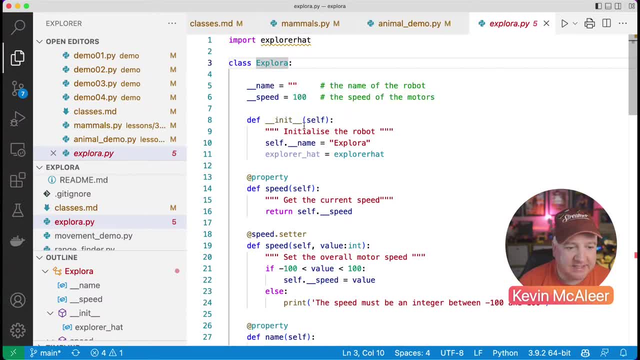 speed because we use that throughout the code. we've then got an initialization function and it just says the name is explorer and explorer hat equals explorer. i don't think i actually use that when i'm doing a code in my computer to do it, but i will let you know if that's something you'd want. 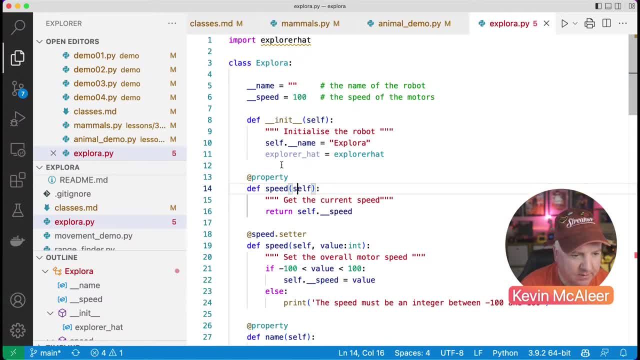 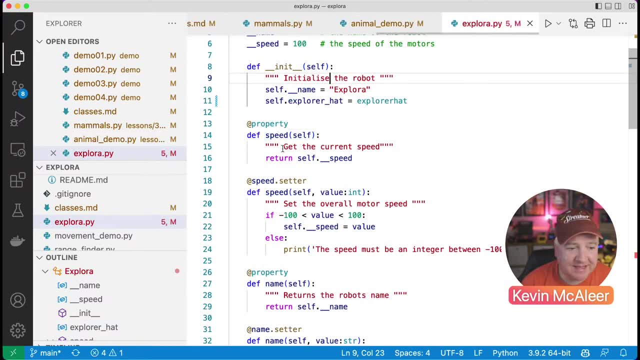 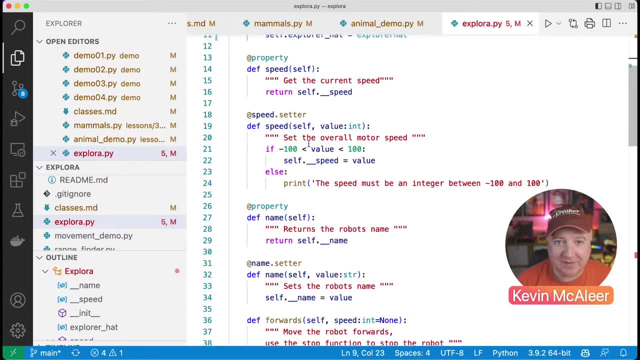 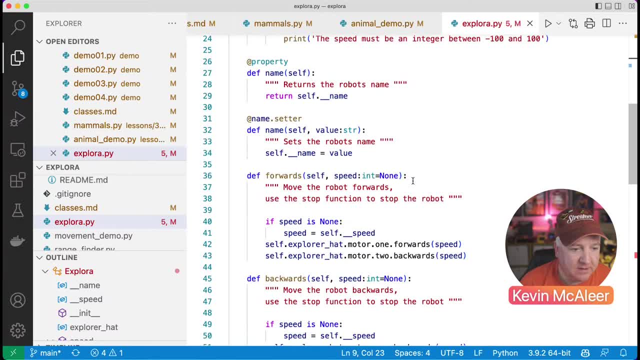 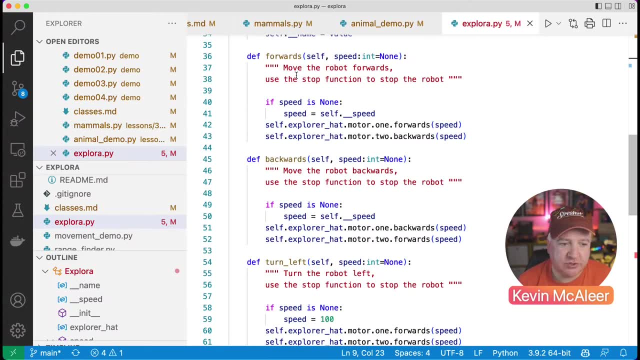 between minus 100 and 100, then we can set the internal private value. otherwise we can raise an minus 100 and 100. we then allow the user to set or get the robot's name and then we've got some movement functions. so we want to move the robot forward. we can pass in a speed which needs to be. 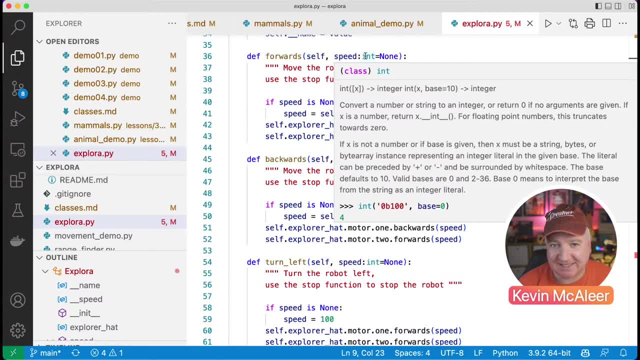 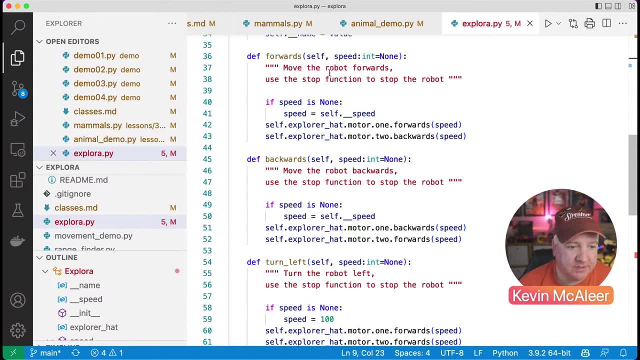 an integer. so the colon says: this is what type is a type? hint should be an integer, but it can also be optional. we can just use that internal speed value that we've got further up the code so it moves the robot forward and we use the stop function, which is further down, to stop the robot. 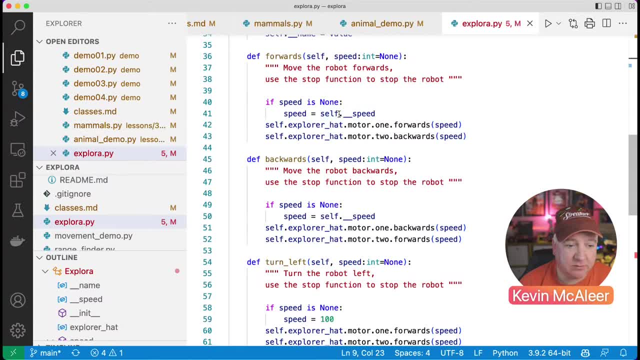 rolling forward. so if the speed is non, then the speed becomes equal to selfdouble underscore speed- that value we've defaulted to. and then selfexplorer hat motor one forwards and self explorer hat motor two backwards, and that's because the motors are actually facing in opposite. 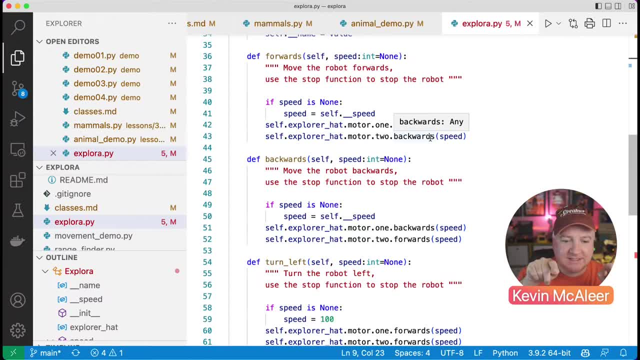 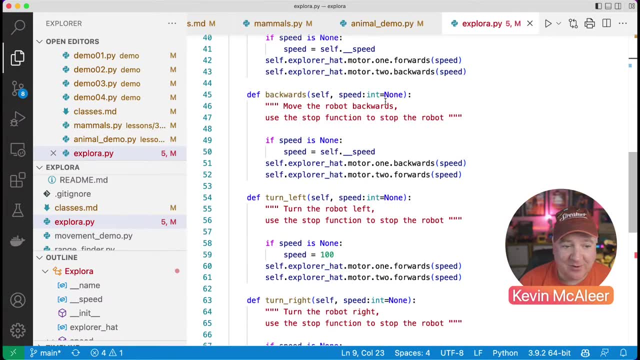 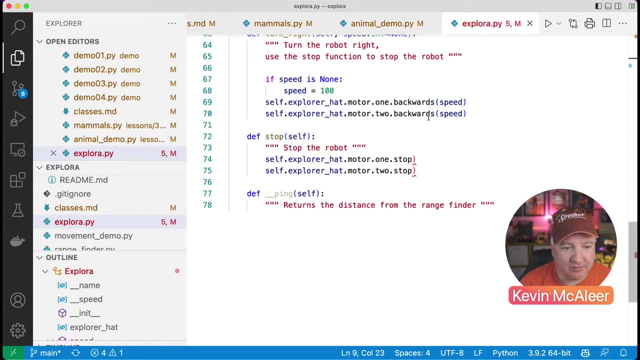 directions and therefore the direction they're turning in is kind of the opposite, to make them go in the same direction. so that's why one's forward and one's backwards to make the robot go backwards it's basically the reverse of that. so backwards and forwards. to turn left, they both go forwards. to turn right, they both go backwards. 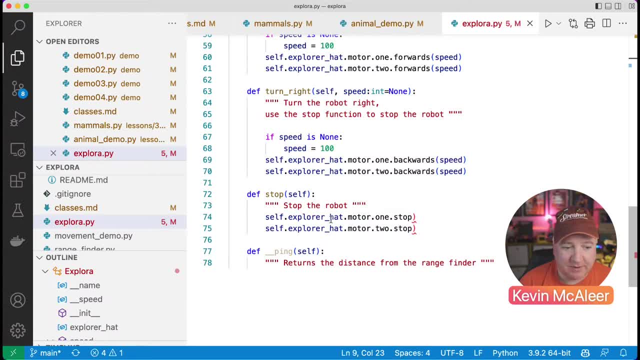 and to stop it we basically just pass in stop and that passes in motor one dot stop. i think that probably just needs to have that at the end too. okay, i need to test this code out before we we run this. and then finally, the ping is for the range finder. now i'm actually not going to do. 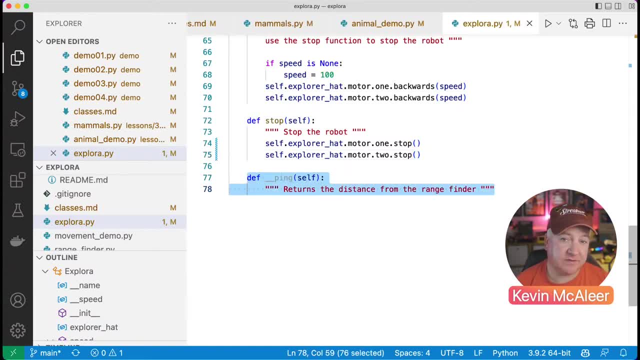 it like this: i'm going to create a new class for the range finder, because i've actually created that previously and all the internal workings of how that work we don't need to worry about. in our explorer hat code we can basically just say ping and it will return the distance, so we can just do. 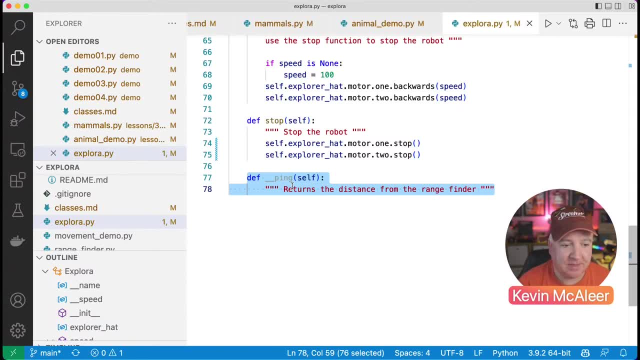 dot distance and we can figure out what that is in front of us. um, and it will figure out how to do all the measurements and the speed of sound halved and all that kind of stuff that could be in a separate range finder class. so i'll create that as a separate piece of code. we'll have a stat. 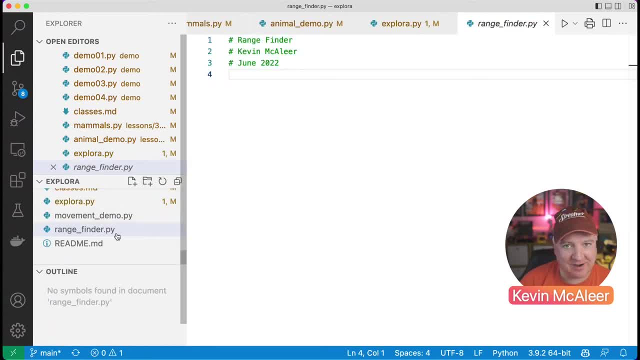 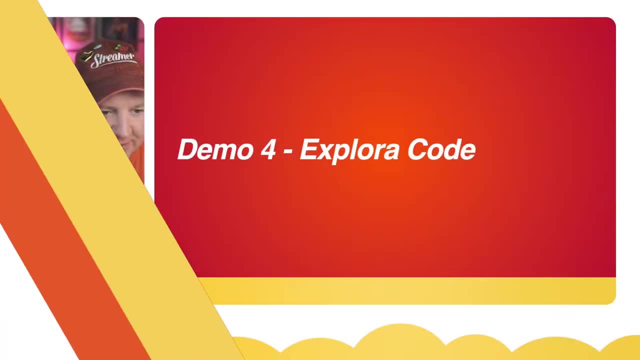 to do that, but i've actually not finished that yet. so that's kind of where i'm up to with that code. i just wanted to give you a sneaky peek of that, okay, so let me just have a look back on the keynote, because i think that's pretty much everything i wanted to cover off today. yes, it is so. um, the. 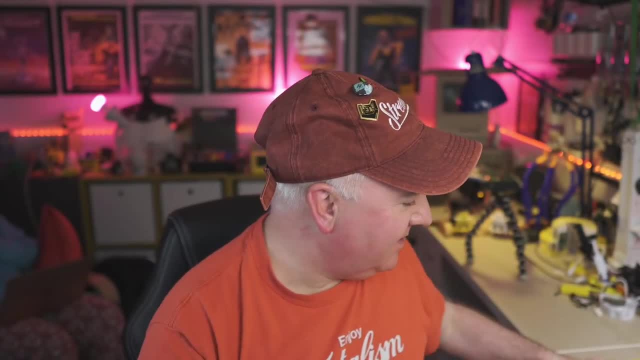 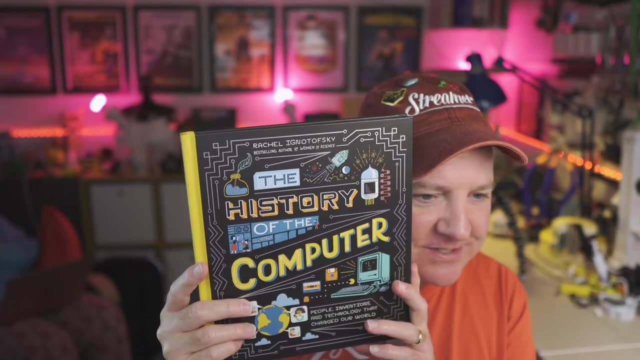 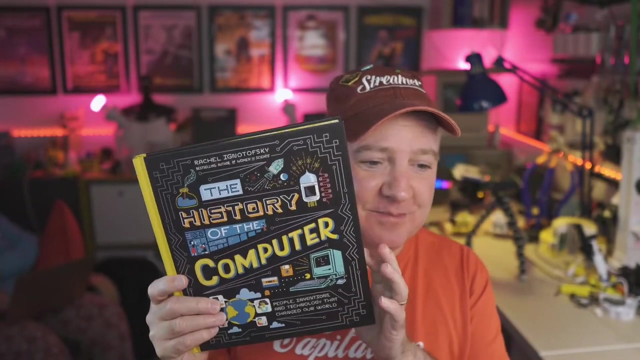 other things i wanted to cover off while we're all together is um this book i bought, which is by rachel- i want to try that name- ignotus sky, oh, not of sky, and this is a fantastic book. I'm not sponsored at all, I just love the. 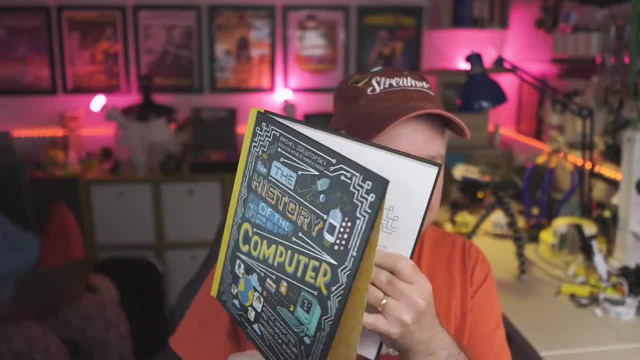 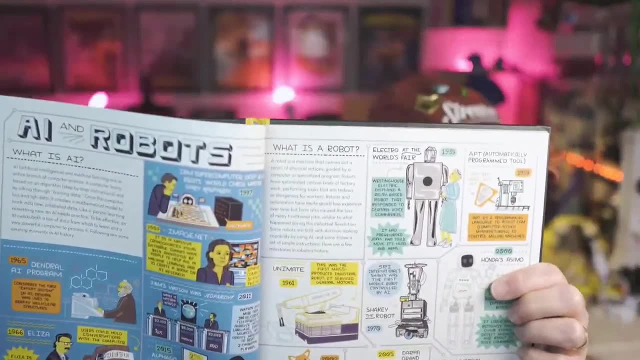 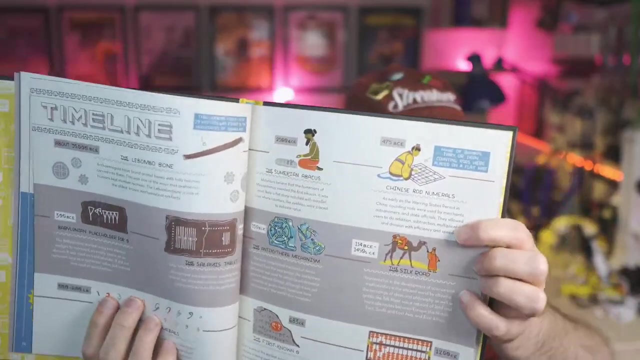 artwork in this book and I thought I wanted to sort of show this off. so it's history of computers and the artwork in here is absolutely amazing. just take a look at some of the the artwork in there don't to sort of show the entire book that you need to come by your own copy of that, but if you work in a school, 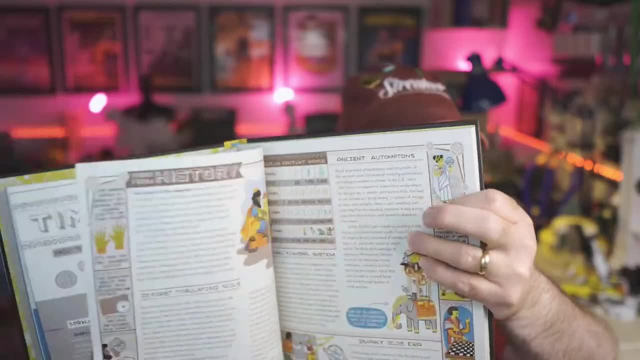 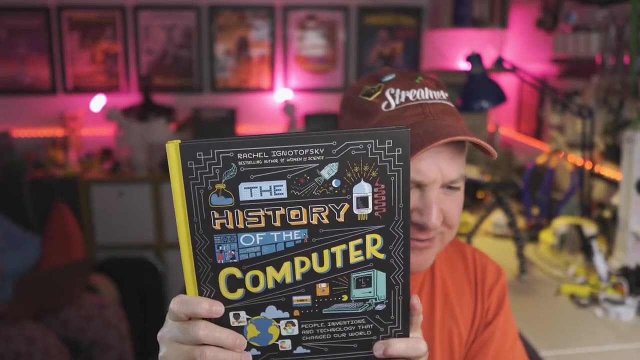 work in a library, or you just love computers as much as I do and you want to have your own copy of this, then seek that out. it's the history of computer and it's by Rachel Ignot of sky, and I'm probably butchering a name that I just 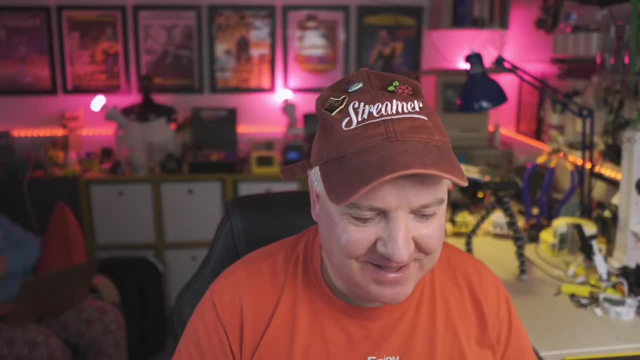 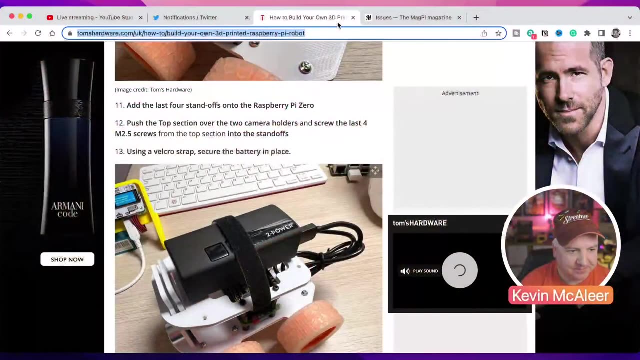 wanted to show that because it's so nice. the other couple of things I wanted to show you as well before we get into the Q&A, is a couple of things we talked about the the Tom's hardware article, so I'm now writing articles for Tom's. 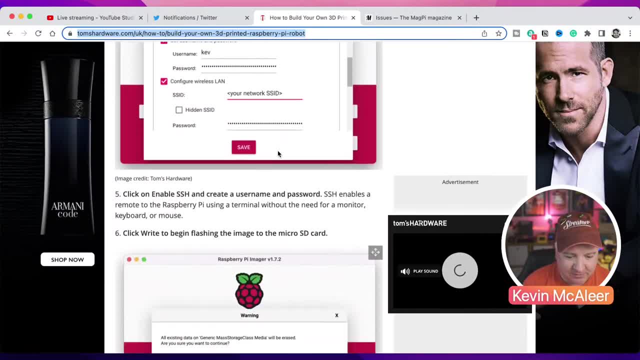 hardware, very detailed articles as well. they are in there. and also I want to show you this portrait by this guy. I'll show you this one here, but I don't want to show you this part of the photo. I wanted to show it. this is what we have. 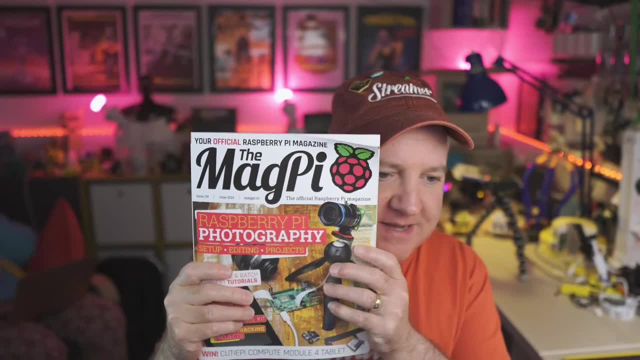 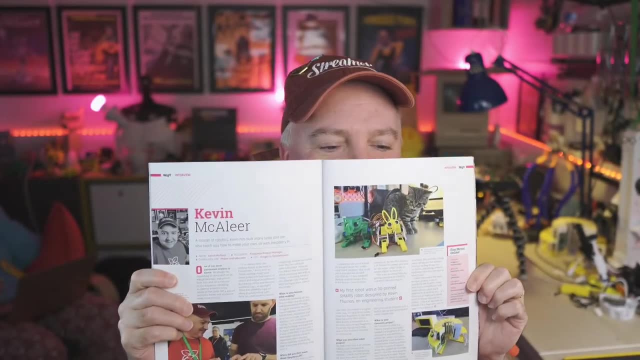 posted. this is where you can get the pictures of the pictures. so I'd like to take a look at the pictures. I've most recently interviewed by Magpie magazine for the Magpie magazine. so here we are. so on page 86. that's where they normally have the the interviews, there I am. 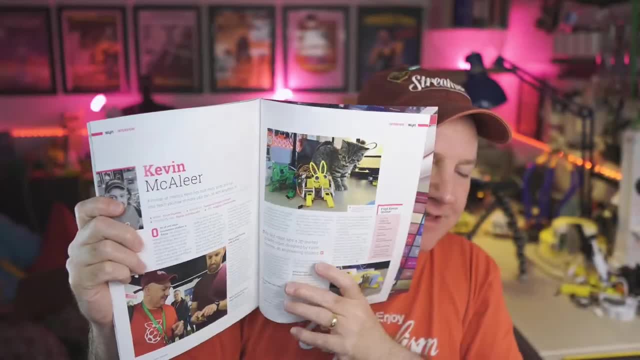 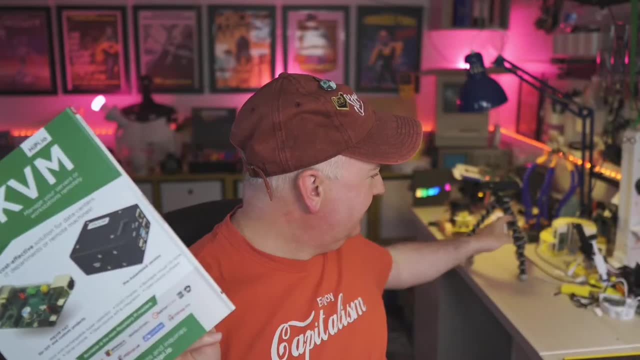 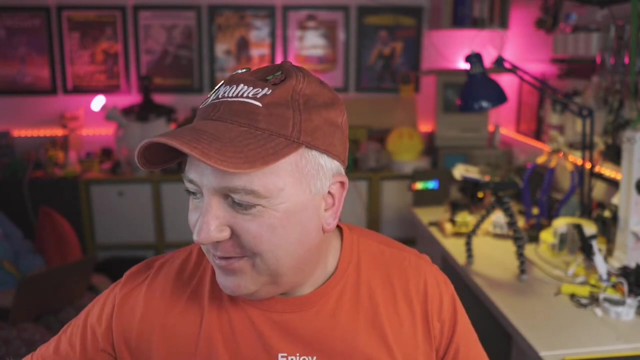 interviewed. there's my cat Tiger up there and you can see we've also got me speaking to even upton there, ebbing upton at the raspberry pi exhibit launch and we've also got which is the clustered pie. so i'm really, really honored to be in the magazine. um, hopefully that'll. 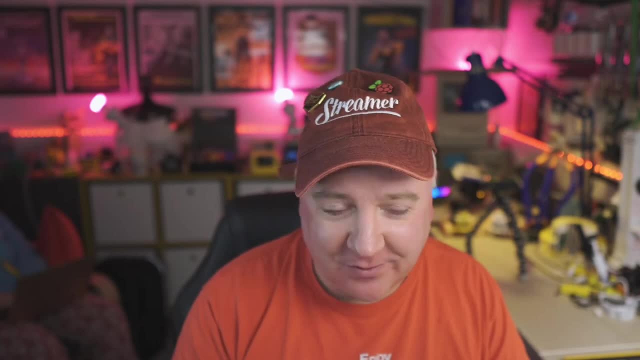 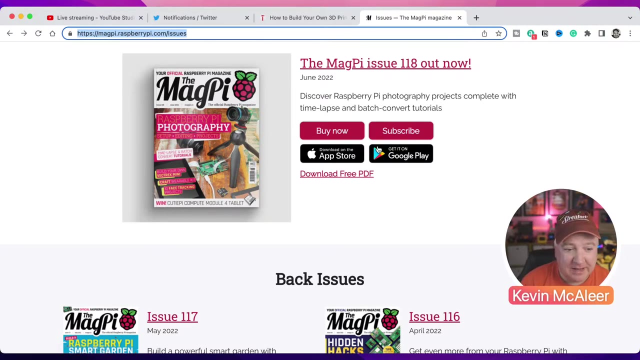 raise the profile and get me known by a couple more people. so if you want to get that copy, you can buy that from magpie. you go to magpieraspbypiecom. you can either buy it, subscribe to the magazine. if you subscribe you actually get a raspberry pie zero, and i believe they do actually. 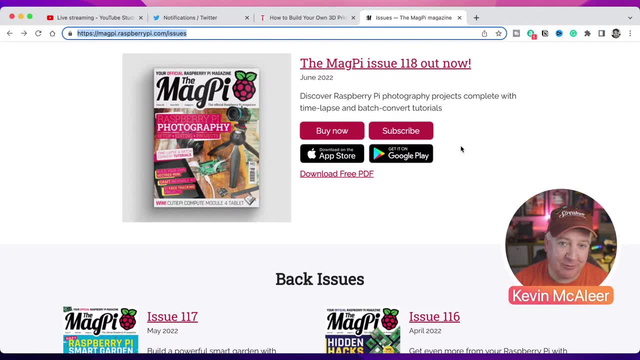 honor that, even though the supply is really short, you do get a raspberry pie zero if you subscribe to the magazine. so if you want to get yourself a raspberry pie zero, um, that's the way to do it. you can actually download the pdf for free as well, so if you click on that,